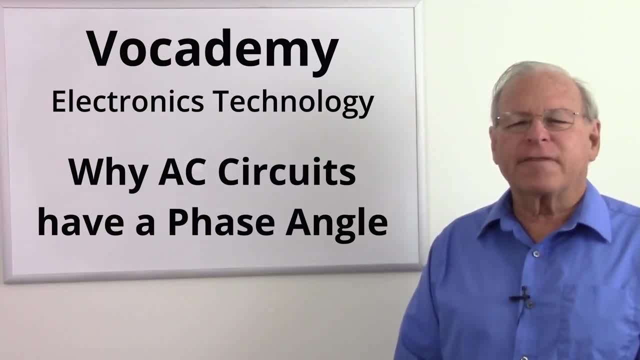 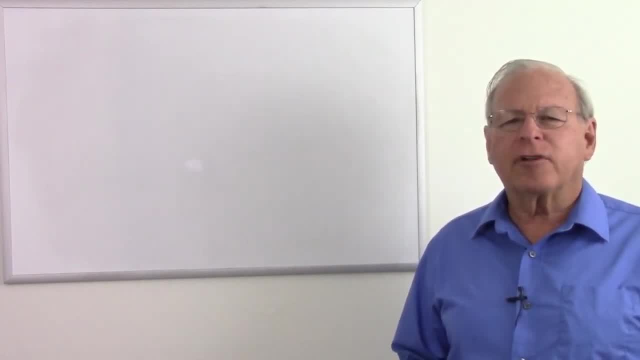 Today I'm going to explain why AC circuits have a phase angle. If you've worked with alternating current, you're familiar with phase angle and you've probably calculated it. but why does the circuit have a phase angle in the first place? Well, first of all, let's explain what we mean. 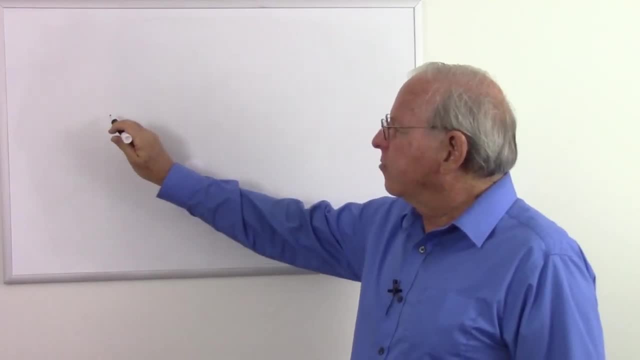 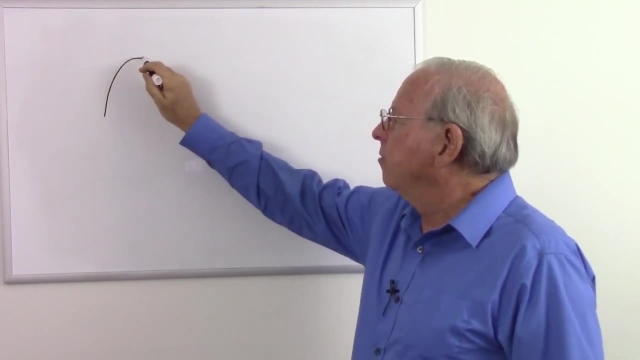 by phase angle. In alternating current we have a voltage that is constantly changing. Usually it follows a sine wave, so I'm going to draw my best sine wave here. So the voltage goes up to some certain voltage goes back down. Typically in alternating current it will cross zero volts. 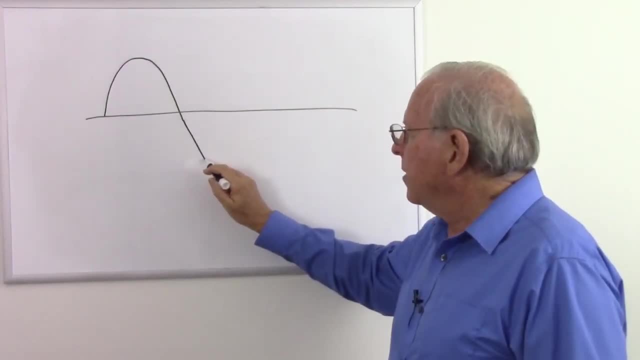 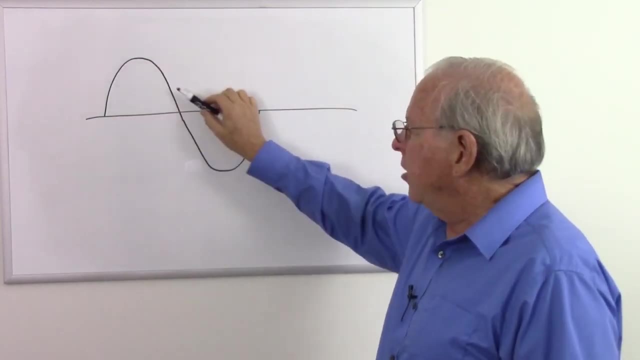 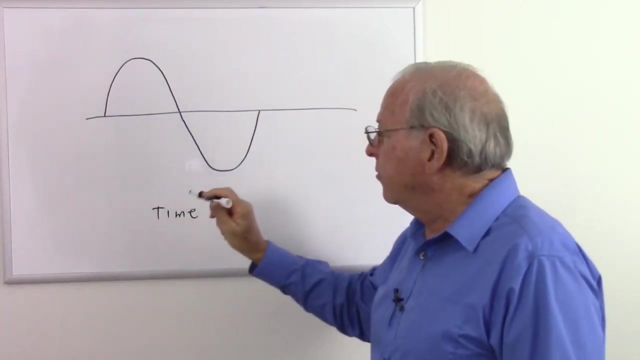 so I'll put a zero volt line right there. The voltage goes down to some negative voltage and then back up to zero, and then it repeats that over and over again. In North America this happens in 16.6 milliseconds. so this is our time axis over here and our voltage axis is the vertical axis. 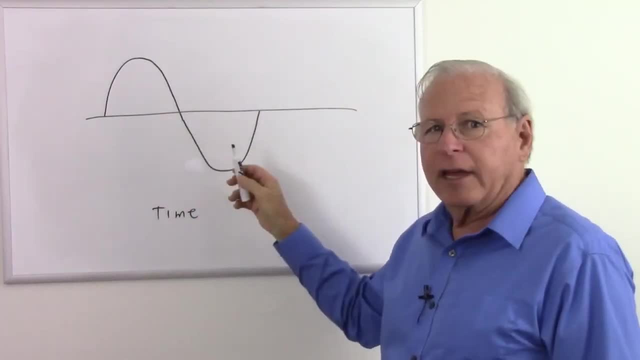 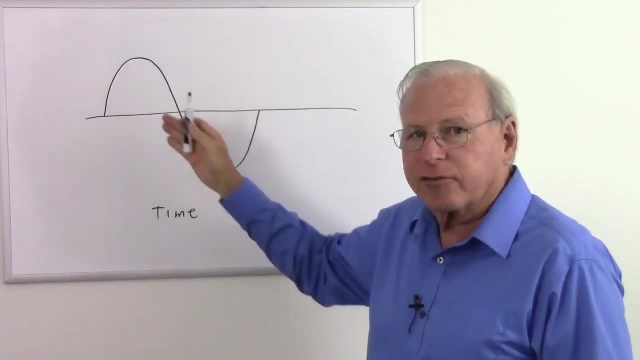 And in most of the world this happens in 20 milliseconds because most of the world uses a 50 hertz standard, where in North America we use a 60 hertz standard. so it's a little faster in North America, But there is our voltage constantly changing The. 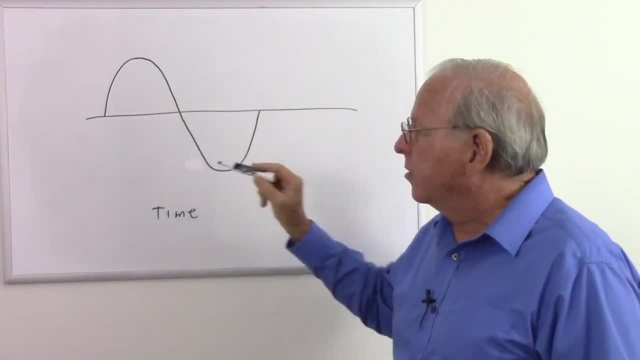 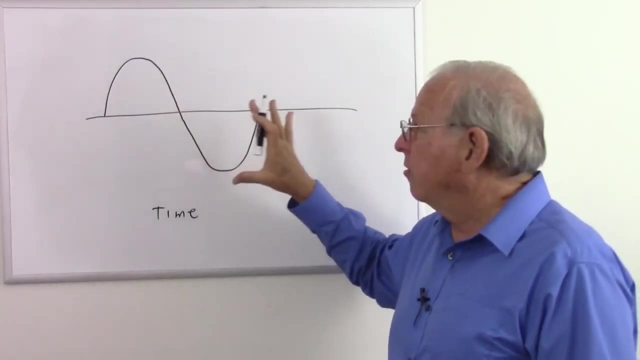 voltage goes up, voltage goes down, voltage goes back up over time, and this takes 16.6 or 20 milliseconds depending on where you are, but as far as the phase angle is concerned, that doesn't matter. Now, remember that we can measure a sine wave as a number of degrees. 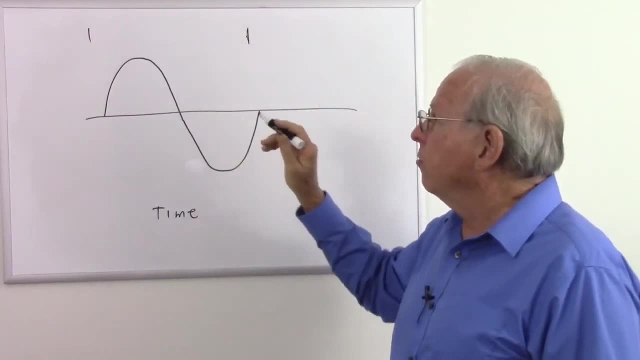 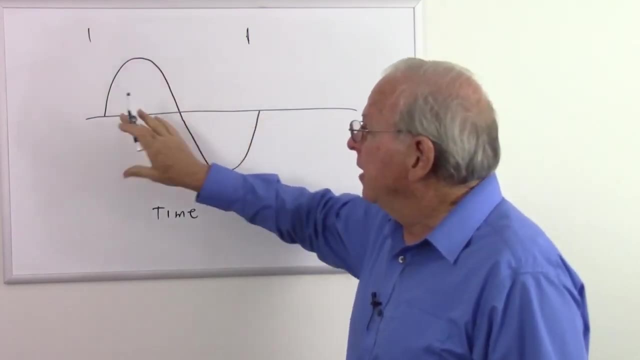 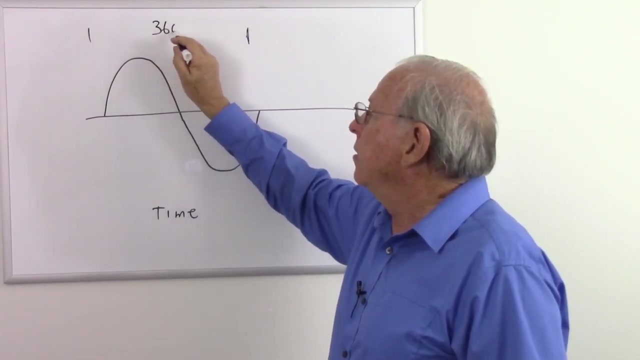 As a matter of fact, a sine wave is closely related to a circle, so we actually measure the time it takes to reach one complete cycle- not really the time, but just the parts of the wave- in degrees, just like a circle, and one cycle is 360 degrees. 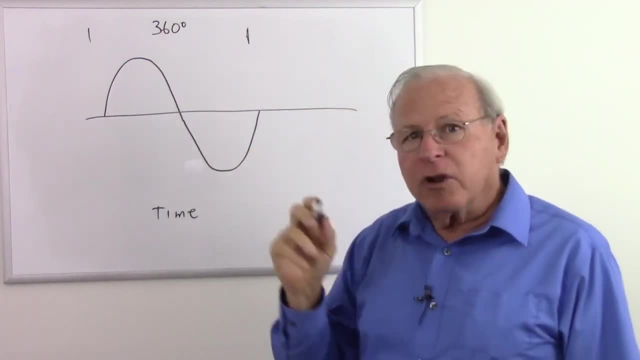 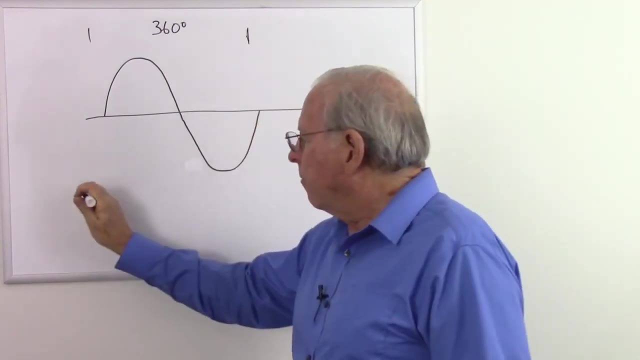 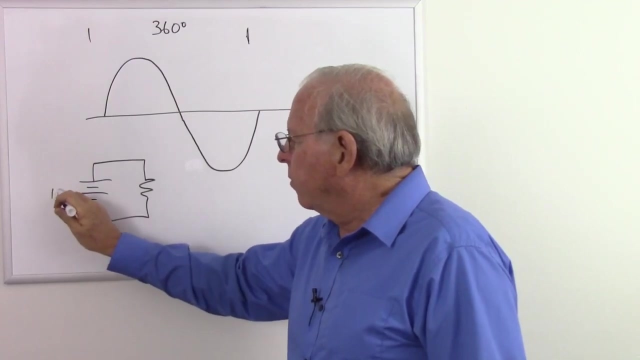 So what do we mean by a phase angle? What we're concerned about is the current through the circuit. so let's take a look at a DC circuit for just a moment. I'm just going to draw a battery here and we'll just put a resistor in there. very simple circuit. We'll make this 10 volts and 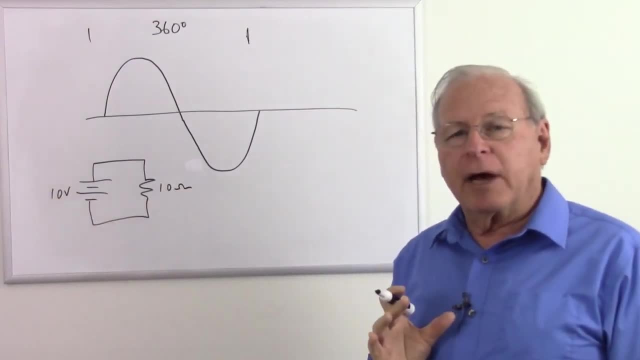 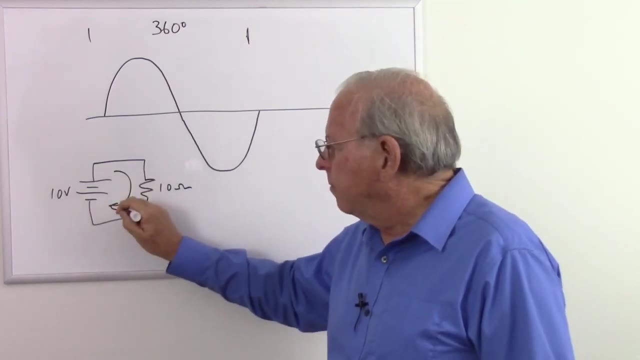 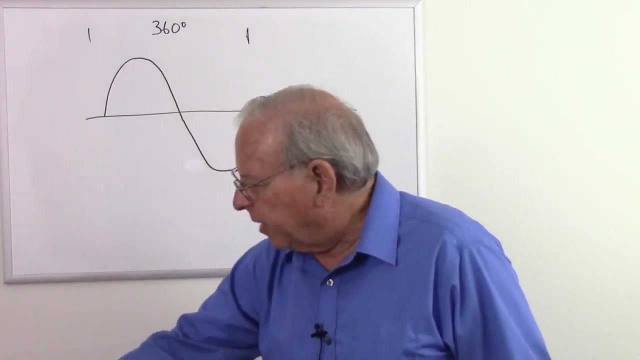 make this 10 ohms. So what are we concerned about? We're concerned about the current through the circuit: 10 ohms divide that into 10 volts. we know that there is one amp of current flowing in the circuit. Okay, in an AC circuit we have the same thing. I'm going to draw a simple AC circuit. 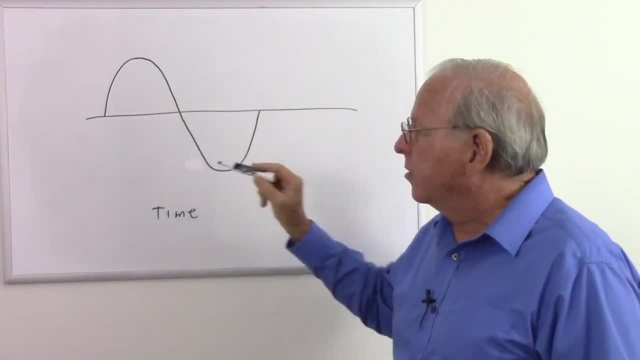 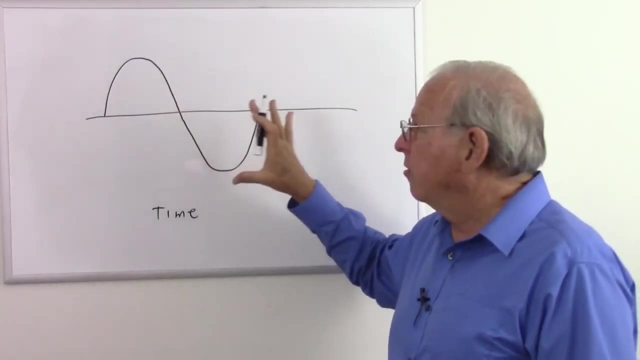 voltage goes up, voltage goes down, voltage goes back up over time, and this takes 16.6 or 20 milliseconds depending on where you are, but as far as the phase angle is concerned, that doesn't matter. Now, remember that we can measure a sine wave as a number of degrees. 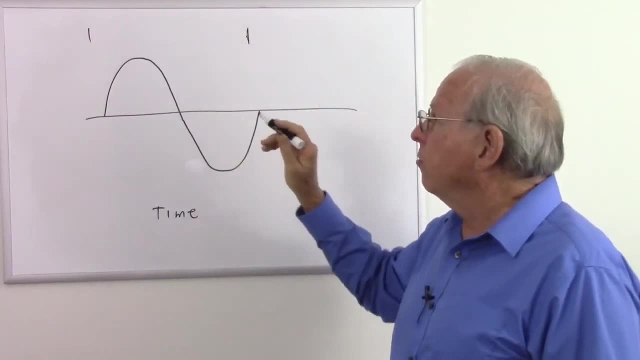 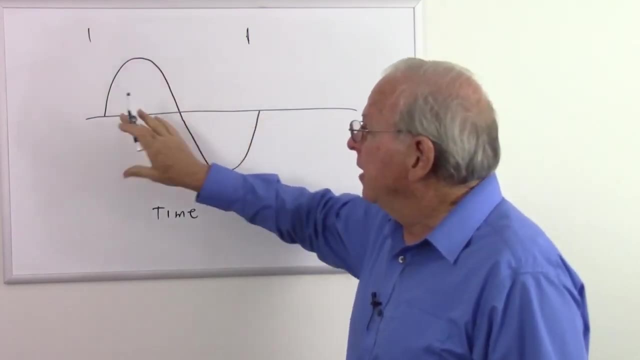 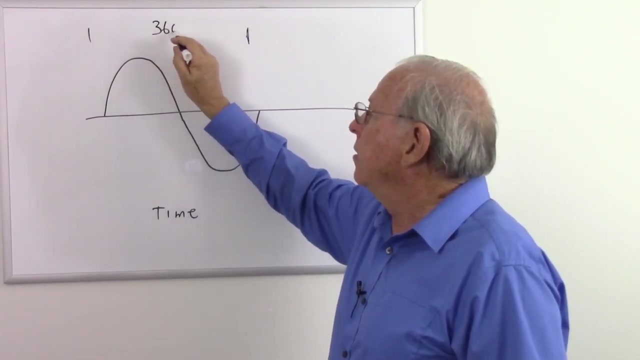 As a matter of fact, a sine wave is closely related to a circle, so we actually measure the time it takes to reach one complete cycle- not really the time, but just the parts of the wave- in degrees, just like a circle, and one cycle is 360 degrees. 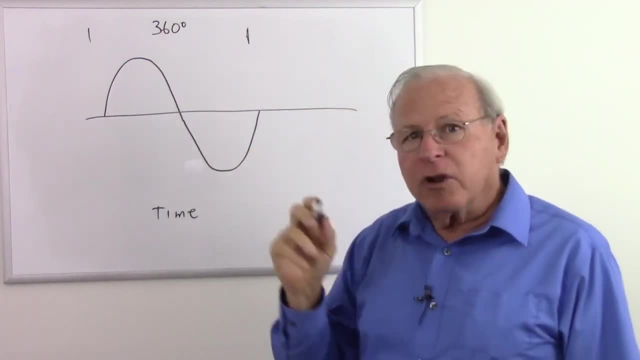 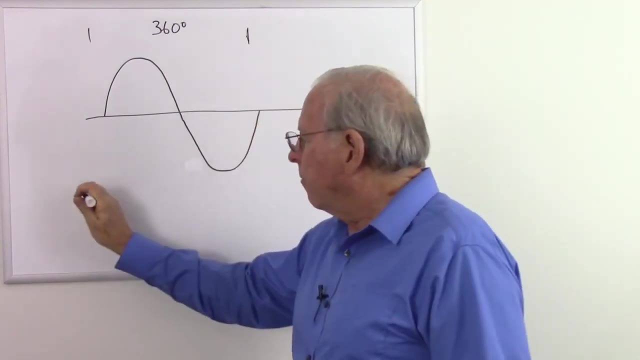 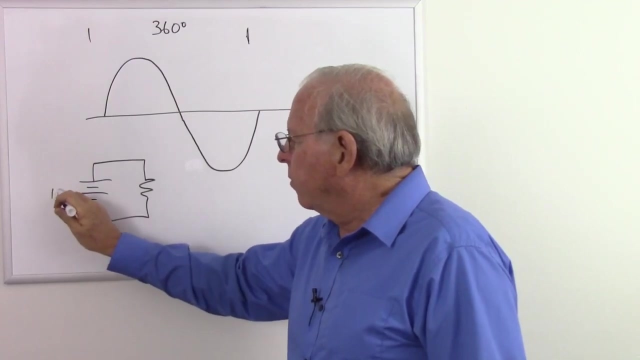 So what do we mean by a phase angle? What we're concerned about is the current through the circuit. so let's take a look at a DC circuit for just a moment. I'm just going to draw a battery here and we'll just put a resistor in there. very simple circuit. We'll make this 10 volts and 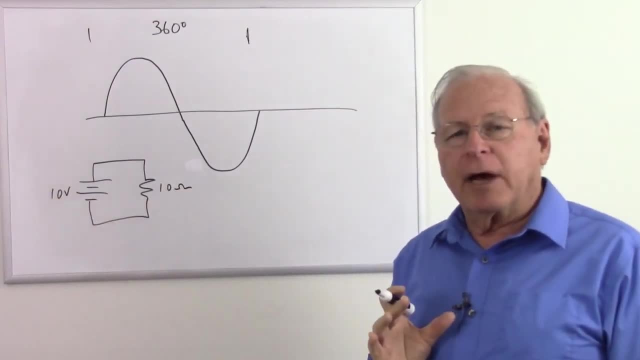 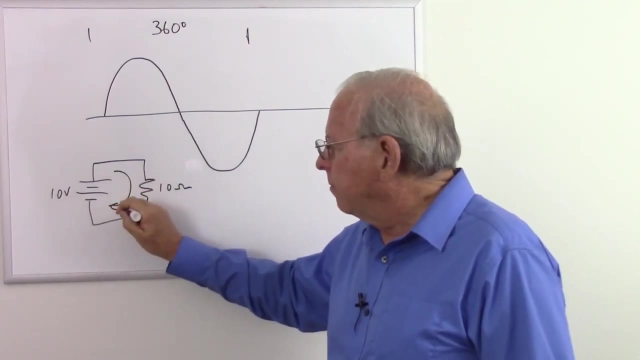 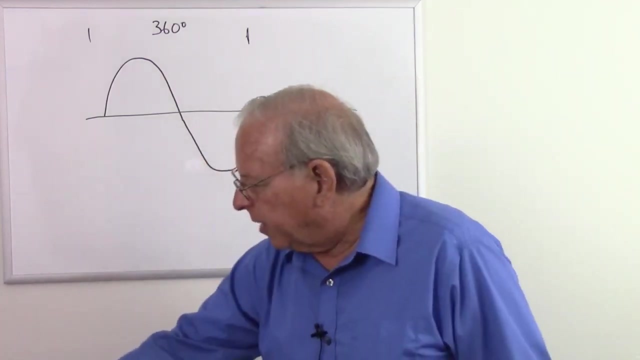 make this 10 ohms. So what are we concerned about? We're concerned about the current through the circuit: 10 ohms. divide that into 10 volts. we know that there is one amp of current flowing in the circuit. Okay, in an AC circuit we have the same thing. I'm going to draw a simple AC. 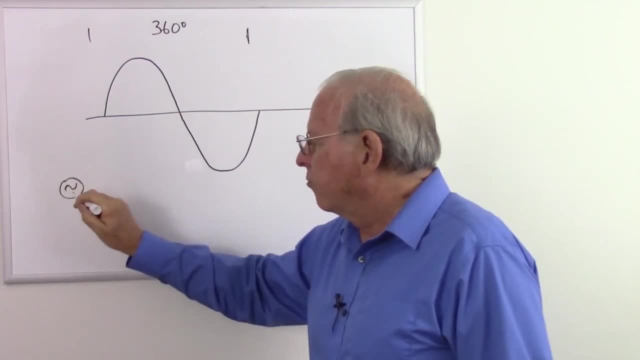 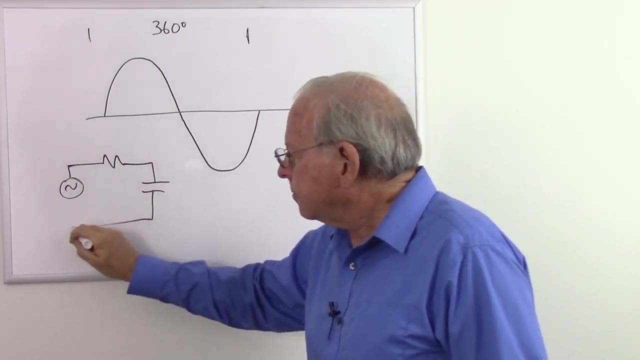 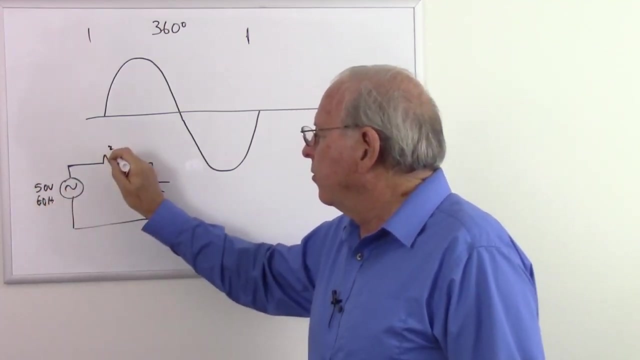 circuit with a capacitor. There's our alternating current source. We'll see this bigger a little bit later, but right now we'll just draw it here. There's our resistor, there's our capacitor and let's say, this is 50 volts at 60 hertz and we'll make this 30 ohms and 100 microfarad. It's. 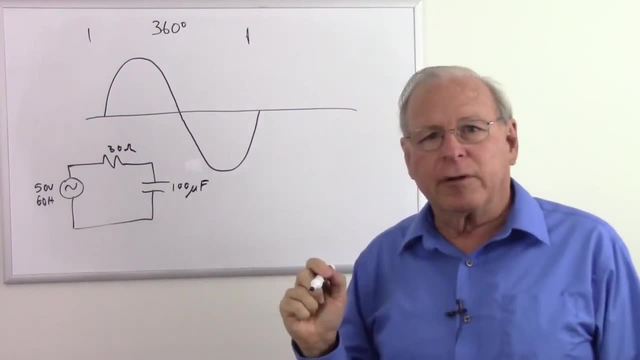 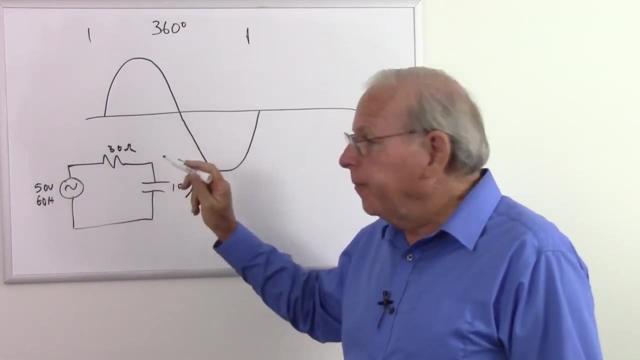 not going to do much calculation right now, but we'll use those numbers in a moment. So we want to know what the current is through this circuit. I'm not going to go through all the calculations just now, but one thing we do know: we're going to have a certain amount of 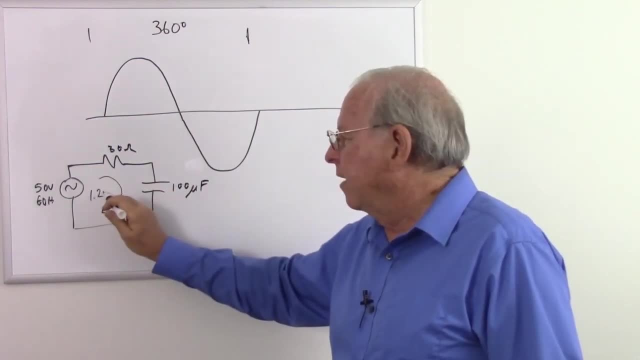 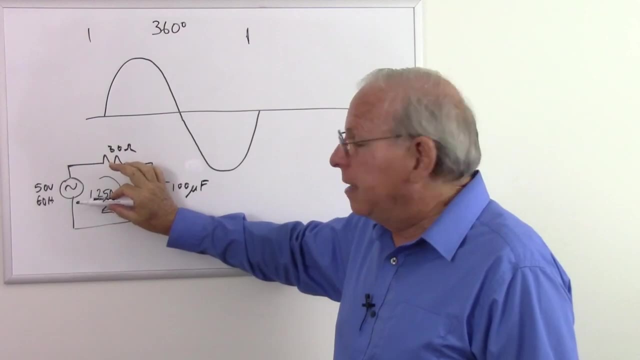 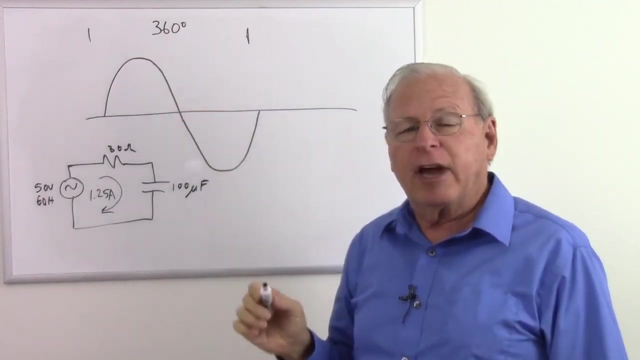 current, And I know it's going to be 1.25 amps. but we also know that the current is not going to be peaking at the same time as the voltage. In other words, when the voltage reaches its highest point, the current's going to reach its highest point at some other time. And because this is a capacitor, 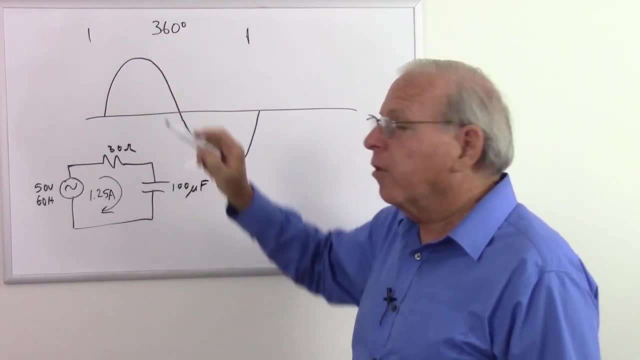 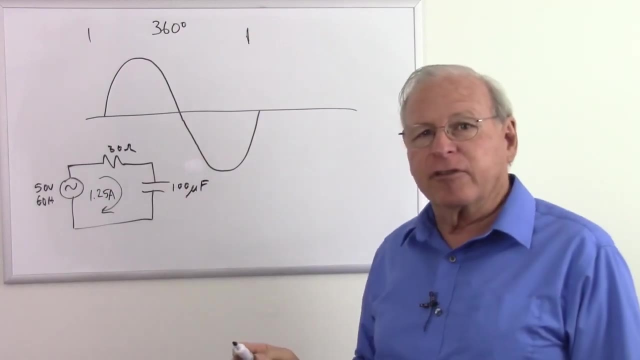 that means the current's going to reach its highest point sometime before the voltage does. If this was an inductor, it would happen sometime after the voltage. but we're not concerned about. we're just going to look at capacitance in this particular circuit. Remember that. 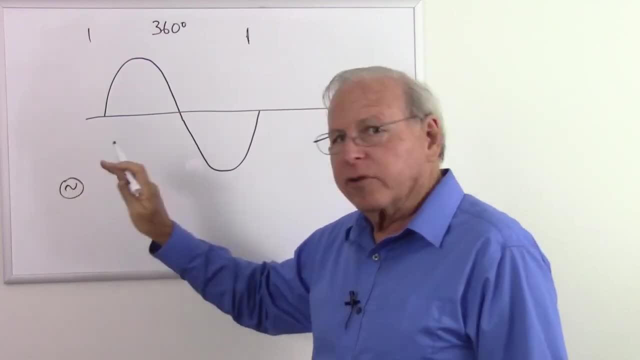 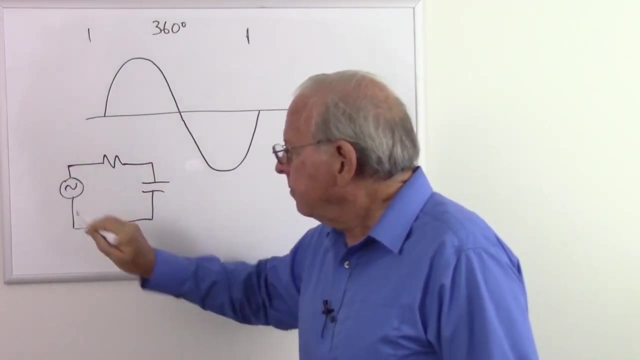 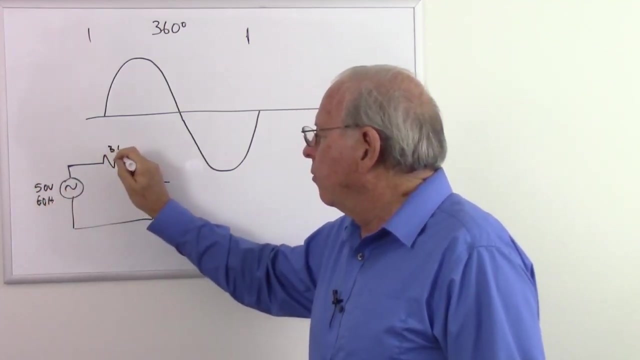 with a capacitor. There's our alternating current source. We'll see this bigger a little bit later, but right now we'll just draw it here. There's our resistor, there's our capacitor and let's say, this is 50 volts at 60 hertz and we'll make this 30 ohms and 100 microfarad. It's. 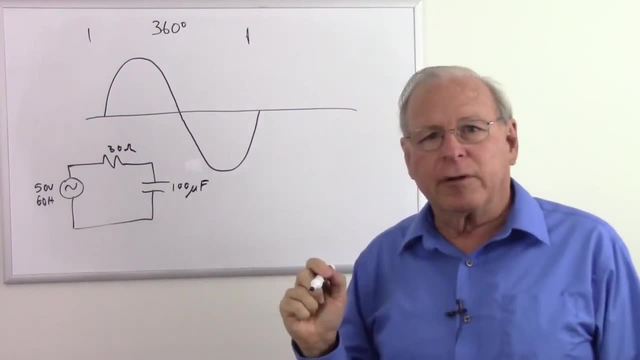 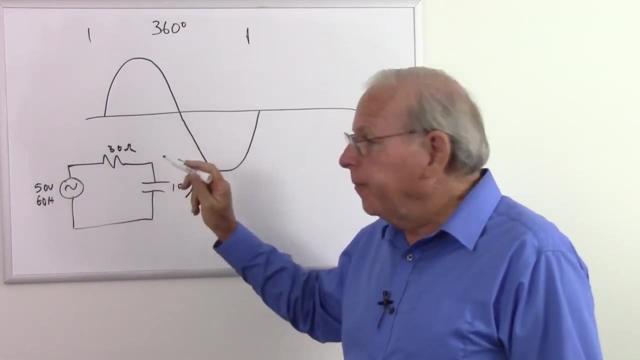 not going to do much calculation right now, but we'll use those numbers in a moment. So we want to know what the current is through this circuit. I'm not going to go through all the calculations just now, but one thing we do know: we're going to have a certain amount of 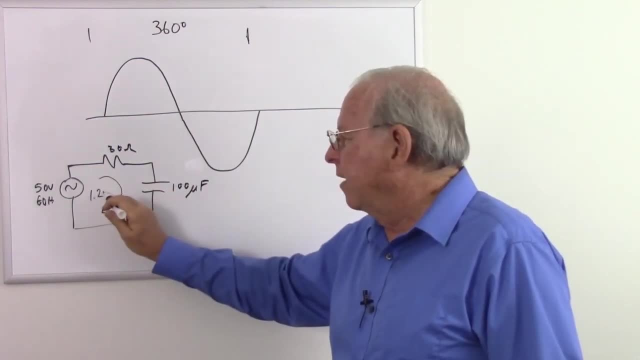 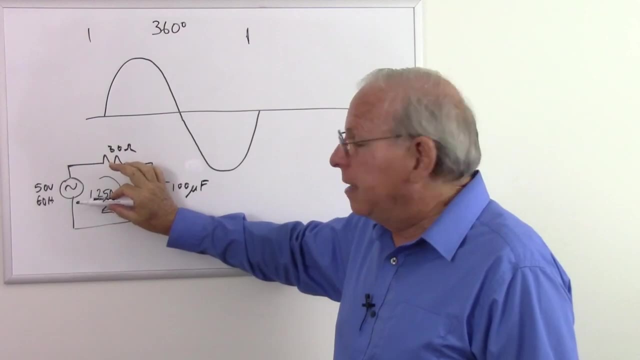 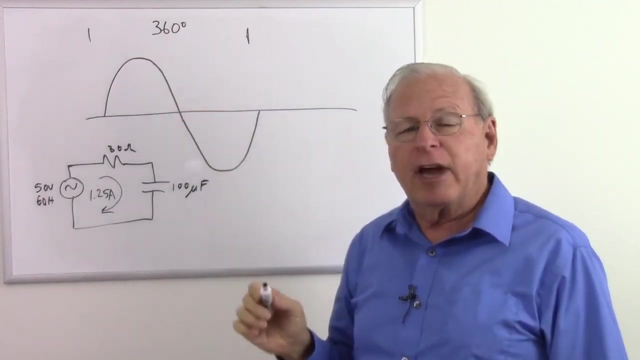 current, And I know it's going to be 1.25 amps. but we also know that the current is not going to be peaking at the same time as the voltage. In other words, when the voltage reaches its highest point, the current's going to reach its highest point at some other time. And because this is a capacitor, 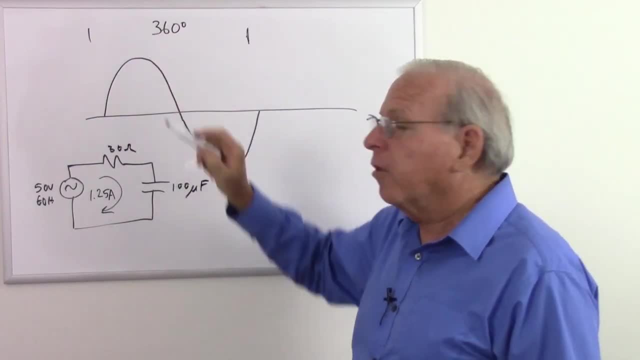 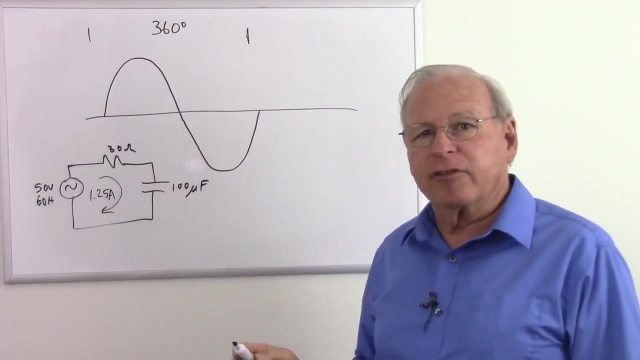 that means the current's going to reach its highest point sometime before the voltage does. If this was an inductor, it would happen sometime after the voltage, but we're not concerned about that. we're just going to look at capacitance in this particular circuit. Remember that an 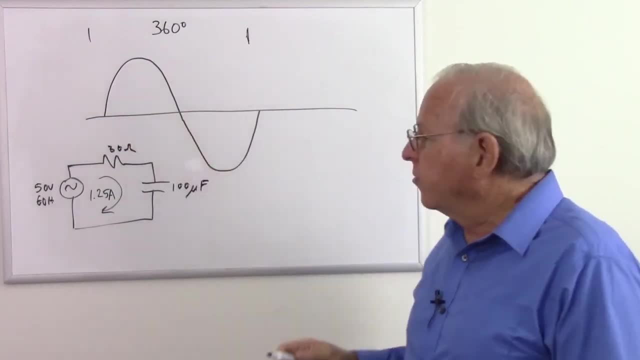 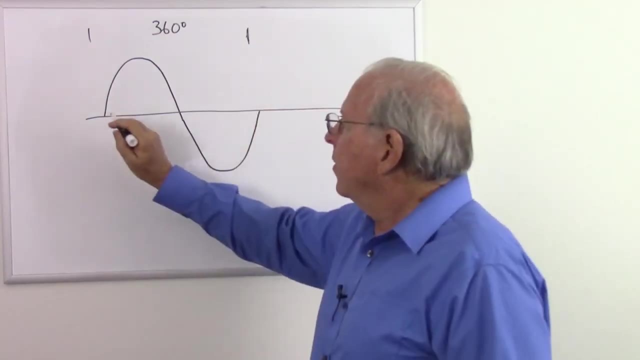 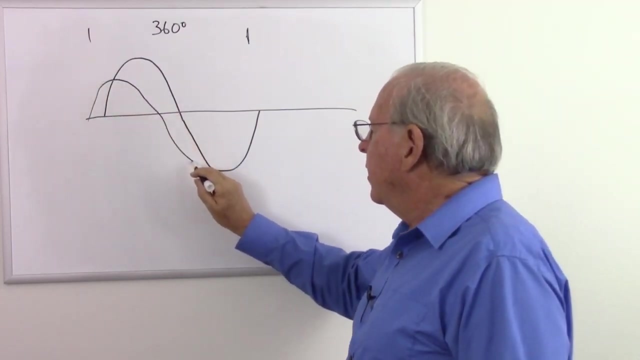 inductor would be later rather than earlier. So let's take a look at about where the current would be here. So we know the current's going to peak earlier. so here comes the current. It's going to peak earlier and it's going to follow a path something like that, And so 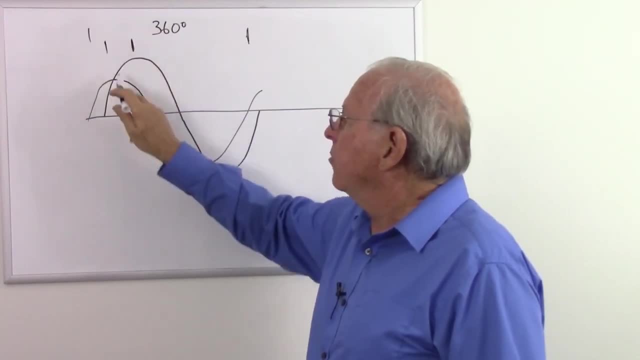 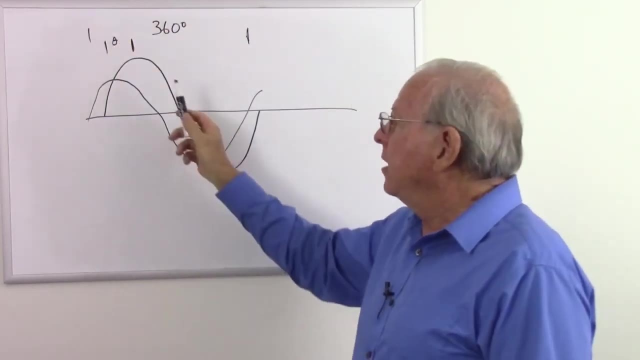 here's the moment that the voltage peaks and the current peaks some earlier time, And we measure that in a certain number of degrees, And that's what we're interested in is how many degrees before the voltage does the current peak, And that's called. 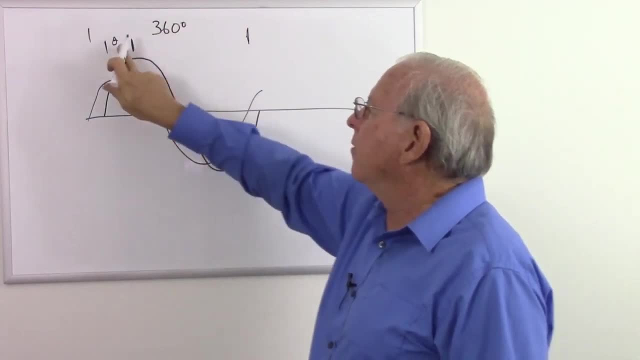 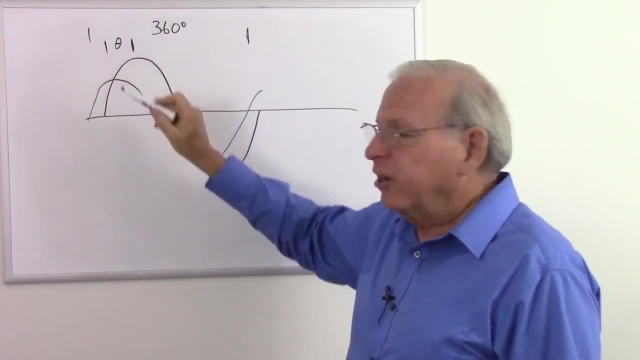 the phase angle which I've represented with the Greek letter theta. there, Remember the crummy little theta. Let's draw that again. There we go. There's a nice little Greek letter, theta. So the current peaks sometime before the voltage does And the current hits zero sometime before. 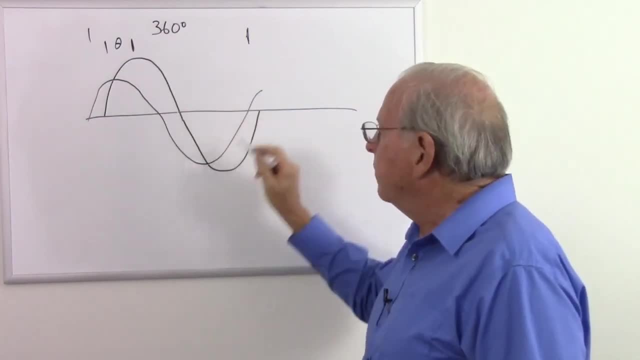 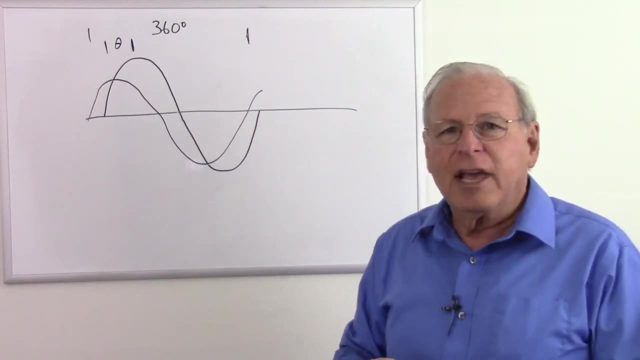 the voltage does, And we measure that difference in degrees and it's called the phase angle. So everywhere along these curves, everything happens with the current some number of degrees before it happens with the voltage. And that's what the phase angle of the circuit is. It's the 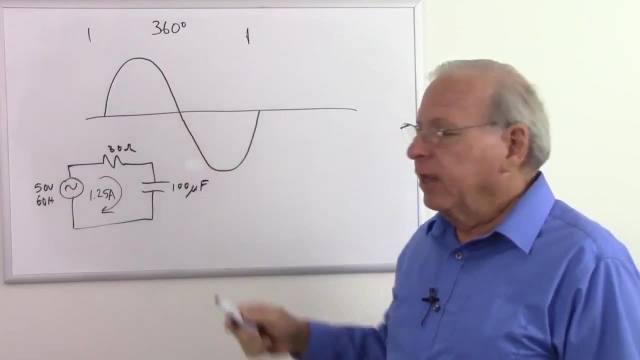 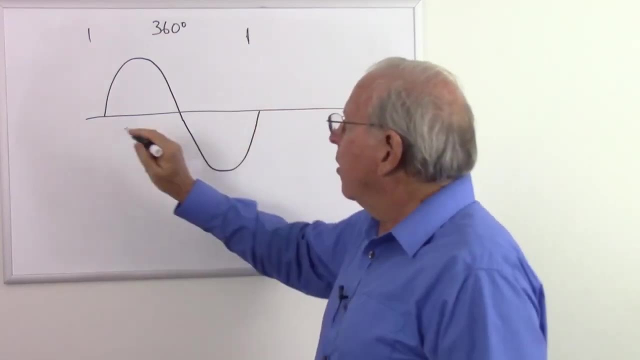 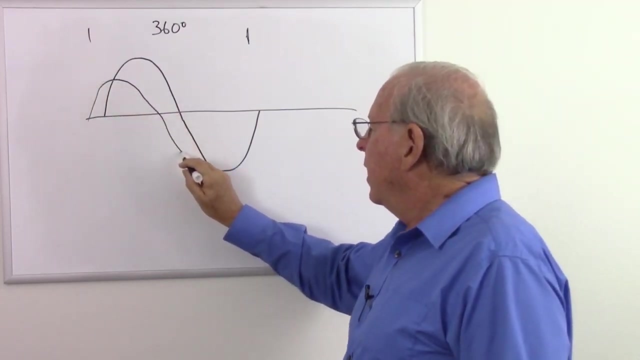 an inductor would be later rather than earlier. So let's take a look at about where the current would be here. So we know the current's going to peak earlier. so here comes the current. It's going to peak earlier and it's going to follow a path something like that. 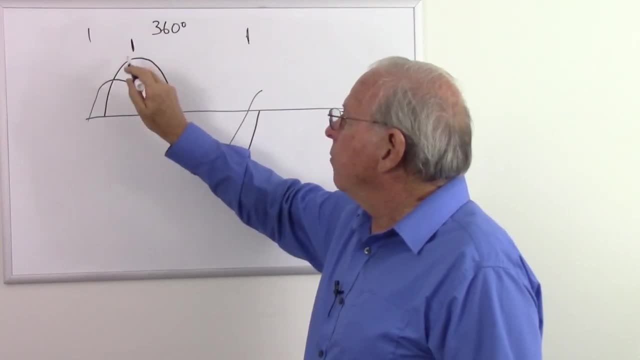 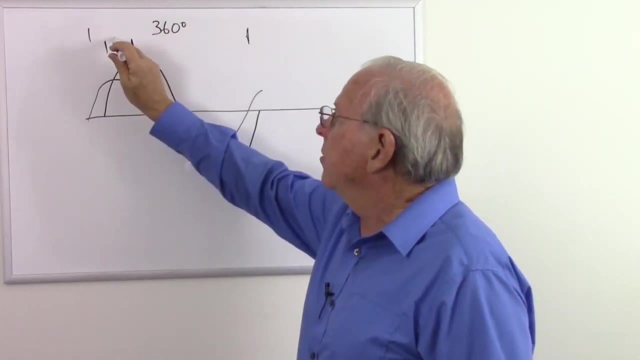 And so here's the moment that the voltage peaks and the current peaks some earlier time. And we measure that in a certain number of degrees. And that's what we're interested in is how many degrees before the voltage does the current peak, And that's called. 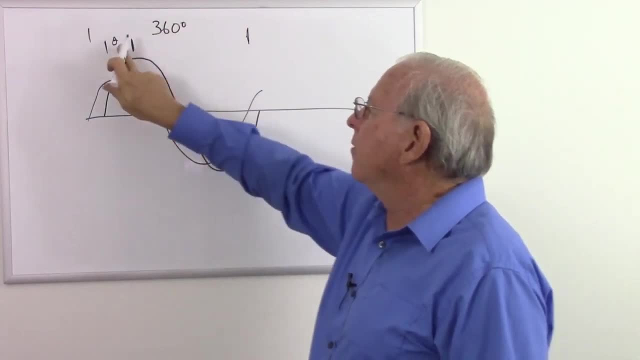 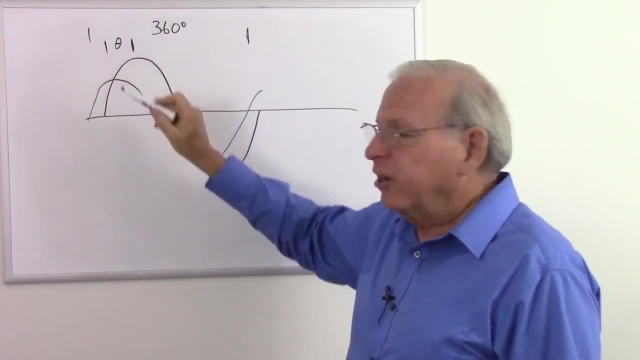 the phase angle which I've represented with the Greek letter theta. there, Remember the crummy little theta. Let's draw that again. There we go. There's a nice little Greek letter, theta. So the current peaks sometime before the voltage does And the current hits zero sometime before. 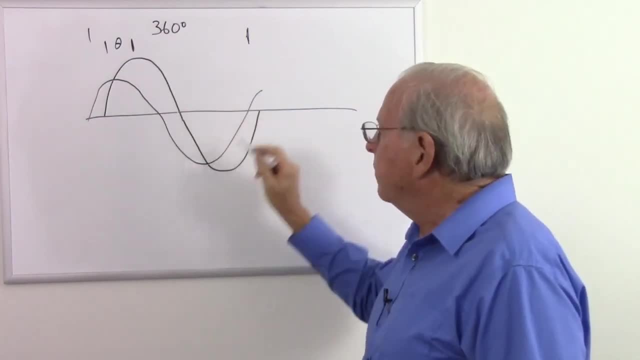 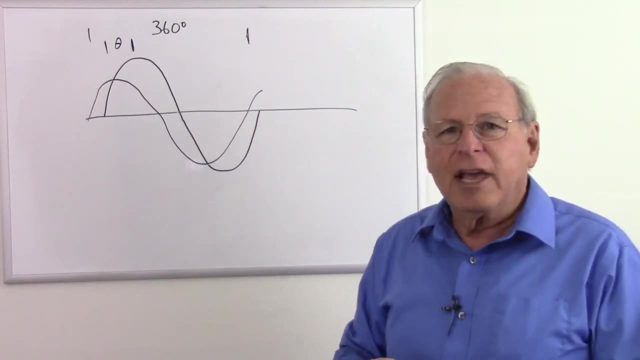 the voltage does, And we measure that difference in degrees and it's called the phase angle. So everywhere along these curves, everything happens with the current some number of degrees before it happens with the voltage. And that's what the phase angle of the circuit is. It's the 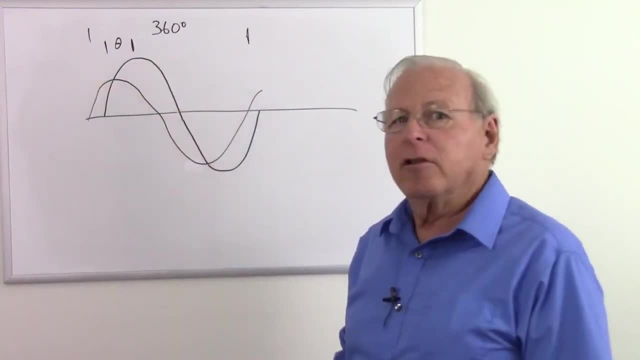 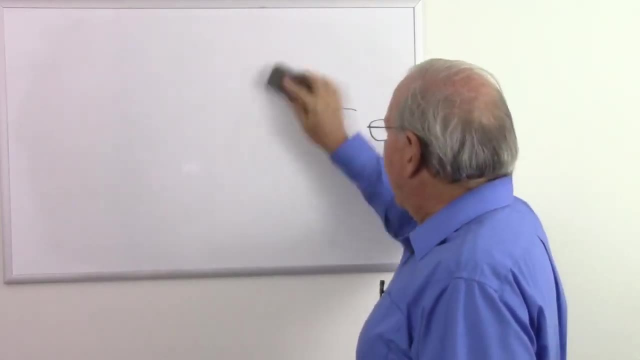 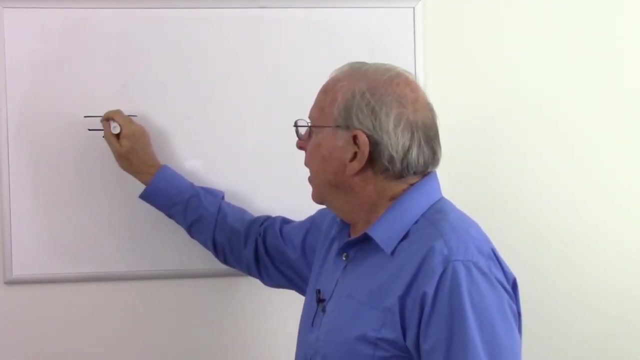 lead or lag angle of the current compared to the voltage. So why does this happen? Well, to explain it, let's first look at how a capacitor acts when it charges and discharges with direct current. So I'm going to draw a battery here and a resistor. 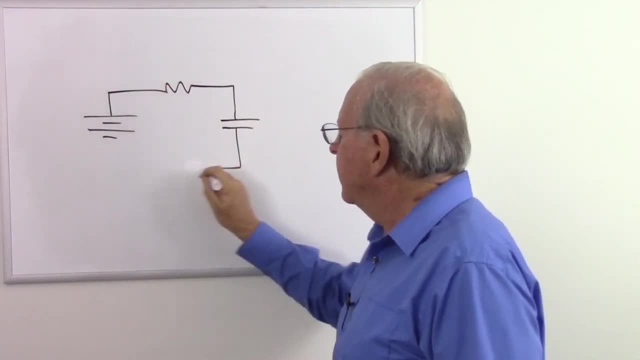 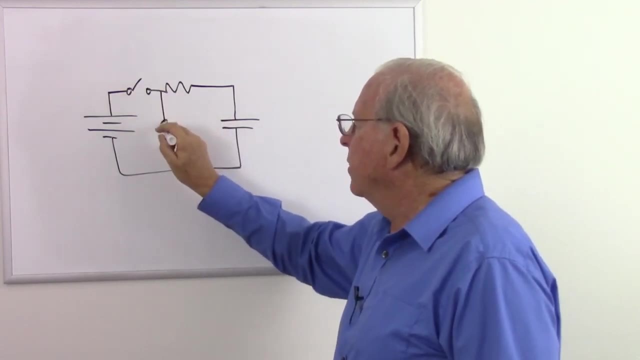 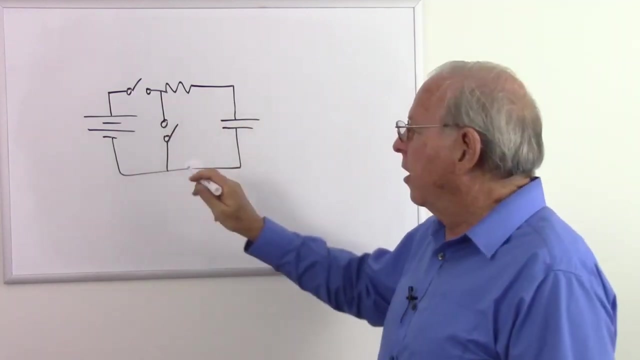 And put our capacitor here And we're going to put a little switch here to help us do with what we need to with the circuit And put another switch here. This switch is here just to make sure that capacitor is discharged when we start everything off. Let's make this one volt. 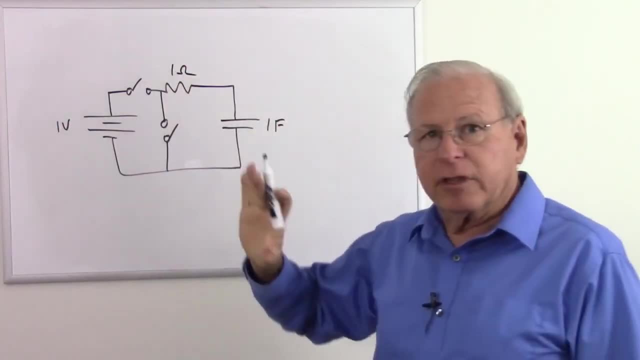 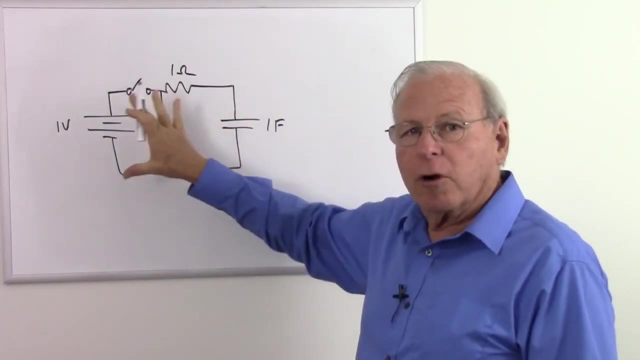 one ohm and one farad. I use those numbers in this demonstration because not only are they easy to deal with, but they show something important about the circuit. So let's start with the capacitors. But if you want to know more about this particular circuit, you can watch my video. 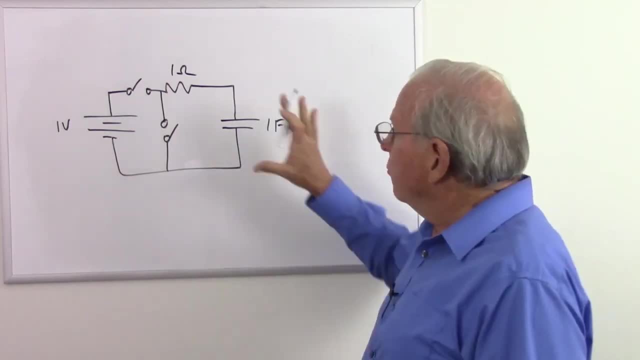 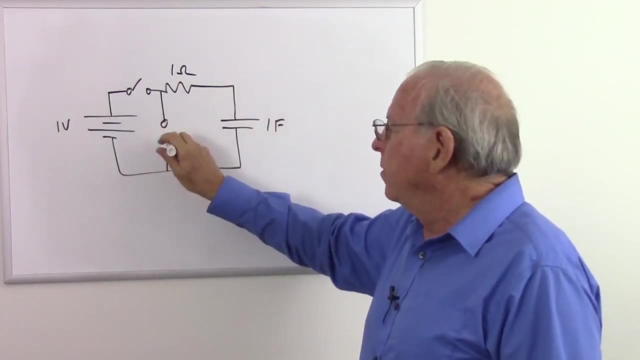 and read the textbook material that I have linked in the video below. We're just going to go through it real quickly right now. So what I'm going to do is close this switch, make sure that capacitor is completely discharged. Now I'm going to open the switch and I'm going to close this one. 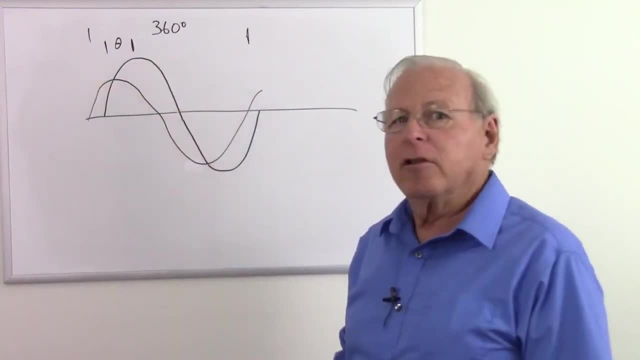 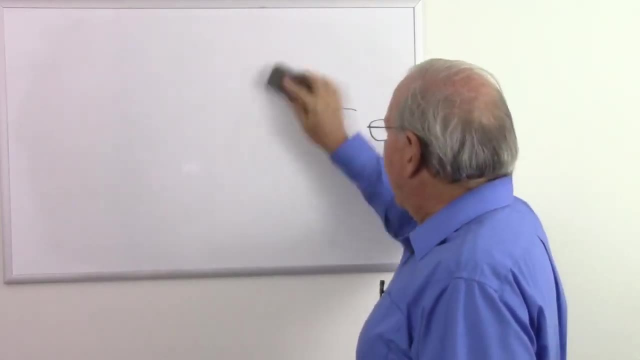 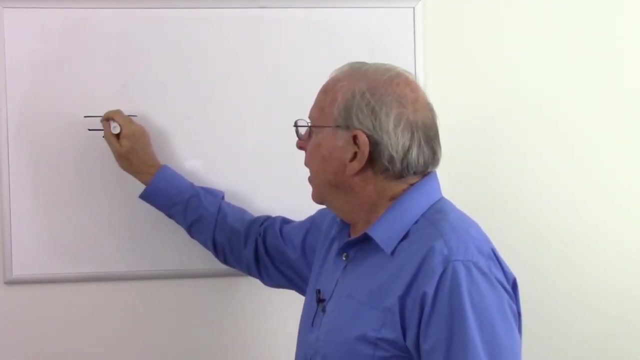 lead or lag angle of the current compared to the voltage. So why does this happen? Well, to explain it, let's first look at how a capacitor acts when it charges and discharges with direct current. So I'm going to draw a battery here and a resistor. 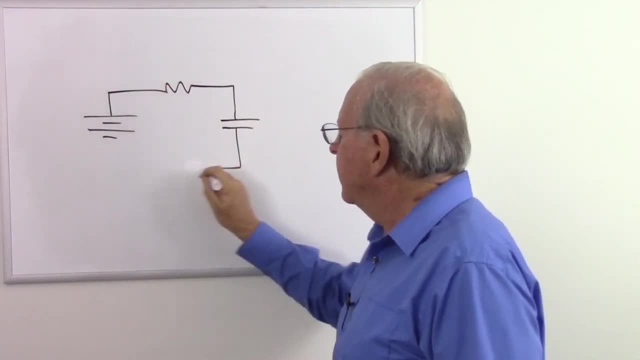 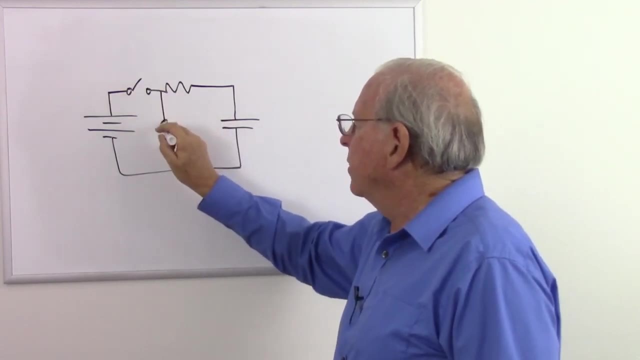 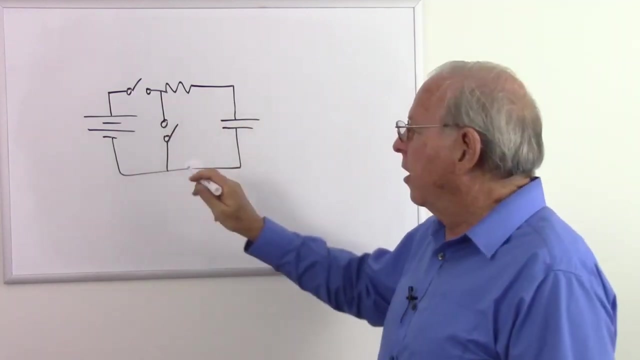 And put our capacitor here And we're going to put a little switch here to help us do with what we need to with the circuit And put another switch here. This switch is here just to make sure that capacitor is discharged when we start everything off. Let's make this one volt. 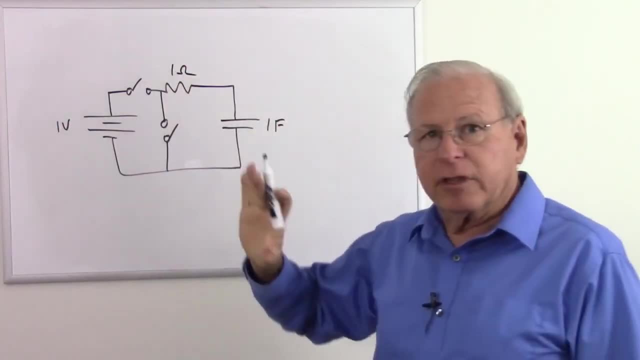 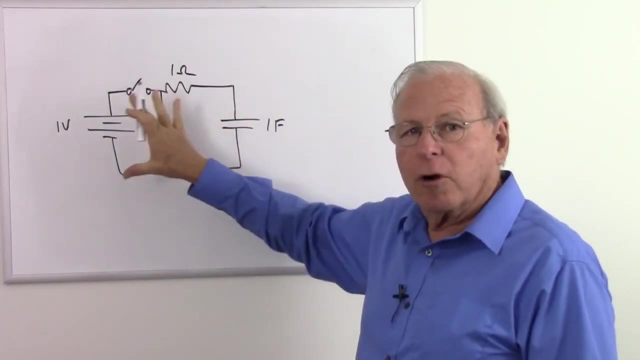 one ohm and one farad. I use those numbers in this demonstration because not only are they easy to deal with, but they show something important about the circuit. So let's start with the capacitors. But if you want to know more about this particular circuit, you can watch my video. 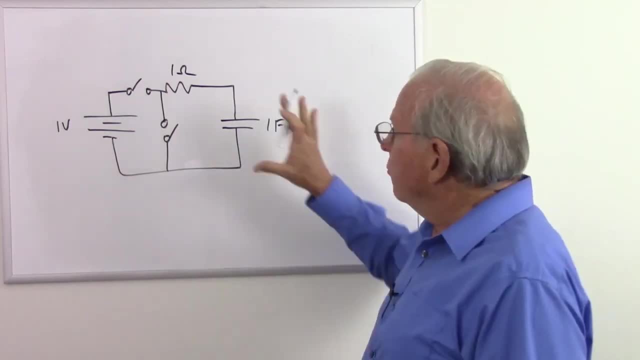 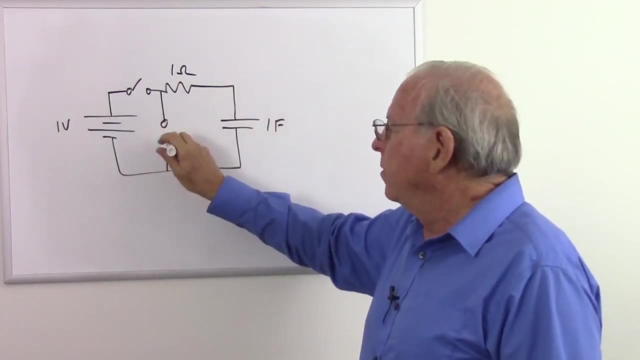 and read the textbook material that I have linked in the video below. We're just going to go through it real quickly right now. So what I'm going to do is close this switch, make sure that capacitor is completely discharged. Now I'm going to open the switch and I'm going to close this one. 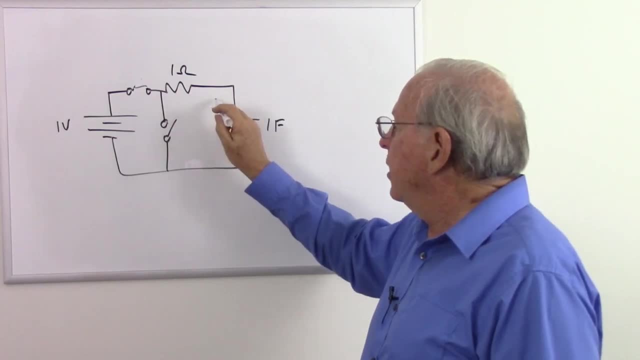 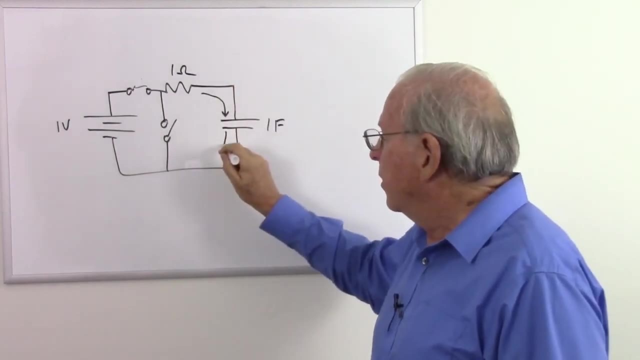 So what's going to happen at that moment? We're going to have current surge into this capacitor and it's going to spread out on this top plate And as that piles on there, it's going to drive current Out the bottom. Now, of course, we know it's electrons going the opposite direction and 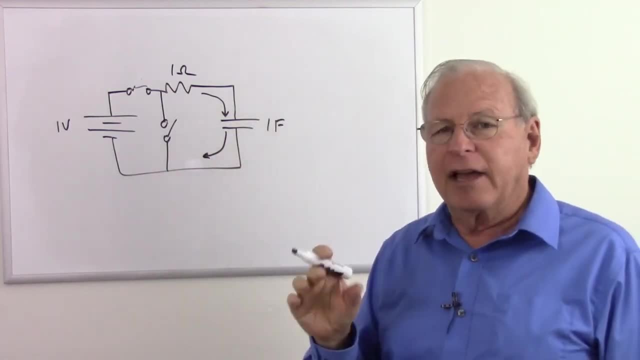 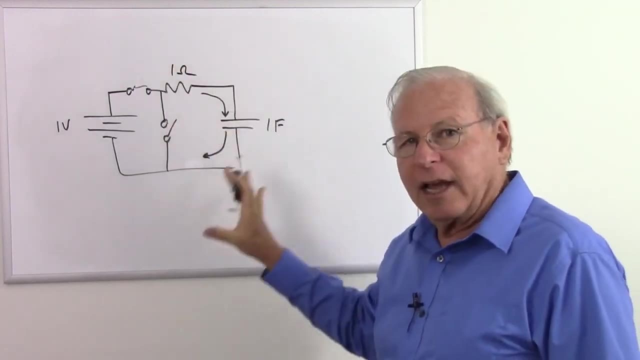 electrons on this plate are repelling them off the other plate. But in this class, as in most of the electronics industry and academia, we use conventional current because it's easier to analyze circuits with current going from a high voltage to a low voltage rather than the other. 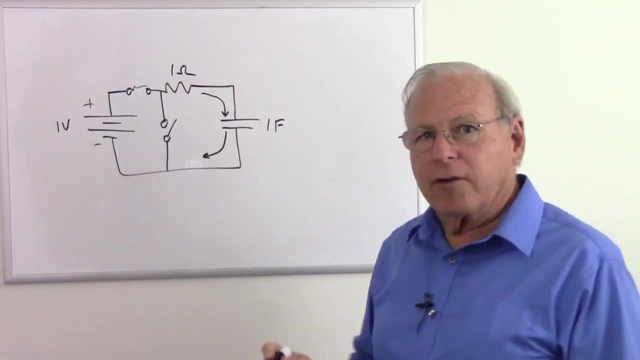 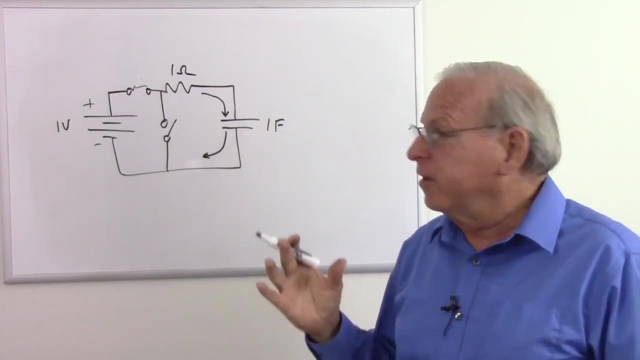 way around. Okay, so current goes in, current comes out. We see the current going in. We see it coming out. Looks like it's going right through. It's not the same current coming out that went in, but we can't tell the difference. So what does that capacitor look like? It looks like a short. 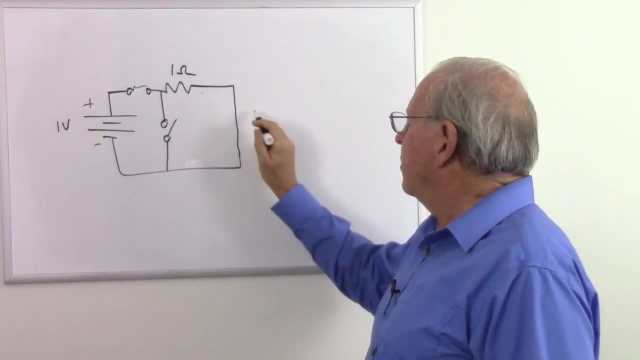 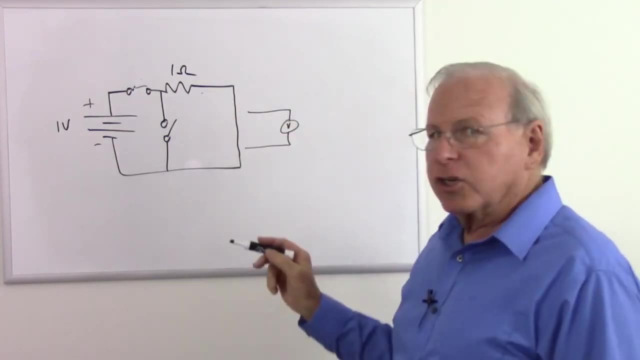 circuit at that moment in time, And if we put a voltmeter across here, what are we going to see? Well, first of all, a short circuit. no matter how much current is going through it, there's no resistance to cause a backup of pressure where the current goes in. 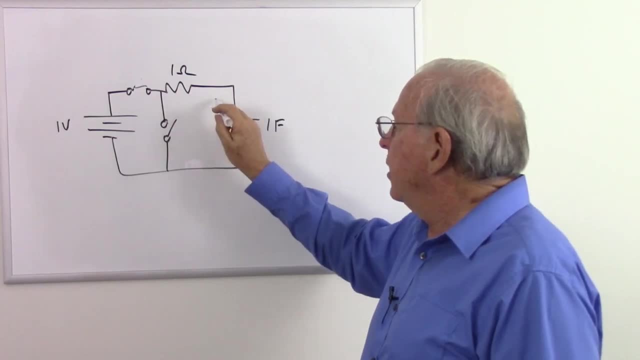 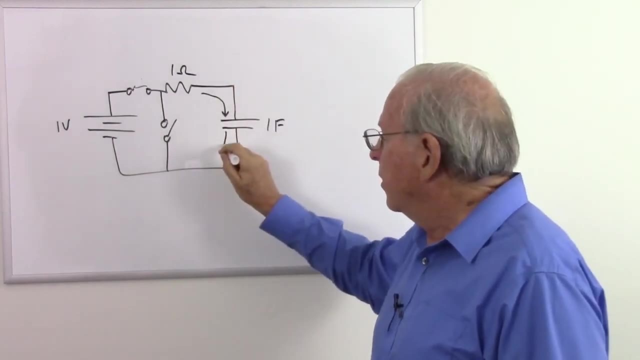 So what's going to happen at that moment? We're going to have current surge into this capacitor and it's going to spread out on this top plate And as that piles on there, it's going to drive current Out the bottom. Now, of course, we know it's electrons going the opposite direction and 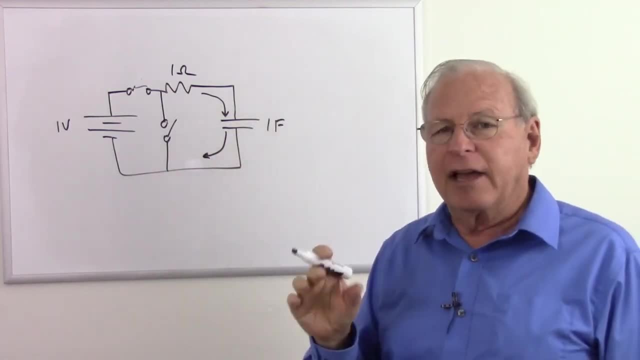 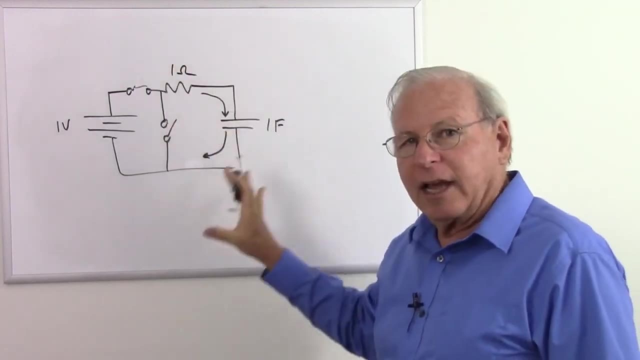 electrons on this plate are repelling them off the other plate. But in this class, as in most of the electronics industry and academia, we use conventional current because it's easier to analyze circuits with current going from a high voltage to a low voltage rather than the other. 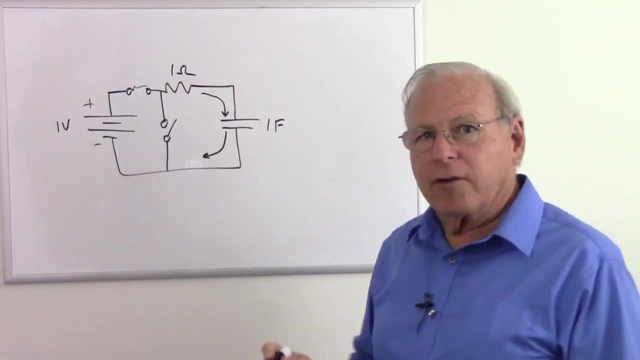 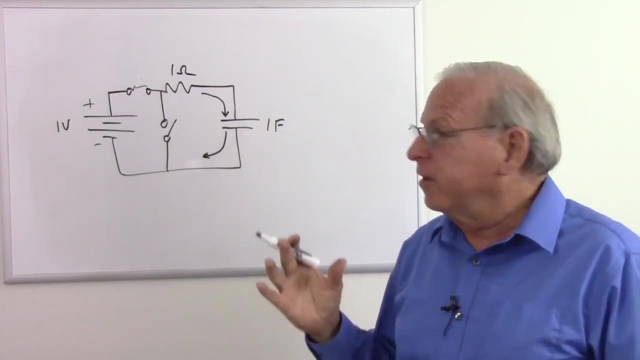 way around. Okay, so current goes in, current comes out. We see the current going in. We see it coming out. Looks like it's going right through. It's not the same current coming out that went in, but we can't tell the difference. So what does that capacitor look like? It looks like a short. 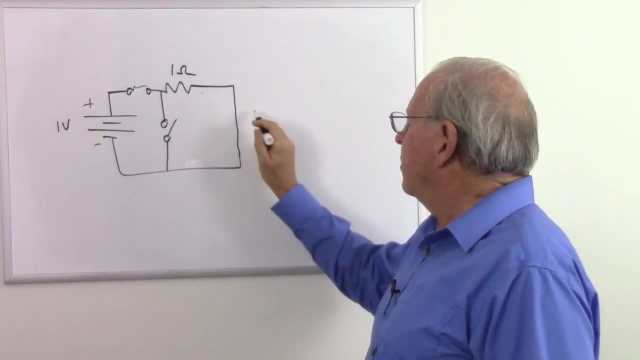 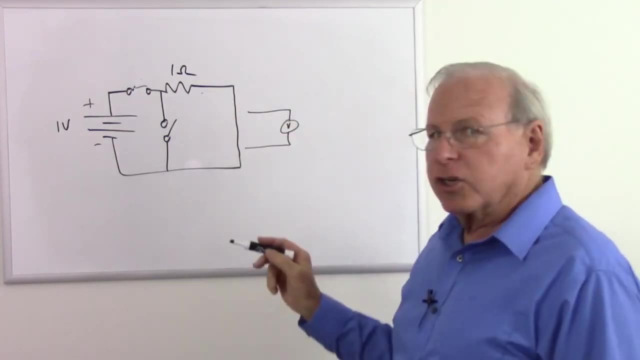 circuit at that moment in time, And if we put a voltmeter across here, what are we going to see? Well, first of all, a short circuit. no matter how much current is going through it, there's no resistance to cause a backup of pressure where the current goes in. 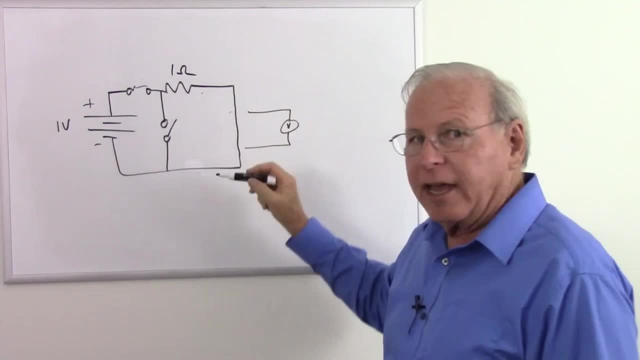 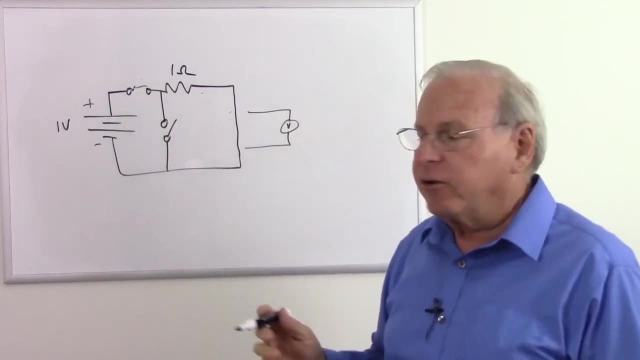 And so there's not going to be any difference in voltage from one side to the other. And what does the voltmeter tell us? It tells us the difference in voltage. One voltage is meaningless without another voltage to compare it to, and that's what a. 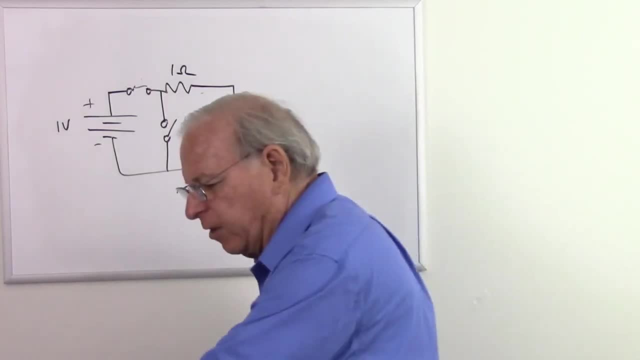 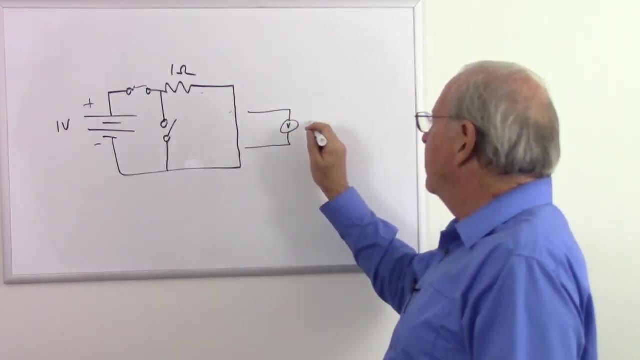 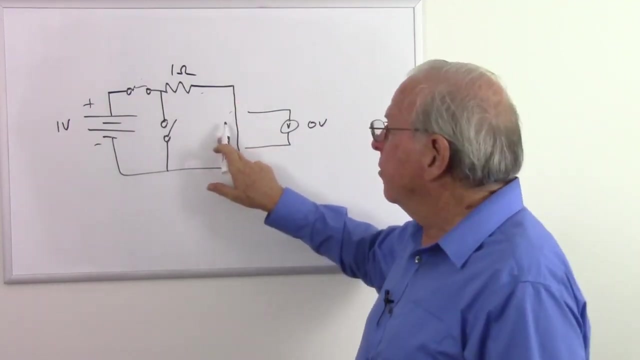 voltmeter tells us. It tells us the difference in voltage between the red lead and the black lead. So at this point here there is no difference. So it says zero volts. And how about the current? Well, right now the capacitor is basically invisible to the circuit. So all we have left 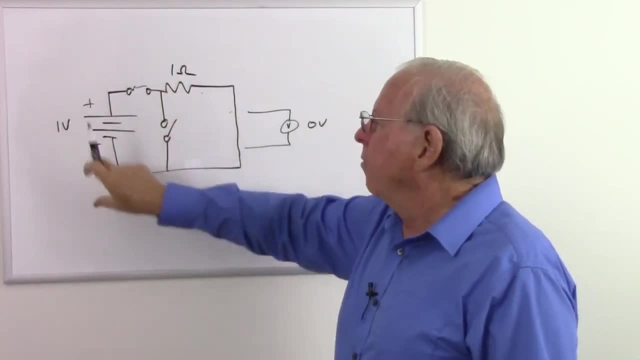 is the battery and the resistor. So it's a one volt battery, a one ohm resistor. Divide the one ohm into the one volt, We get one ohm, And that's what we get. So we get one ohm, And that's what. 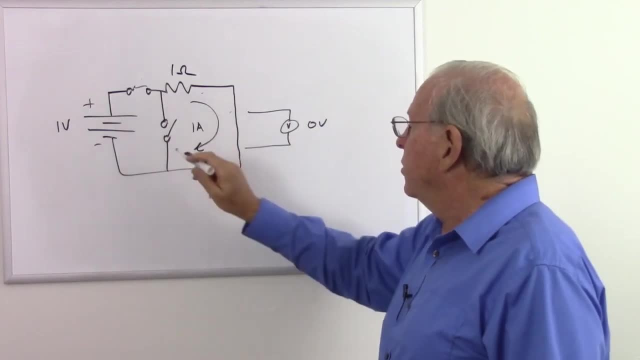 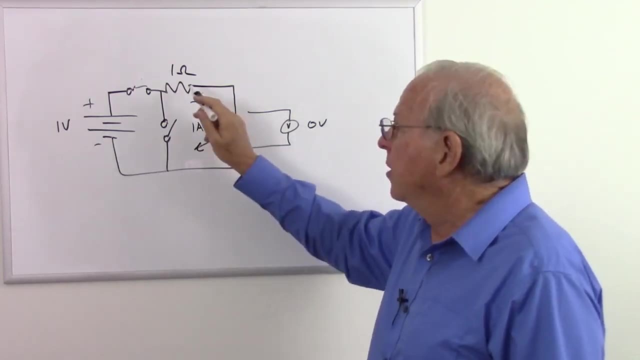 we get. So we get one amp of current. So at the moment we throw the switch, we have zero volts across the capacitor and our maximum current through the circuit. The maximum current, or the current at any time, is determined by the amount of voltage that we have across this resistor. 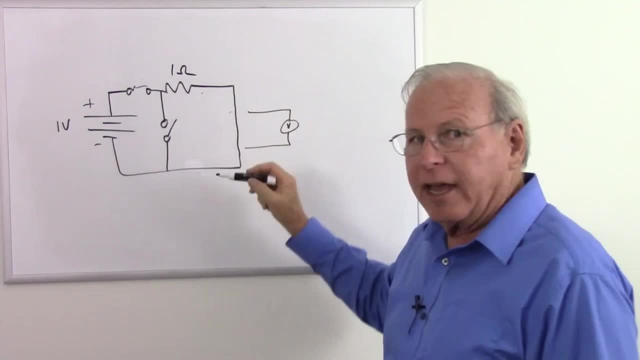 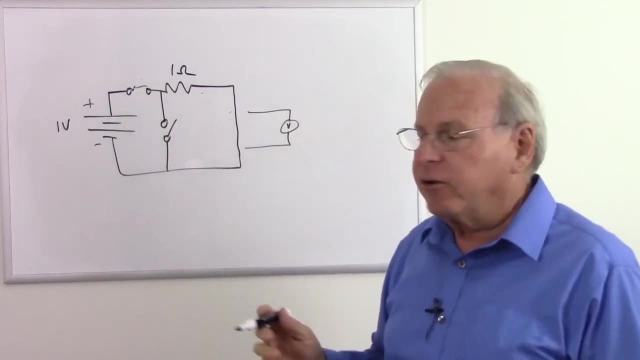 And so there's not going to be any difference in voltage from one side to the other. And what does the voltmeter tell us? It tells us the difference in voltage. One voltage is meaningless without another voltage to compare it to, and that's what a. 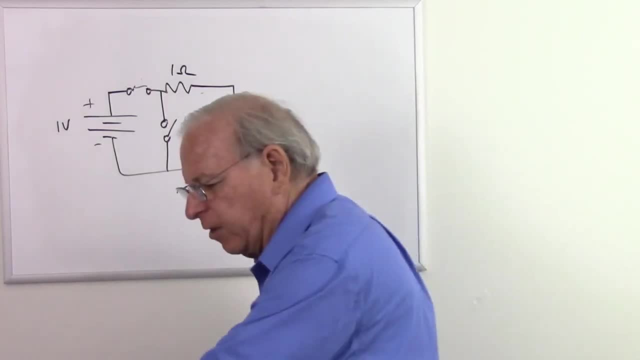 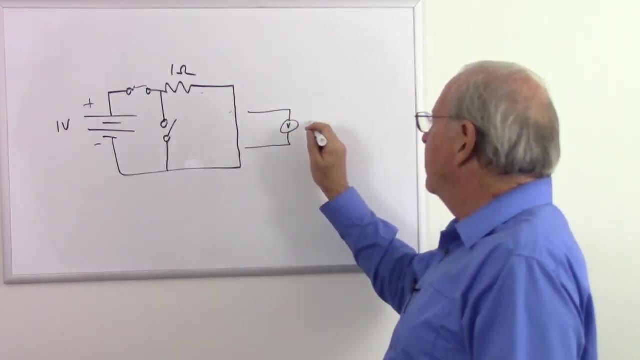 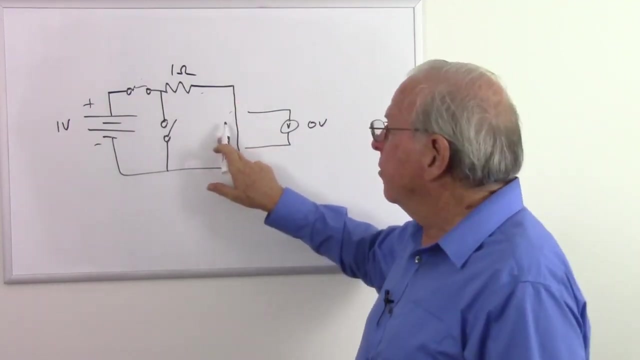 voltmeter tells us. It tells us the difference in voltage between the red lead and the black lead. So at this point here there is no difference. So it says zero volts. And how about the current? Well, right now the capacitor is basically invisible to the circuit. So all we have left 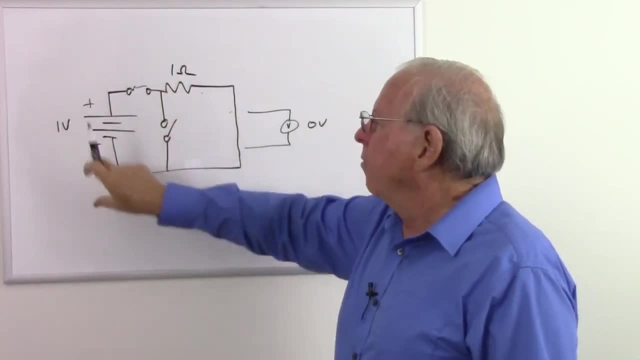 is the battery and the resistor. So it's a one volt battery, a one ohm resistor. Divide the one ohm into the one volt, We get one ohm, And that's what we get. So we get one ohm, And that's what. 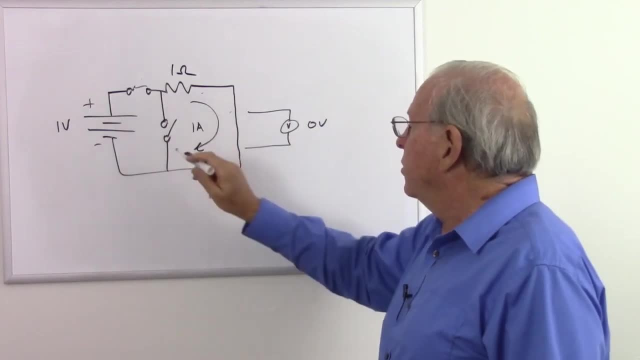 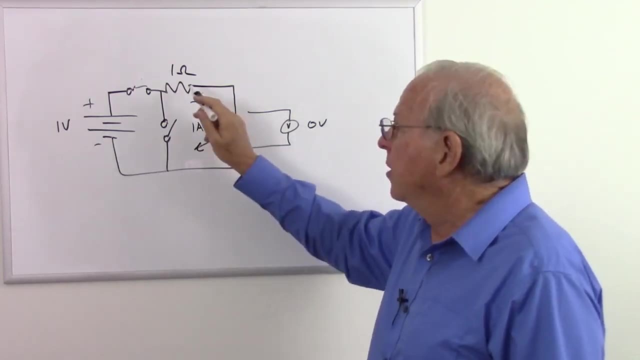 we get. So we get one amp of current. So at the moment we throw the switch, we have zero volts across the capacitor and our maximum current through the circuit. The maximum current, or the current at any time, is determined by the amount of voltage that we have across this resistor. 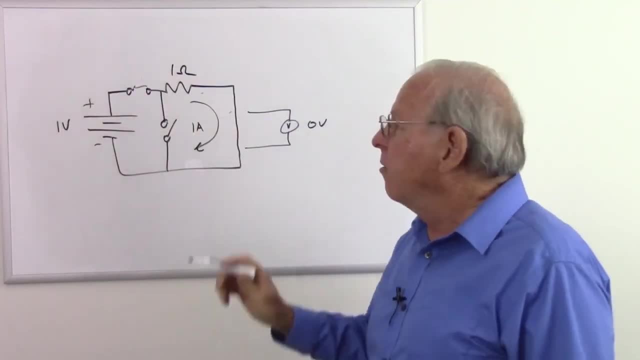 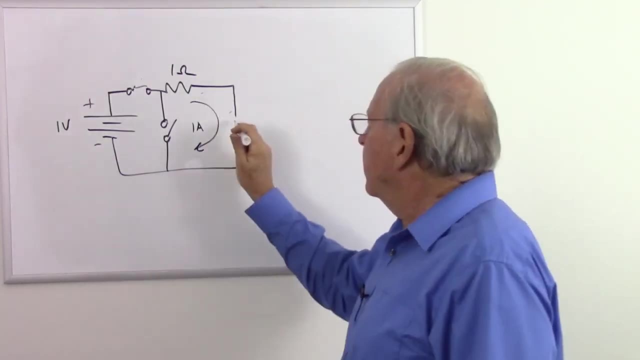 Right now that's just one volt, one ohm, one amp. Okay, but as time goes by that capacitor is going to charge And it's like putting air into an air tank or maybe a tire: You put a little air in. 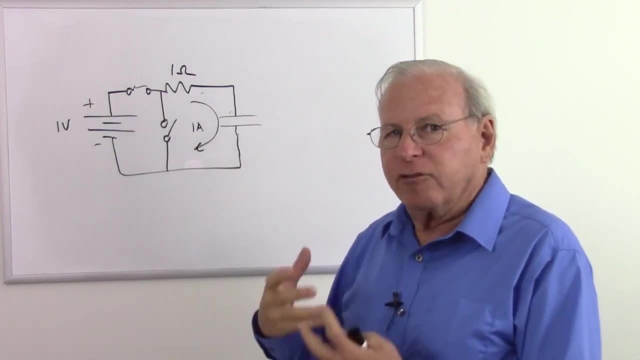 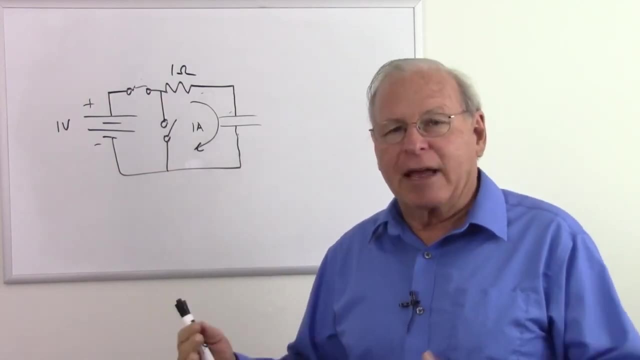 you get some pressure, You put more air in, you get more pressure. And as you put more and more air in, you get more and more pressure, until one of two things happens: Either you can't put any more because your tire is pushing back as hard as your pump is, or the tire explodes, or the air tank. 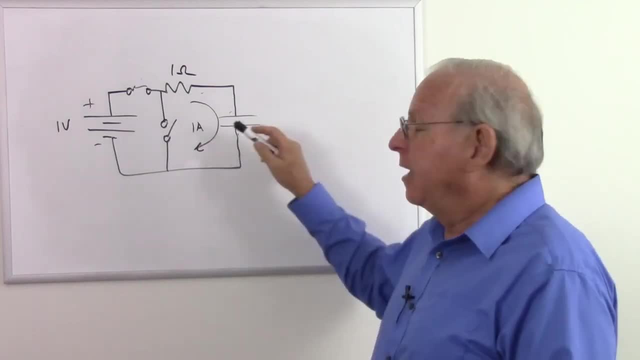 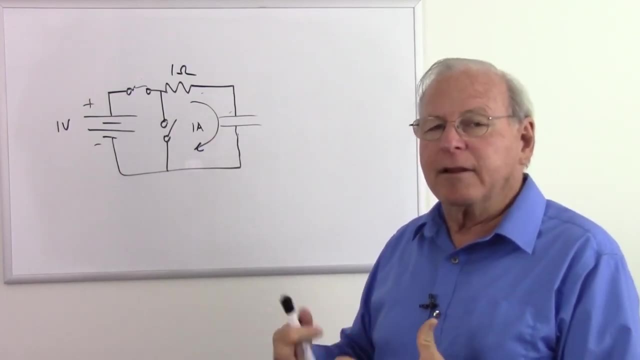 explodes. A capacitor works exactly the same way, except of course voltage is pressure. We put a little electricity and we get a little voltage. We put more in, we get more voltage, And the more we put in, the more voltage we get. until one of two things happens: Either we can't push any more 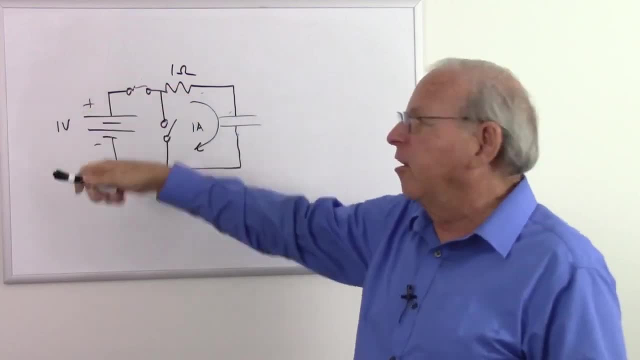 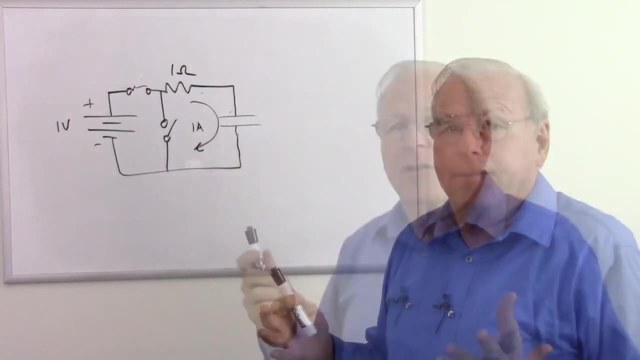 either this: This has the same voltage as our battery and it's pushing back just as hard as the battery is, so there's no current- Or the insulation fails and maybe even the capacitor could explode. So eventually, what's going to happen is this capacitor is going to charge up until 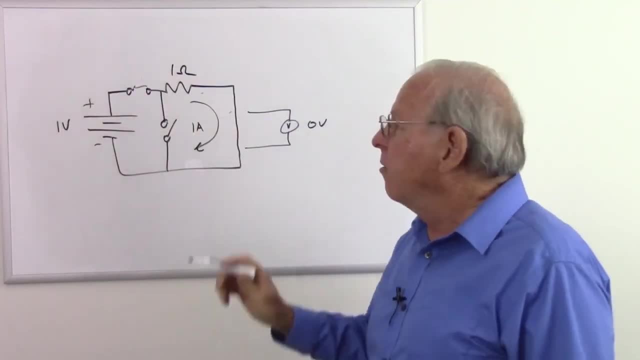 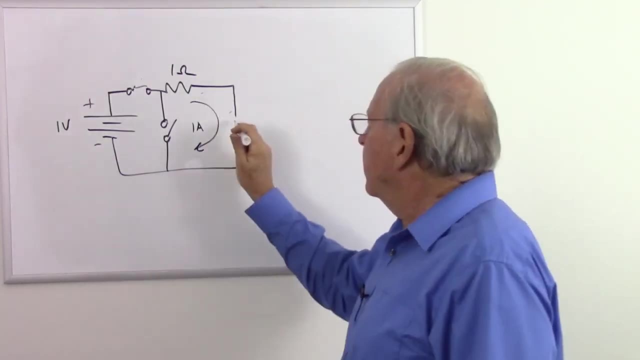 Right now that's just one volt, one ohm, one amp. Okay, but as time goes by that capacitor is going to charge And it's like putting air into an air tank or maybe a tire: You put a little air in. 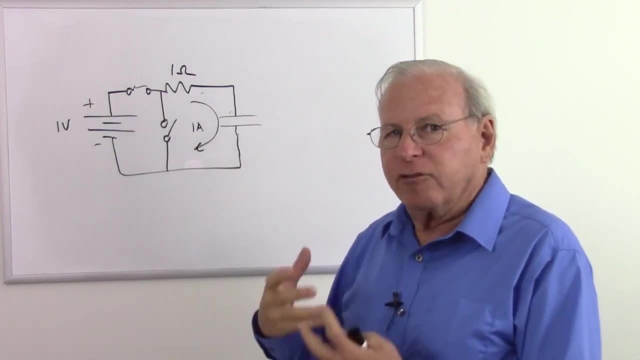 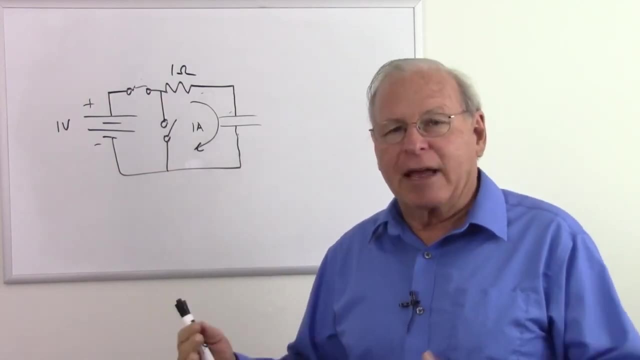 you get some pressure, You put more air in, you get more pressure. And as you put more and more air in, you get more and more pressure, until one of two things happens: Either you can't put any more because your tire is pushing back as hard as your pump is, or the tire explodes, or the air tank. 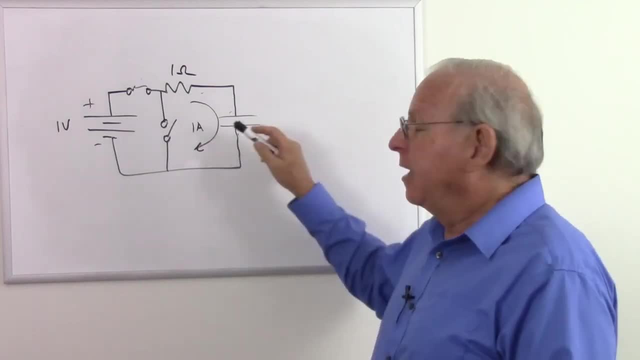 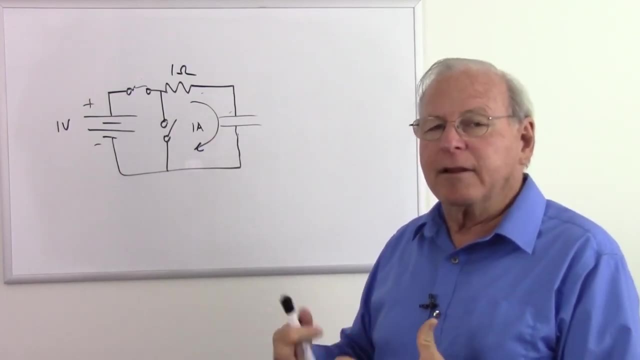 explodes. A capacitor works exactly the same way, except of course voltage is pressure. We put a little electricity and we get a little voltage. We put more in, we get more voltage, And the more we put in, the more voltage we get. until one of two things happens: Either we can't push any more 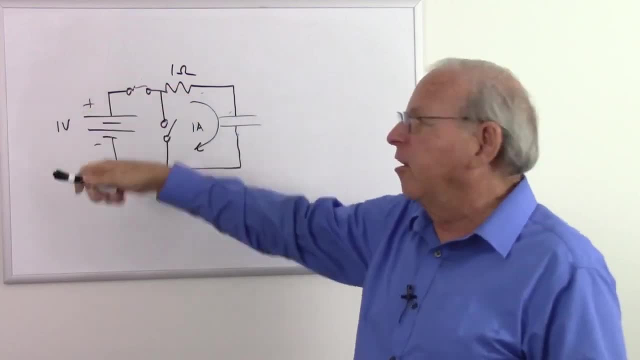 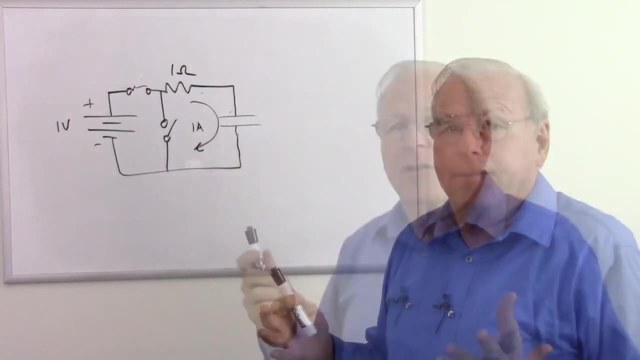 either this: This has the same voltage as our battery and it's pushing back just as hard as the battery is, so there's no current- Or the insulation fails and maybe even the capacitor could explode. So eventually, what's going to happen is this capacitor is going to charge up until 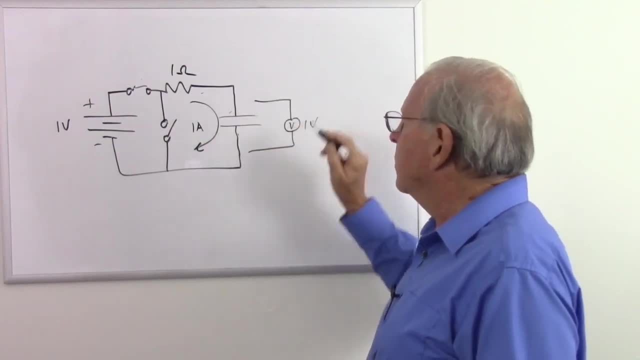 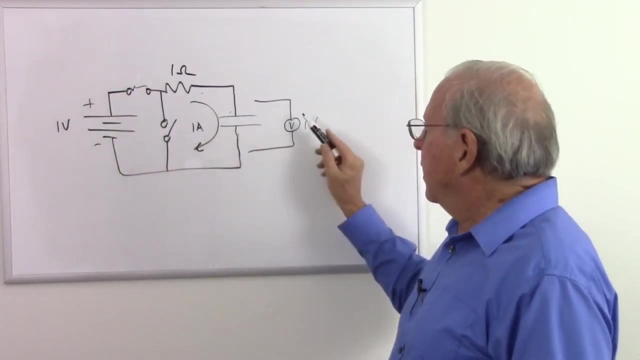 put our voltmeter across here again, it's going to have one volt And at that point the capacitor voltage is the same as our source voltage. And because this voltage is the same as that, this is pushing with one volt. That's pushing the other way with one volt, And that's 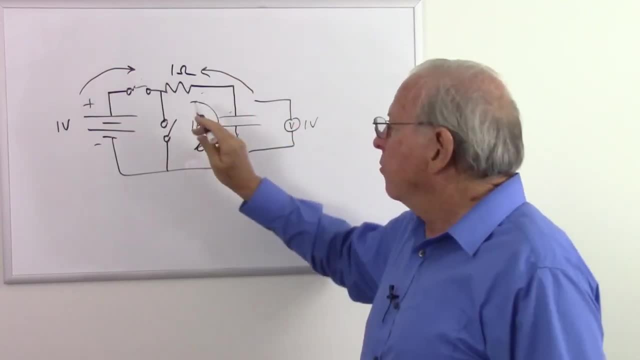 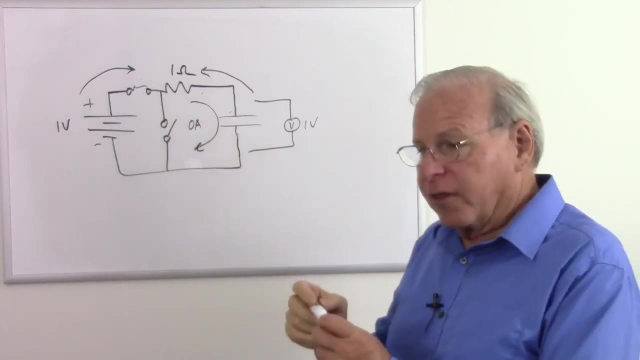 pushing the other way with one volt. How much current is flowing? None, They're pushing opposite directions, So there's no current flowing through the resistor or the rest of the circuit, so we have zero amps. So let's go ahead and draw the graph of what just happened. 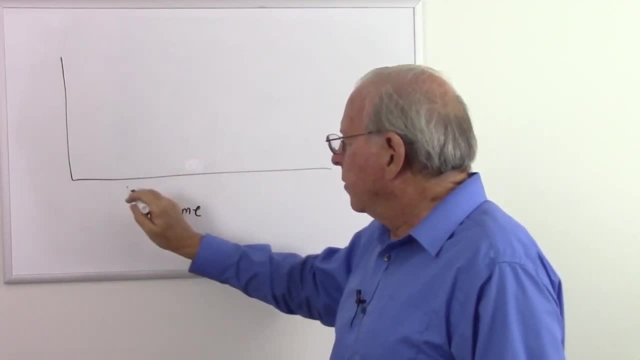 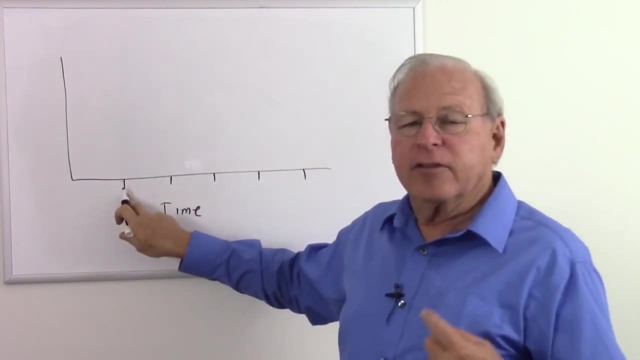 Here is time, And we'll do this in seconds. The reason I chose one ohm and one farad is because one second is the time it takes to charge the capacitor. So we're going to do this in seconds. We're going to charge the 63.2% of the source voltage And then, after five seconds, or five. 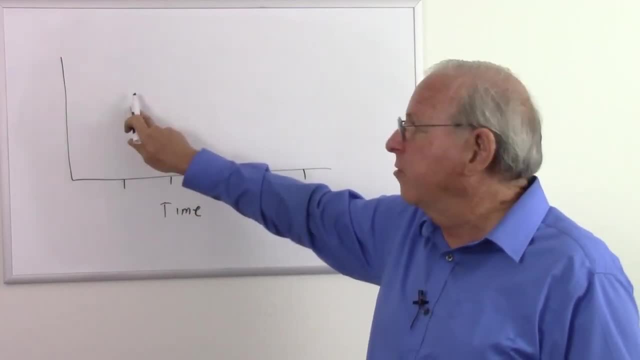 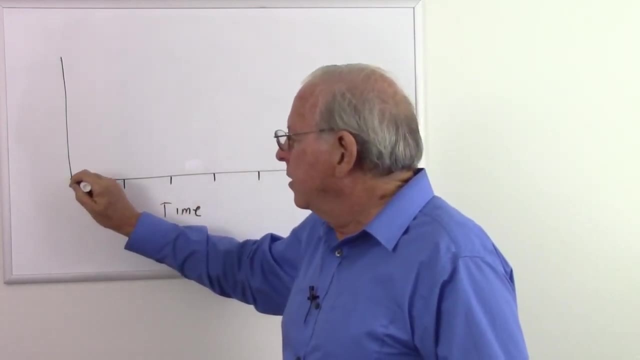 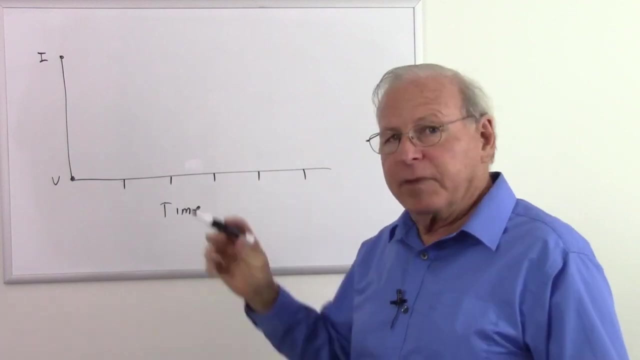 time constants. so one time constant: 63.2%. Five time constants nearest makes no difference: 100%. So remember what happened when we closed that switch. Here's our voltage, Here's our current. Remember our voltage was zero because the capacitor looked like a short circuit. 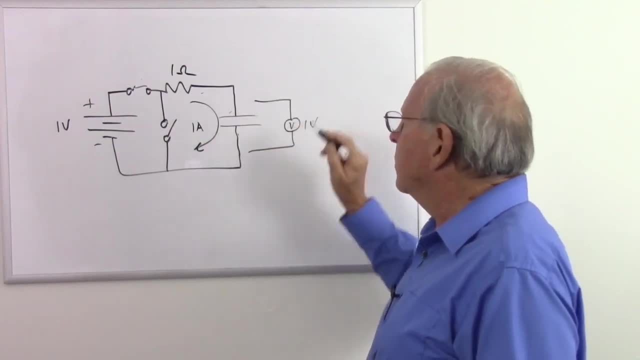 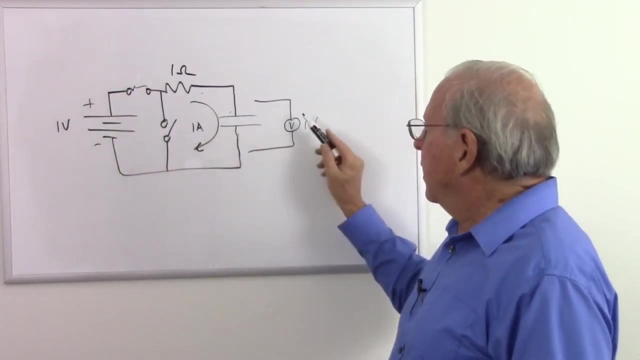 put our voltmeter across here again, it's going to have one volt And at that point the capacitor voltage is the same as our source voltage. And because this voltage is the same as that, this is pushing with one volt. That's pushing the other way with one volt, And that's 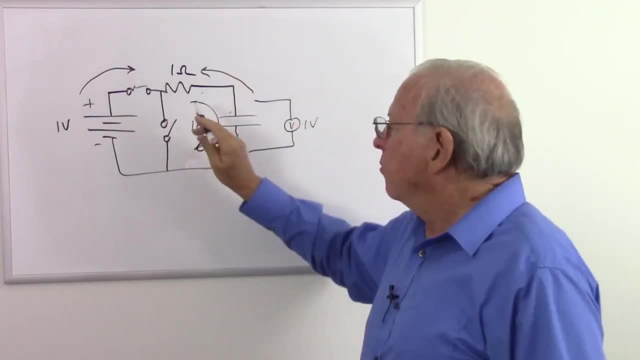 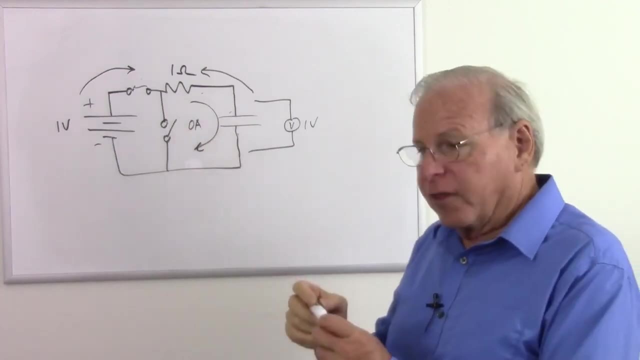 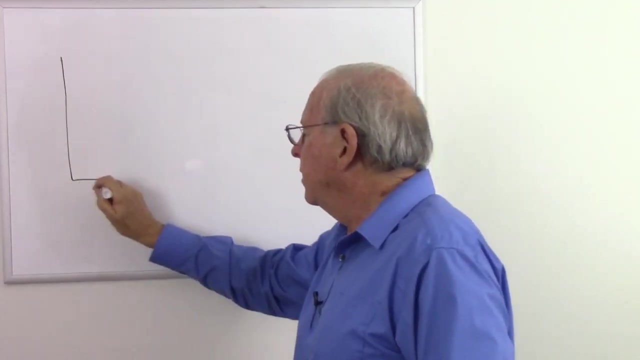 pushing the other way with one volt. How much current is flowing? None, They're pushing opposite directions, So there's no current flowing through the resistor or the rest of the circuit, so we have zero amps. So let's go ahead and draw the graph of what just happened. Here is time, And 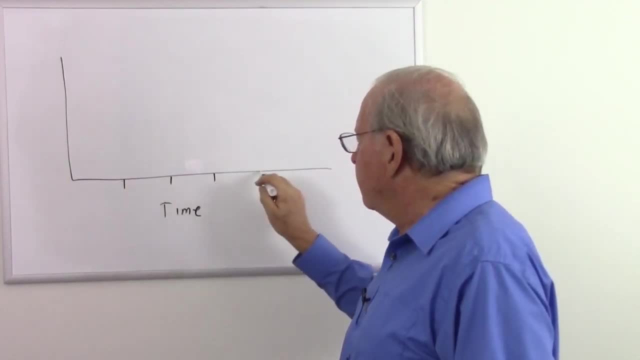 we'll do this in seconds. The reason I chose one ohm and one farad is because one second is the time it takes to charge up. So we're going to do this in seconds And we're going to do this in seconds. So we're going to do this in seconds And we're going to do this in seconds And we'll. 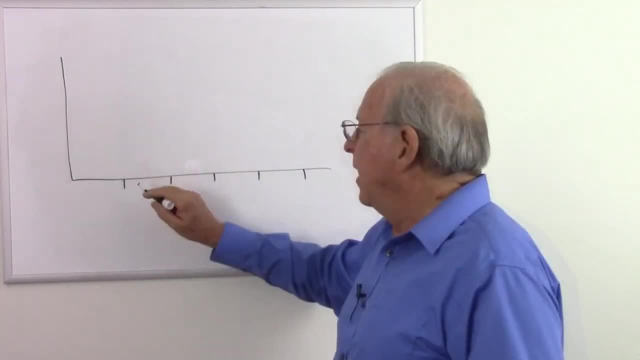 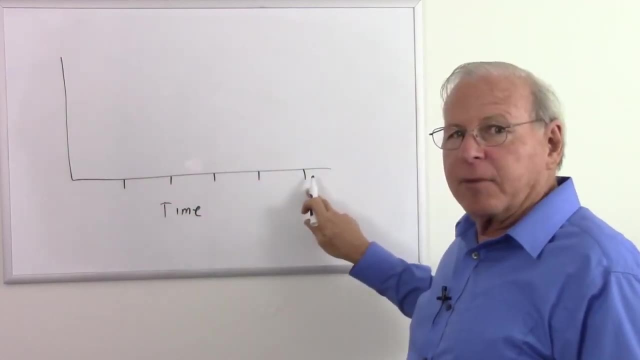 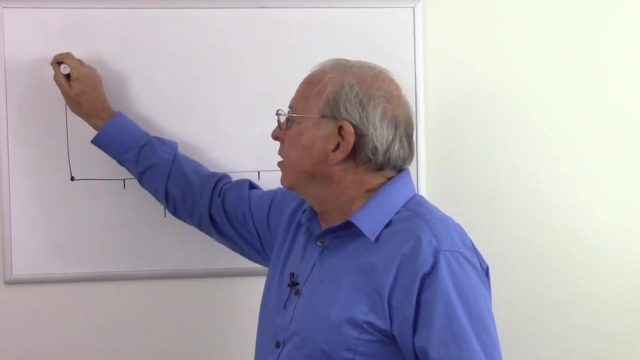 charge to 63.2% of the source voltage And then after five seconds or five time constants. so one time constant, 63.2%, Five time constants- nearest makes no difference- 100%. So remember what happened when we closed that switch. Here's our voltage, Here's our current. Remember our. 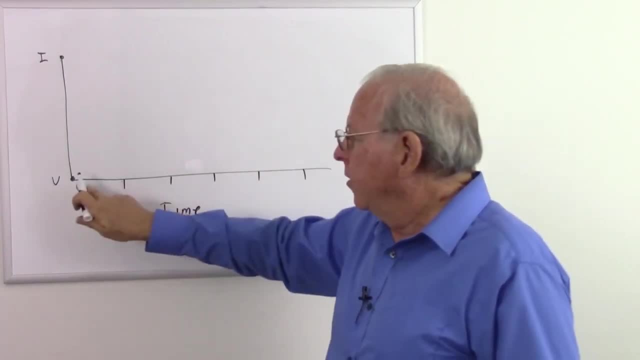 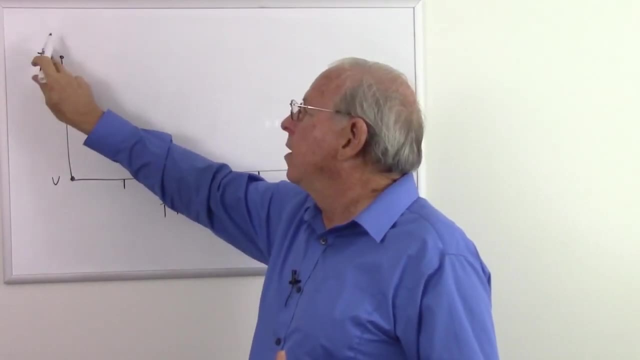 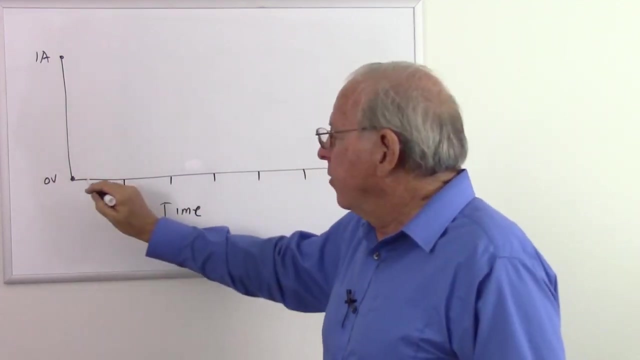 voltage was zero because the capacitor looked like a short circuit. So zero volts maximum current. What was it? We had one volt, One ohm We had- let's just draw it like one amp. So zero volts and one amp, That's going to charge. 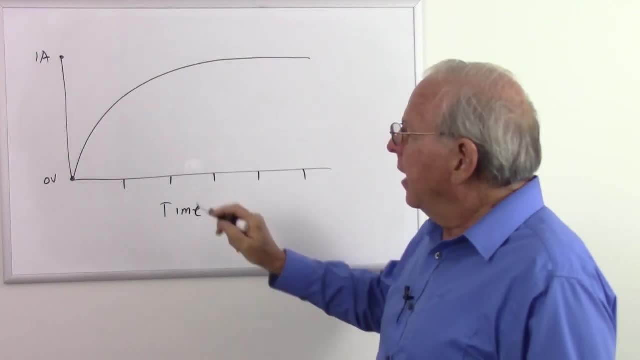 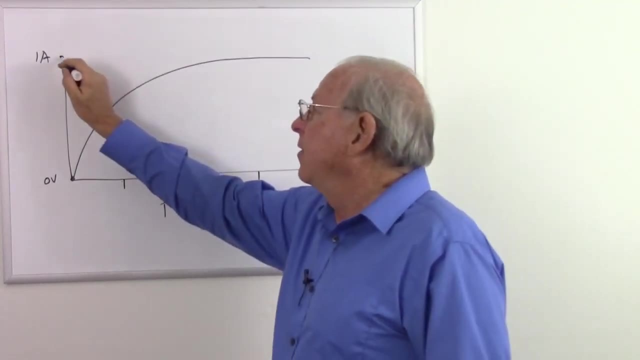 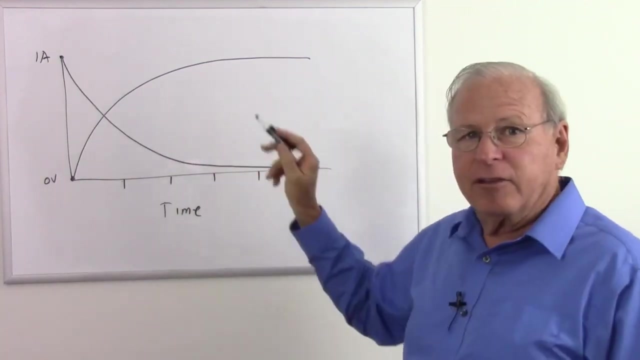 up on a curve that looks something like that, And the current as that capacitor charges, it pushes back more and more, And so we get less and less current, And then we eventually, after the same amount of time, we have no current. So after about five seconds in the case of that circuit, we just 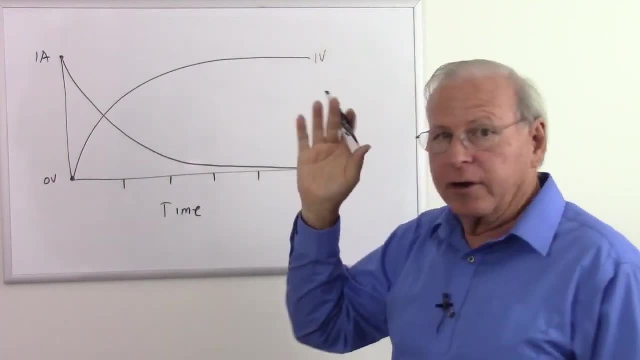 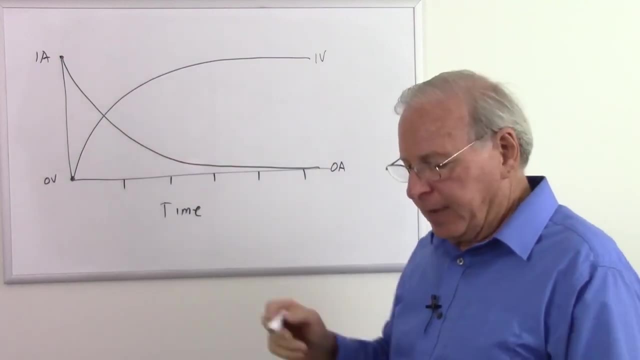 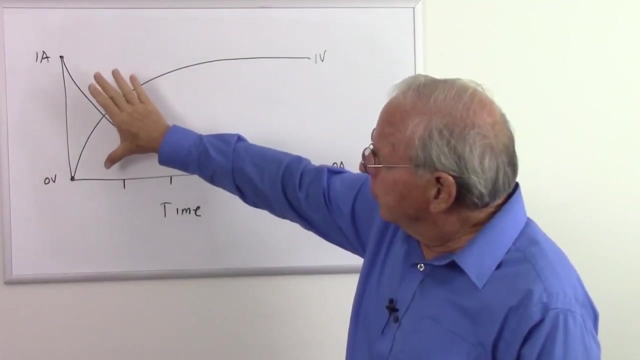 our capacitor has charged up to one volt, or our source voltage, And our current is now at zero amps. So a couple of important points there. When we first flip the switch, the capacitor looks like a short circuit. Let's go ahead and remember this graph. This is when we flip the switch. 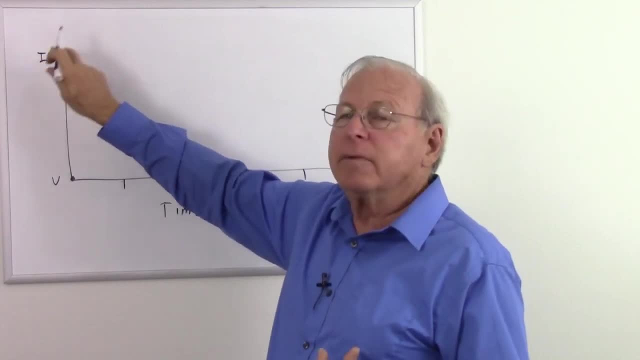 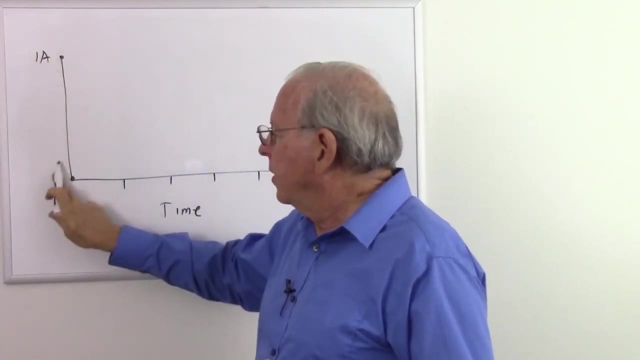 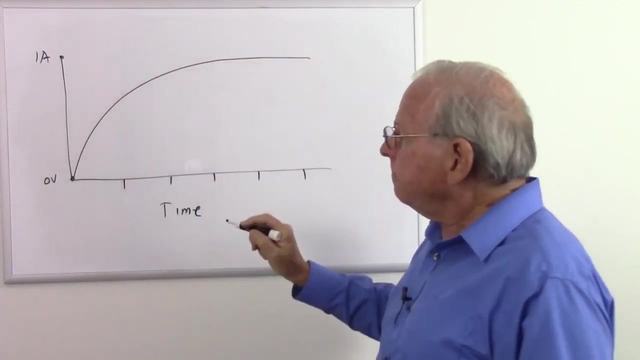 So zero volts maximum current, What was it? We had one volt, one ohm, We had- let's just draw it like one amp. So zero volts and one amp That's going to charge up on a curve that looks something like that, And the current as that capacitor charges. 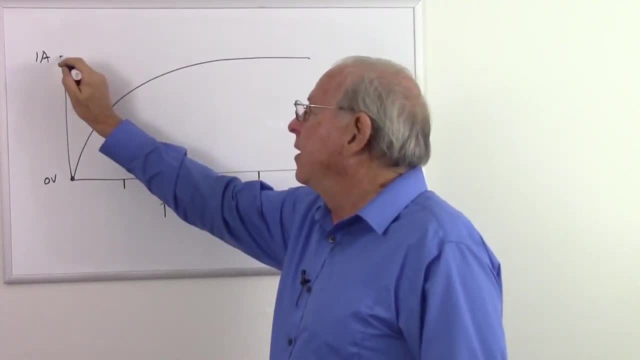 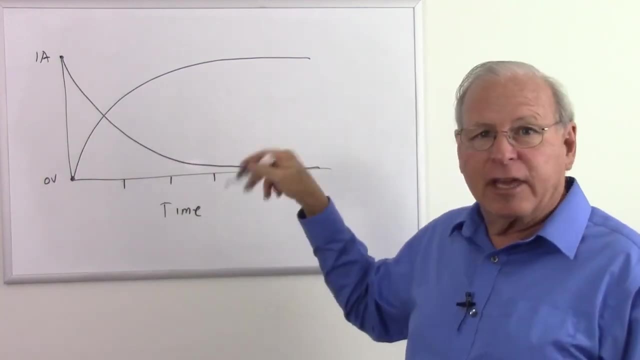 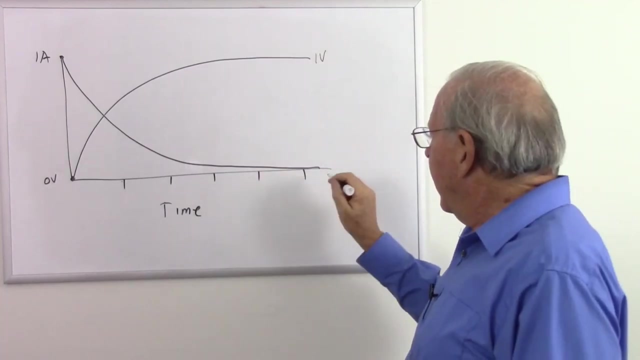 it pushes back more and more, And so we get less and less current, And then we eventually, after the same amount of time, we have no current. So after about five seconds, in the case of that circuit we just had, our capacitor has charged up to one volt, or our source voltage, and our current is now at 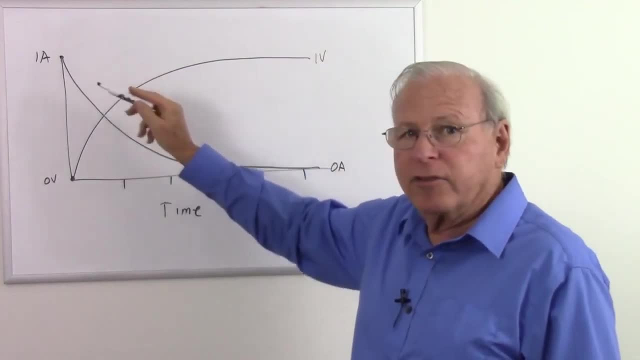 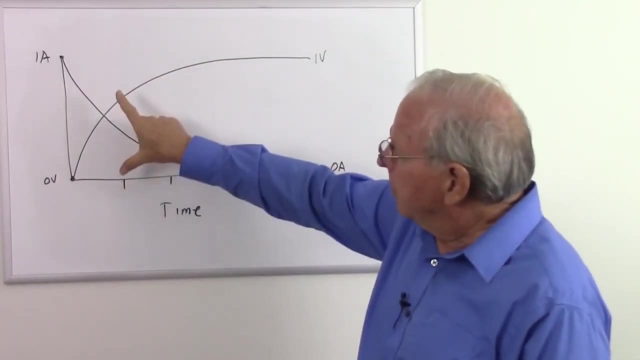 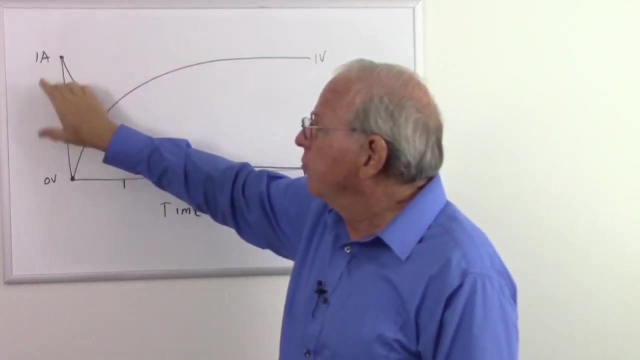 zero amps. So a couple of important points there. When we first flip the switch, the capacitor looks like a short circuit. Let's go ahead and remember this graph. This is when we flip the switch. This is about five seconds later with that particular circuit. We flip the switch. We 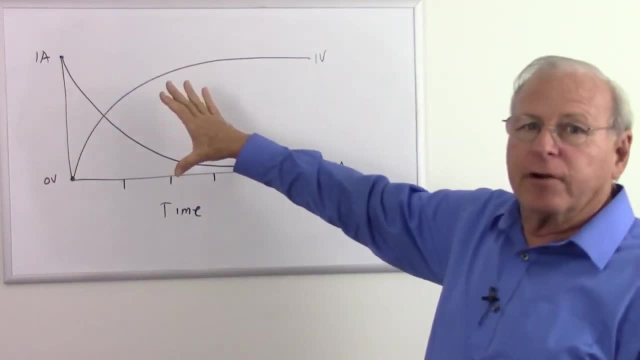 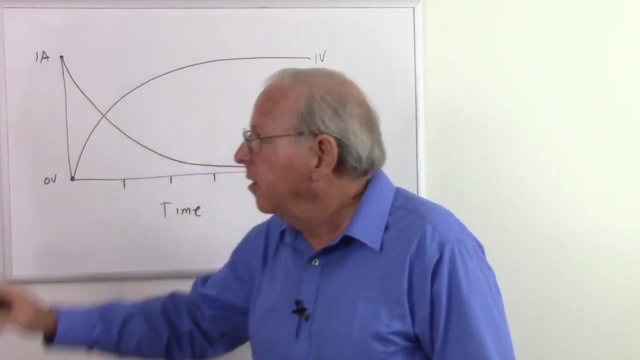 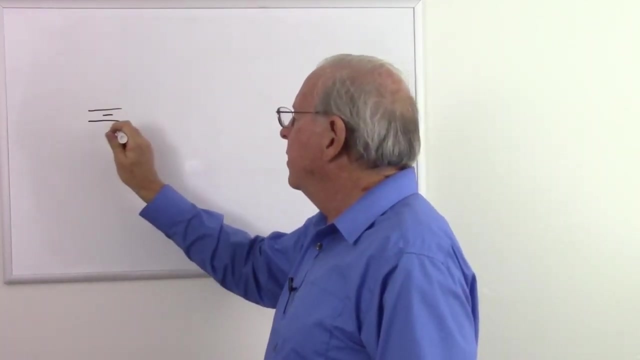 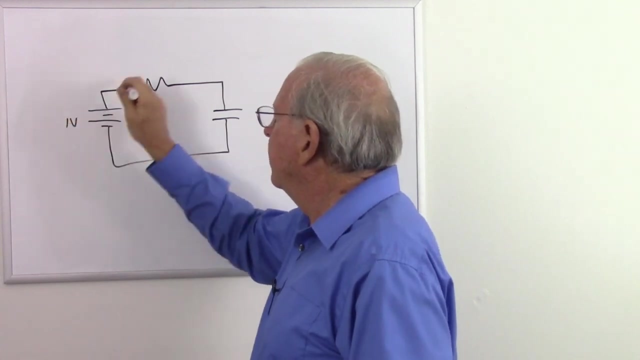 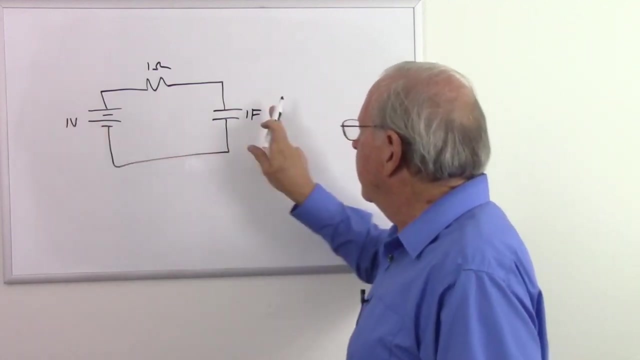 have our maximum current and zero volts After about five time constants- five seconds in this case. we have our maximum voltage and zero current. So let's take another quick look at what's going on there with our circuit. I'll forego the switches at this time. At the time we threw the switch, we had one volt here. 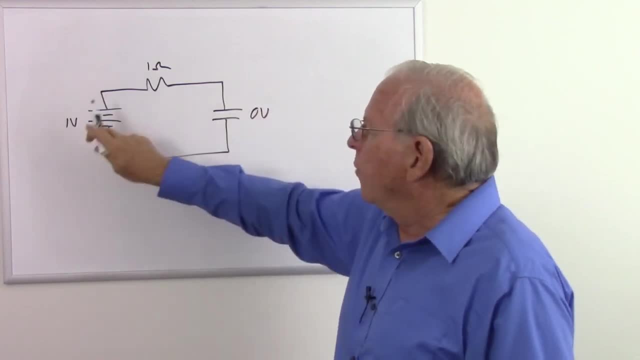 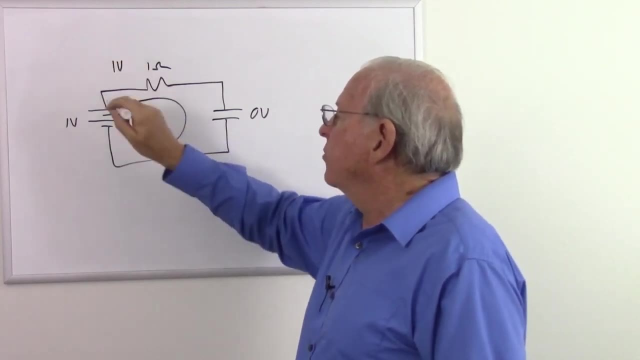 and zero volts here. So we had one volt here and zero volts here. So we had one volt here and zero volts here. One volt across the capacitor, so we had one amp of current. Once again, one volt on this side, zero volts on that side, So we have one amp of current After. 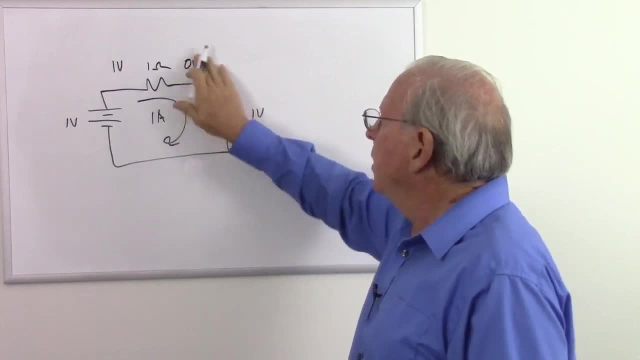 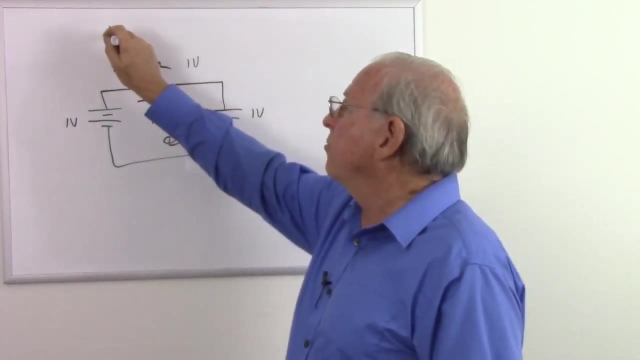 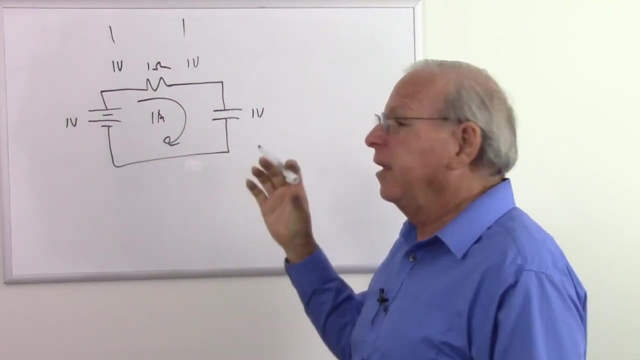 five seconds. this is up to one volt. So now we have one volt on this side and one volt on this side, So we have the same voltage on both sides. How much voltage is that? Remember, if the voltage is the same on both sides, that, by definition, is zero volts. It's the difference in voltage. Zero volts is not a voltage. 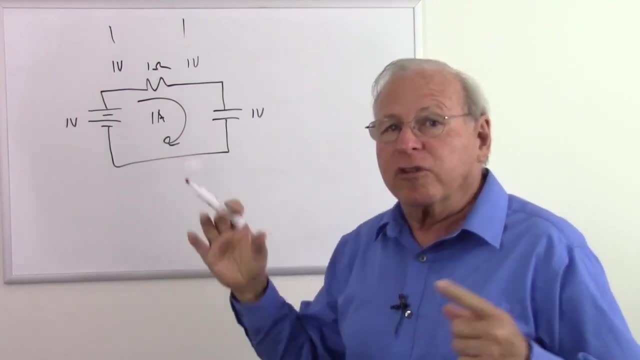 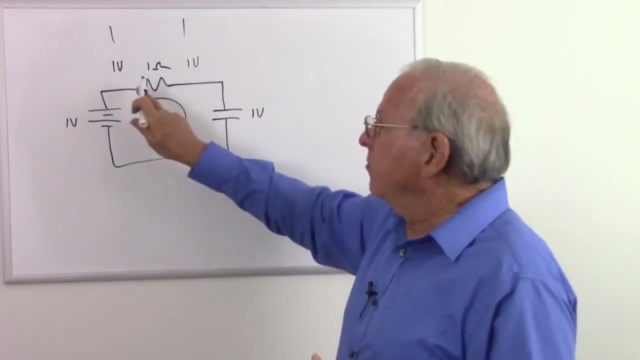 It's not the absence of voltage. Zero volts simply means that two voltages are the same. Typically, it means that the red probe of our volt meter is at the same voltage as our black lead, But what it means is that two voltages are the same. There is zero difference, So zero volts. 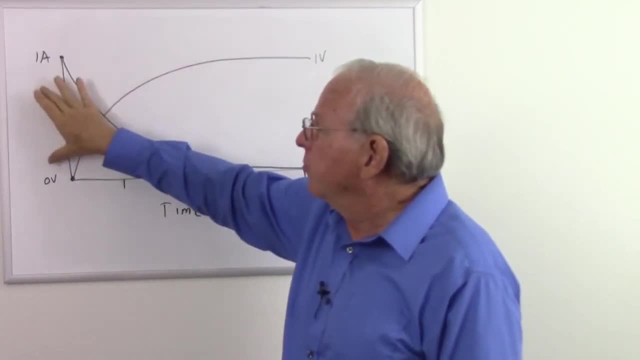 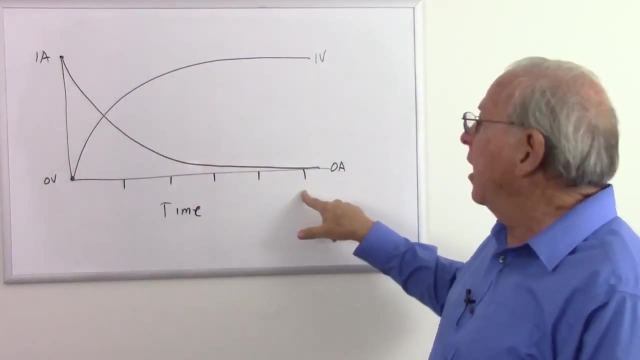 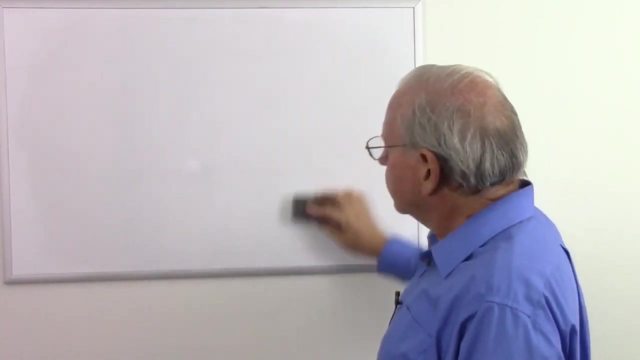 This is about five seconds later with that particular circuit. We flip the switch, we have our maximum current and zero volts. After about five time constants- five seconds in this case- we have our maximum voltage and zero current. So let's take another quick look at what's going on there with our circuit. 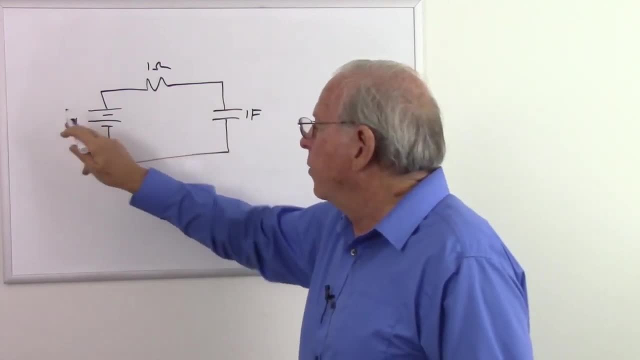 I'll forgo the switches at this time. At the time we threw the switch we had one volt here and zero volts here, So we had one ohm and a nap. So we've got bigger circuit down here And then if you flip the switch for the second half a bar it takes another 15 volts and 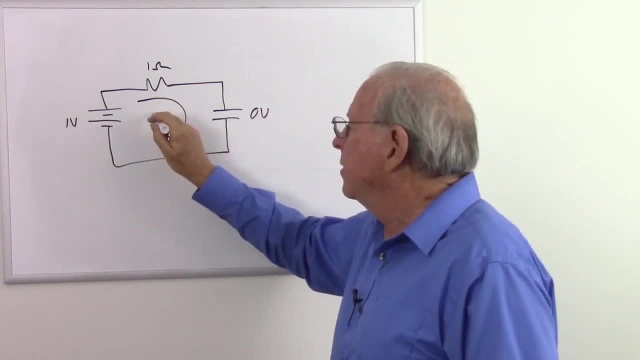 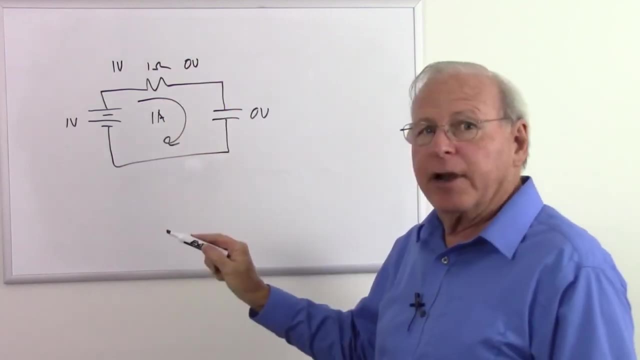 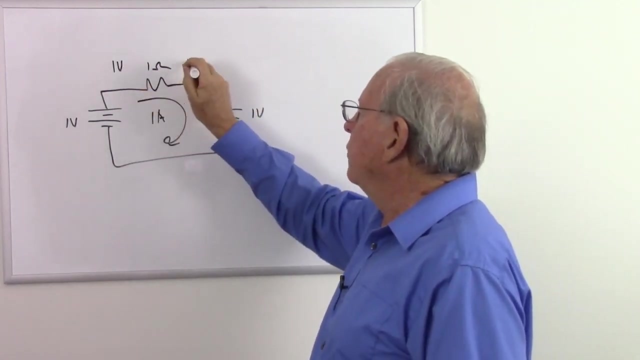 volt across the capacitor. so we had one amp of current. once again, one volt on this side, zero volts on that side, so we have one amp of current after five seconds this is up to one volt. so now we have one volt on this side and one volt. 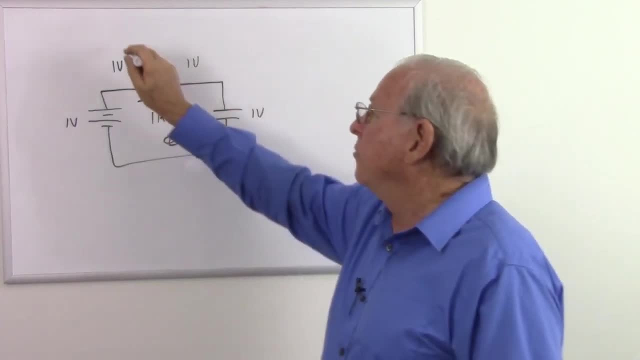 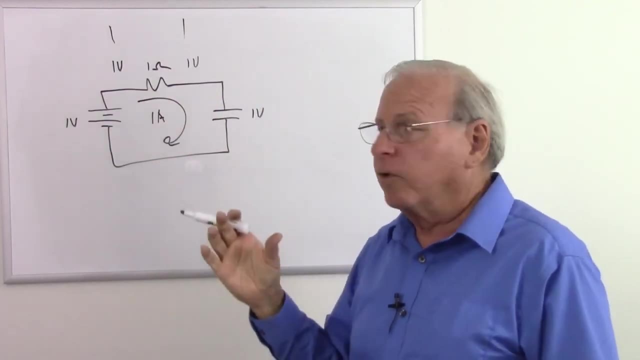 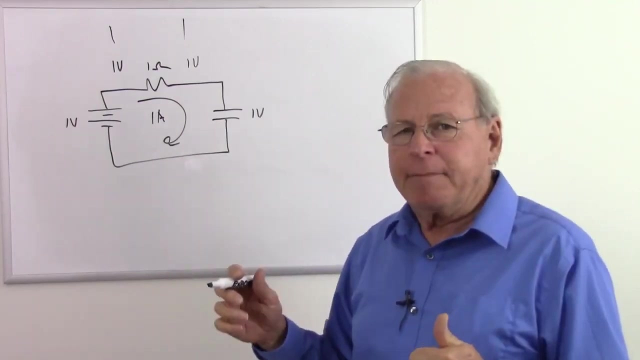 on this side, so we have the same voltage on both sides. how much voltage is that? remember, if the voltage is the same on both sides, that, by definition, is zero volts. it's the difference in voltage. zero volts is not the absence of voltage. zero volts simply means that two voltages are the same. typically it 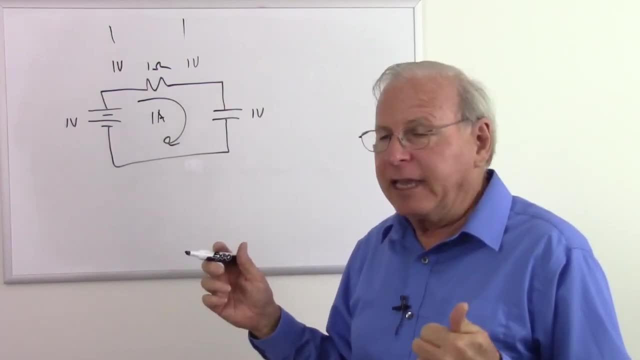 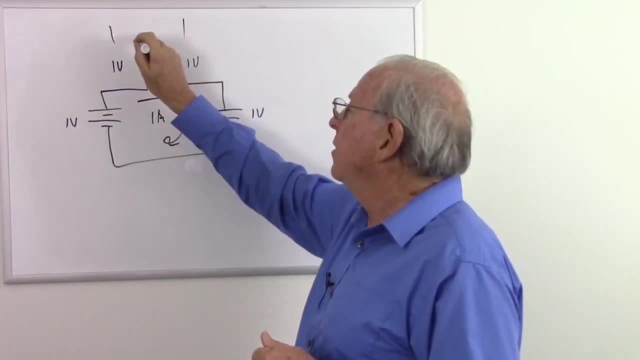 means that the red probe of our voltmeter is at the same voltage as our black lead, but what it means is that two voltages are the same. there is zero difference, so zero volts. so at first one volt and zero volts, a total of one volt. 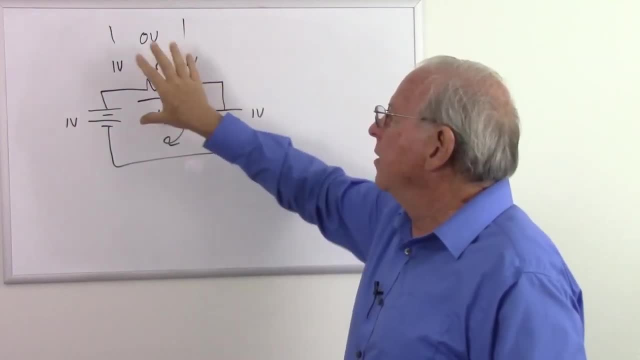 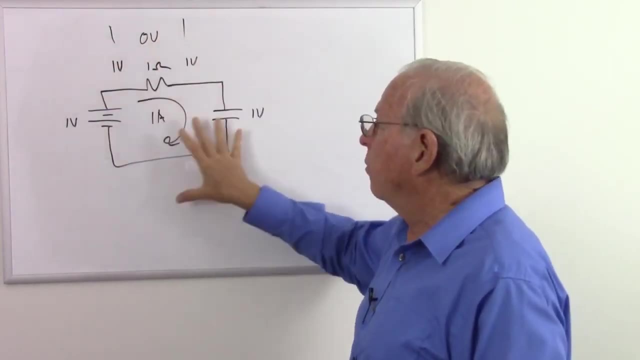 across the capacitor. after a while, we have one volt here, one volt there and zero volts across it. remember this, because this is part of what causes the phase angle: is these changes in voltage across the resistor. so now what we're going to do is take a look at an AC circuit and 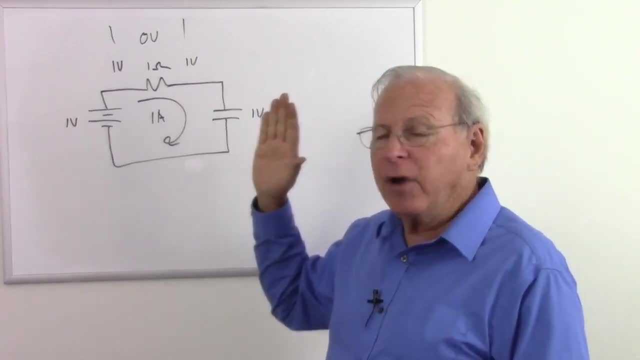 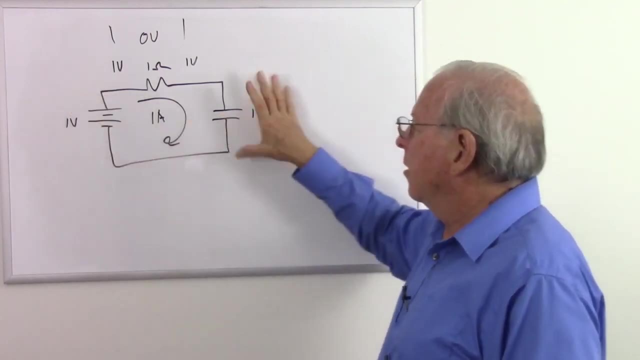 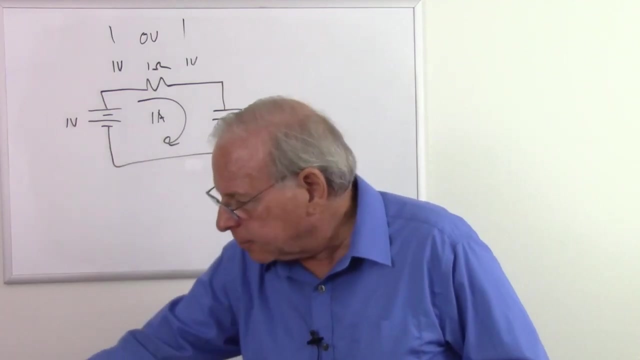 analyze it at different points in time and see how it acts like a DC circuit, but the difference is this voltage is constantly changing. instead of it being steady, the capacitor charges and stays there. this voltage is constantly changing. let's take a quick look at what would happen if this did change. so this charged up. 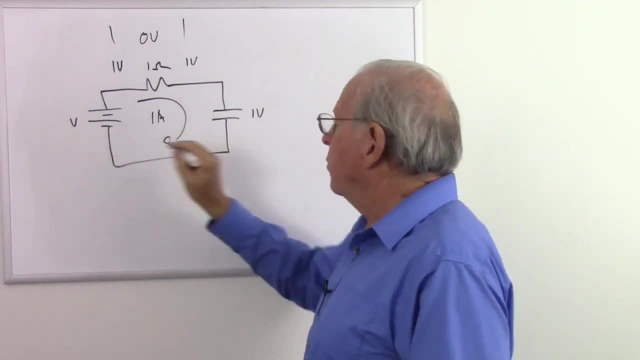 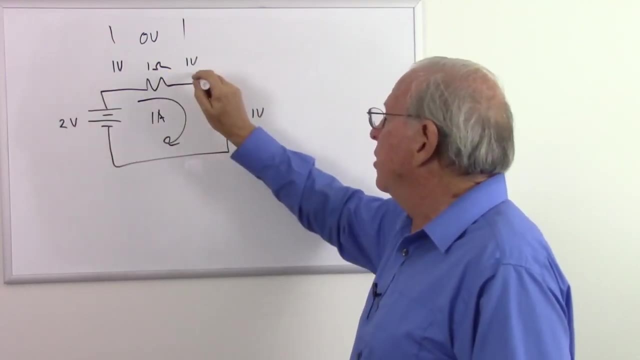 to one volt. what if this kept on going? what if, by the time this got to one volt, this was two volts? well, now, this is pushing this way harder than that. so it's not going to stop charging, it's going to continue to charge. so if this voltage goes up, that's going to continue to charge. what happens? 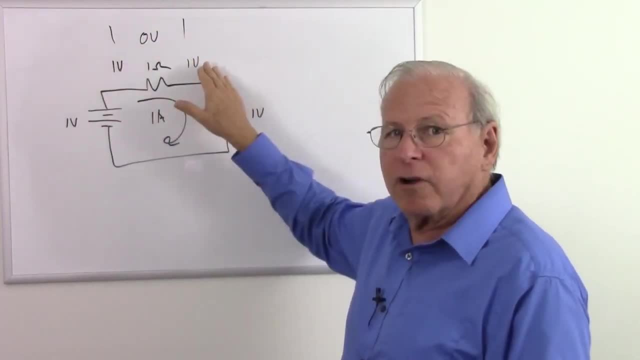 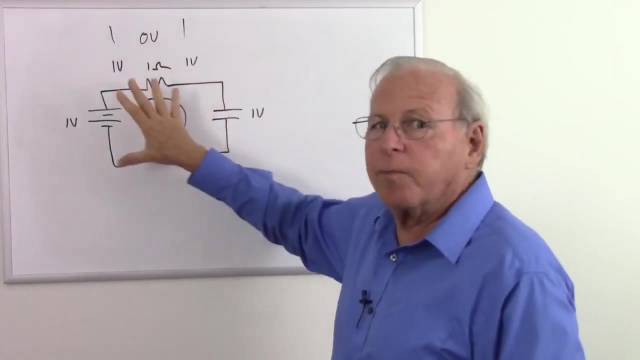 So at first, one volt and zero volts, a total of one volt across the capacitor. After a while, we have one volt here, one volt there and zero volts across it. Remember this, because this is part of what causes the phase. 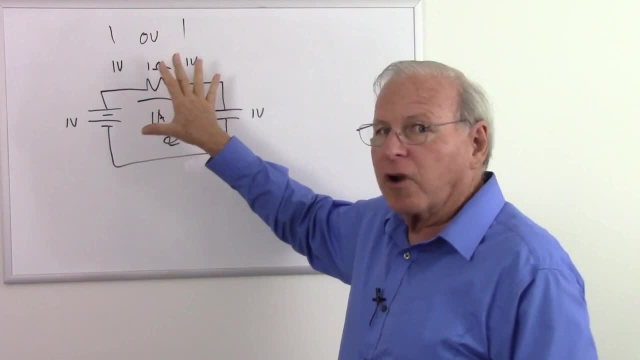 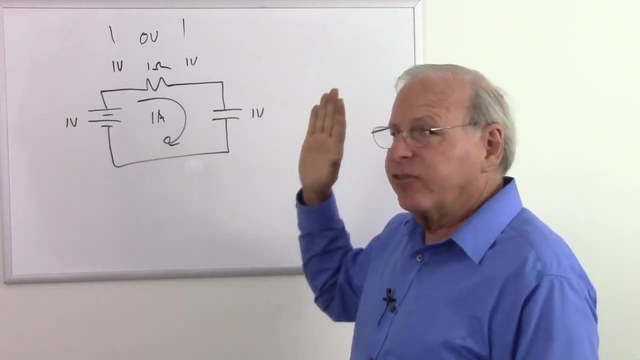 What causes the phase angle is these changes in voltage across the resistor. So now what we're going to do is take a look at an AC circuit and analyze it at different points in time and see how it acts like a DC circuit, But the difference is this voltage is constantly changing. Instead of 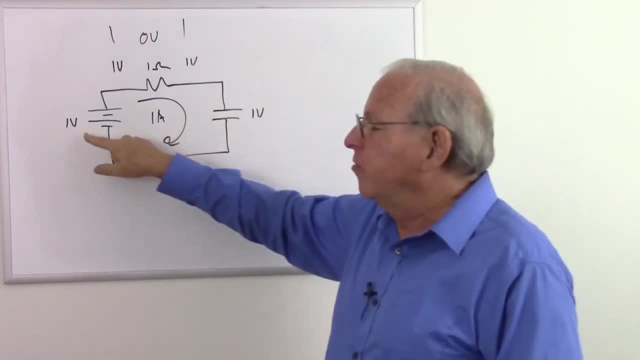 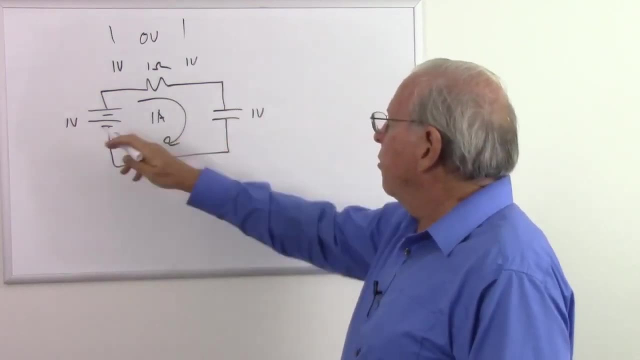 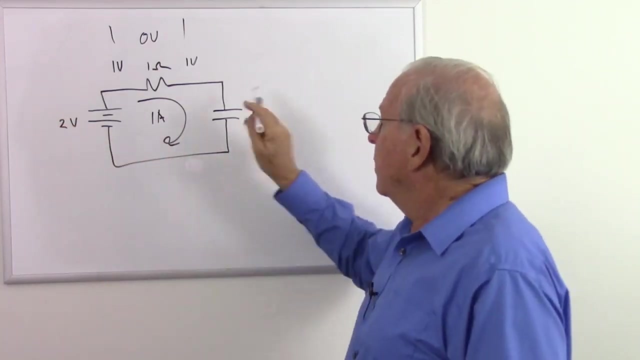 it being steady, the capacitor charges and stays there. This voltage is constantly changing. Let's take a quick look at what would happen if this did change. So this charged up to one volt. What if this kept on going? What if, by the time this got to one volt, this was two volts? Well, now, this is. 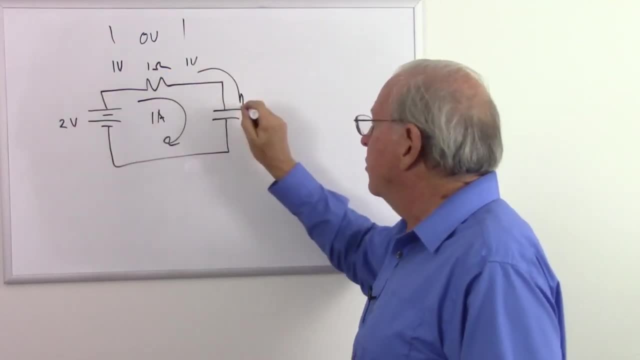 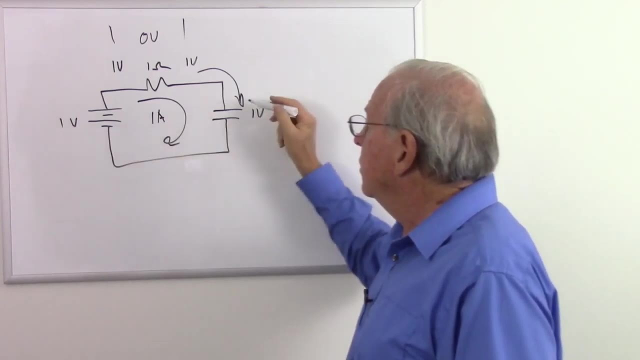 pushing this way harder than that. so it's not going to stop charging, It's going to continue to charge. So if this voltage goes up, that's going to continue to charge. What happens if this goes down? now back to one volt? Well, now, what do we have? We have something like maybe two volts here and one. 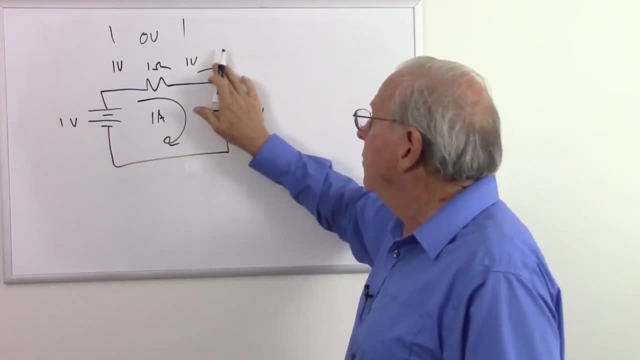 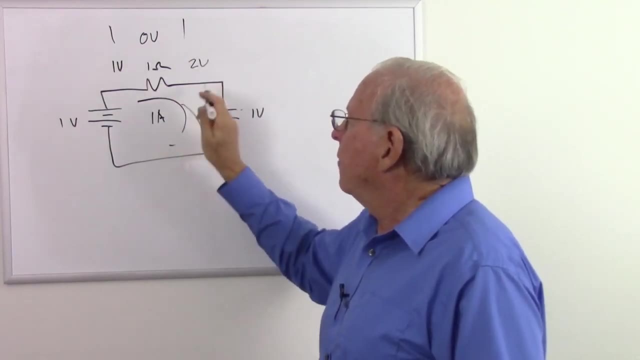 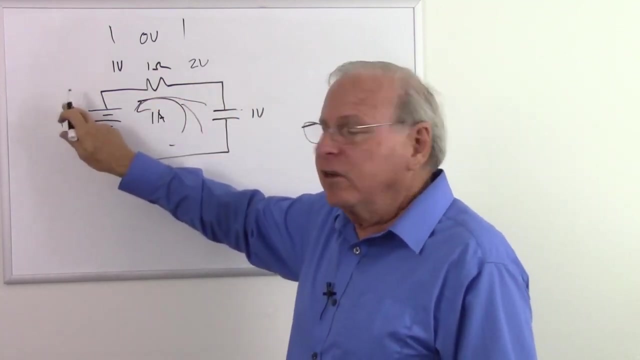 if this goes down now back to one volt, well, now what do we have? we have something like maybe two volts here and one volt there. now we have more voltage on this side than that side and it's going to push the opposite direction. so this voltage goes up. as long as this voltage is higher. 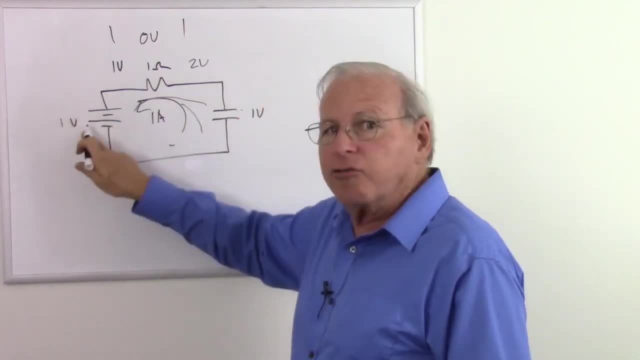 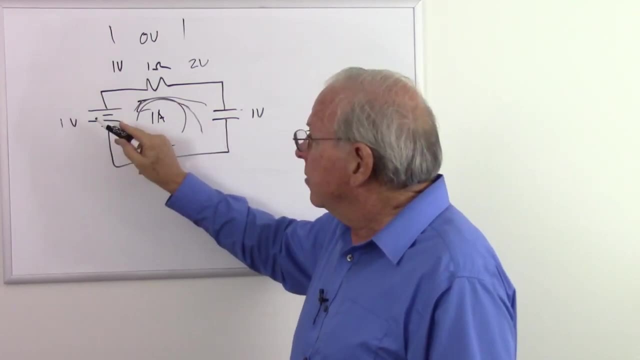 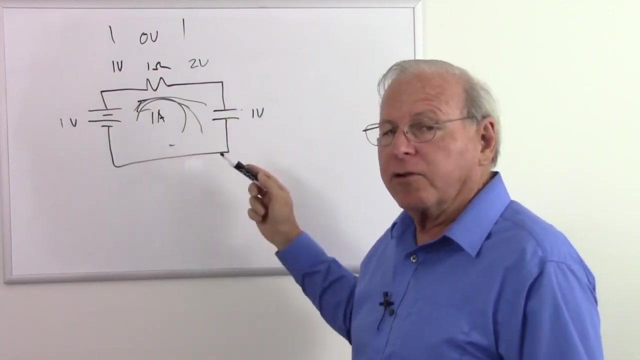 than that voltage, the capacitor will charge, but as soon as this voltage drops below the capacitor's voltage, it'll start discharging. so that's basically what the ac circuit does. it's a like a dc voltage, but the voltage is constantly changing, and if it changes in a periodic way, we call it. 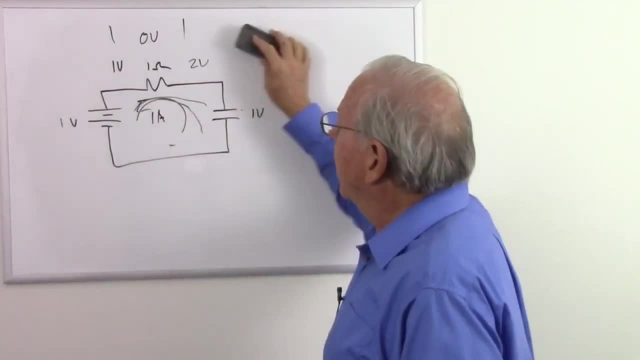 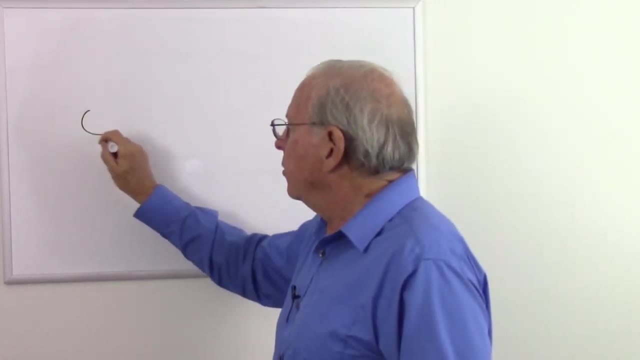 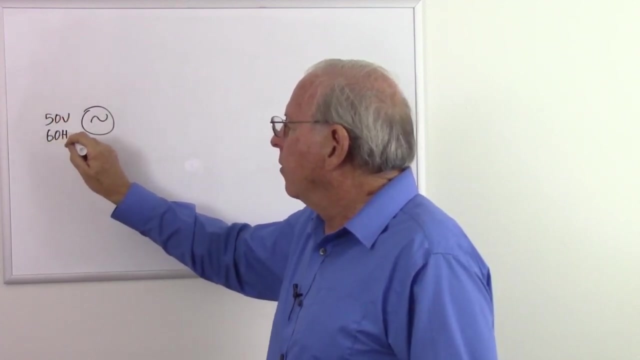 alternating current. so let's take a look at how that circuit works at different moments in time and analyze what that circuit is like, why we get a phase angle. So here's the circuit I'm going to use. There's our alternating current source. I'll use 50 volts at 60 hertz, although the frequency doesn't really matter too much at 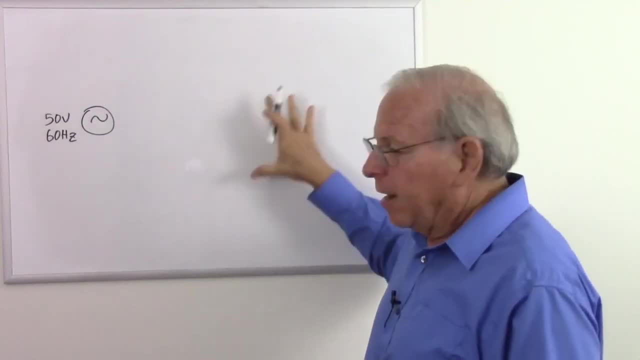 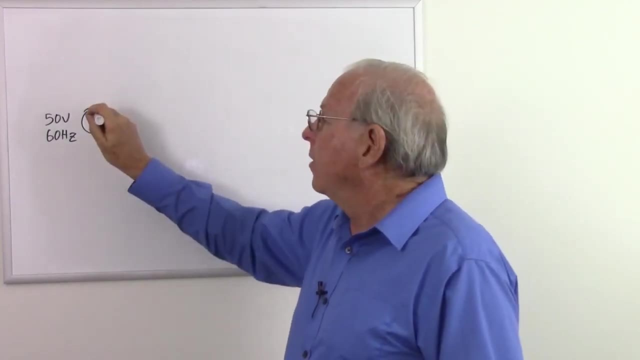 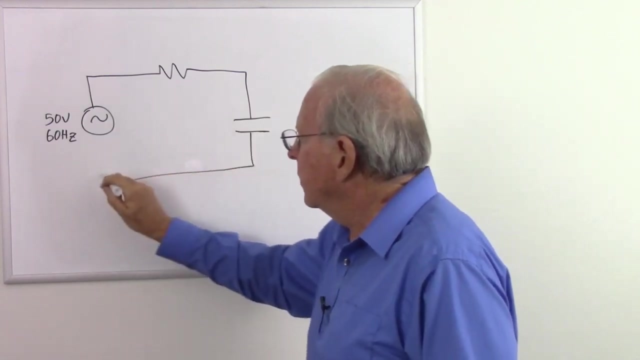 this point It matters for calculating different parameters of the circuit, but for the phase angle, what we need to know for the phase angle, it's somewhat inconsequential. So now I'm going to put a resistor here and a capacitor. I'm going to make this 30 ohms and 100 microfarads. 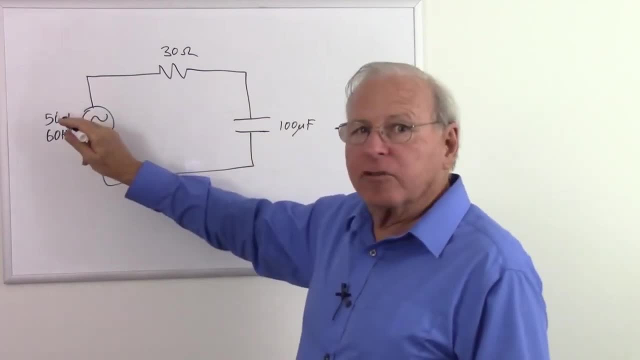 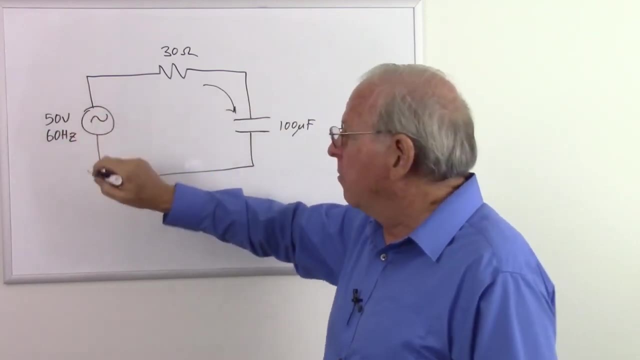 So what's going to happen with this circuit? Well, of course, this voltage is going to go up and this capacitor is going to start charging And it's going to try to charge toward. well, whatever voltage this is, Remember what's happening: That voltage is going up and down. 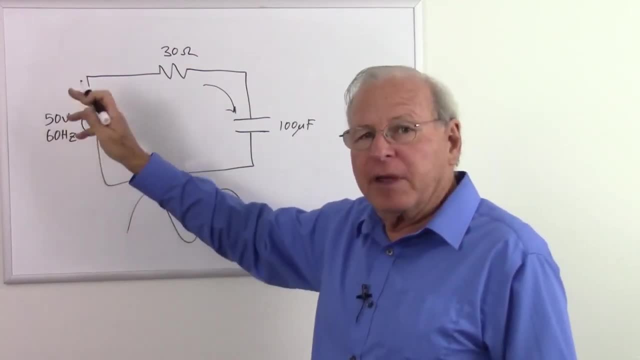 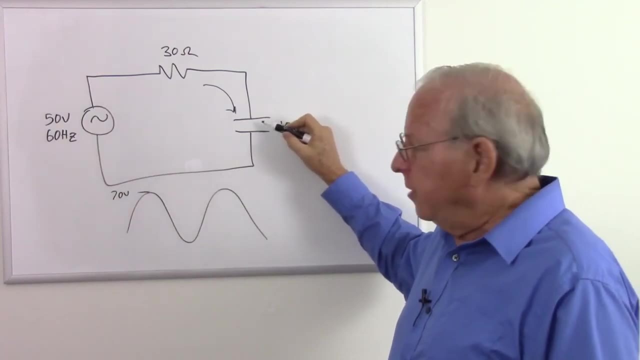 and up and down and it says 50 volts, but that's the rms voltage. it has Actually peaks at about 70 volts. So that keeps going up and up. and as that's going up and up, this is charging And then eventually that's going to drop. As long as this has not caught up. 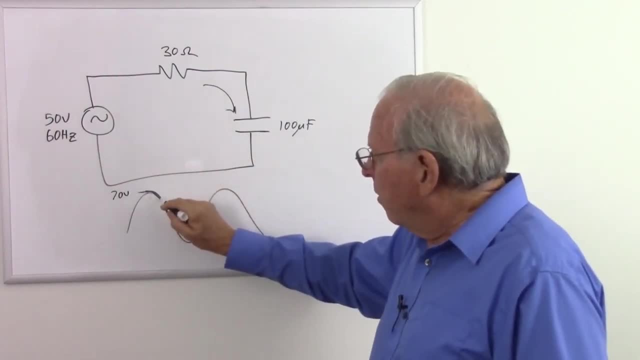 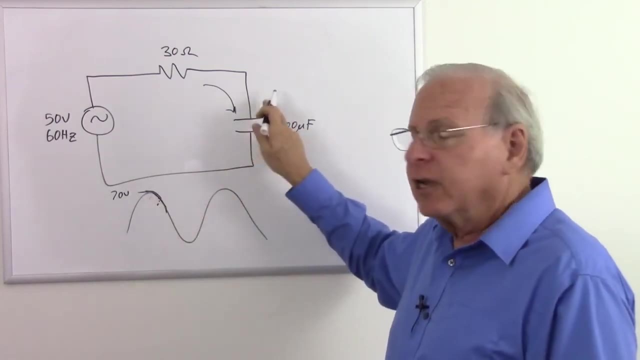 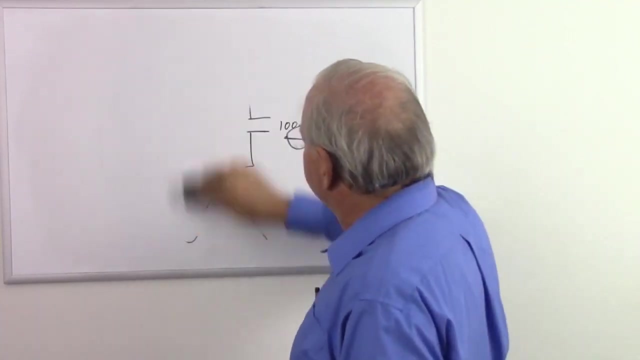 it will continue to charge. And if this starts to fall, as long as this is still higher, it'll still continue to charge, But as soon as this voltage falls below the voltage here, it'll start to discharge. Now let's take a look at a graph of that and see what the consequences are. 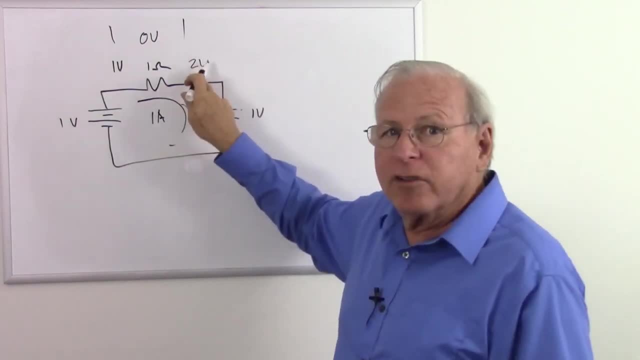 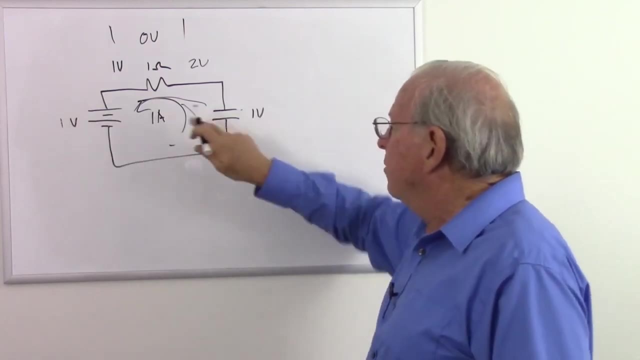 volt there. Now we have more voltage on this side than that side and it's going to push the opposite direction. So this voltage goes up. As long as this voltage is higher than that voltage, the capacitor will charge, But as soon as this voltage drops below the capacitor's voltage, it'll start discharging. 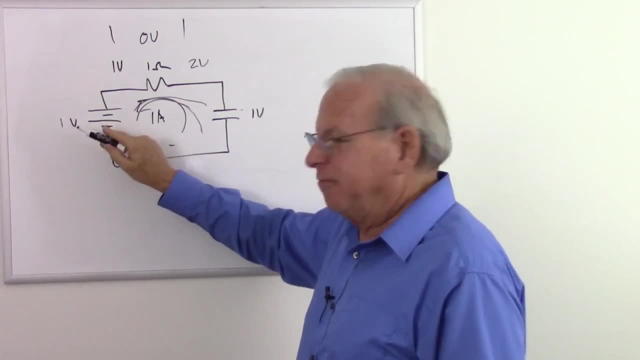 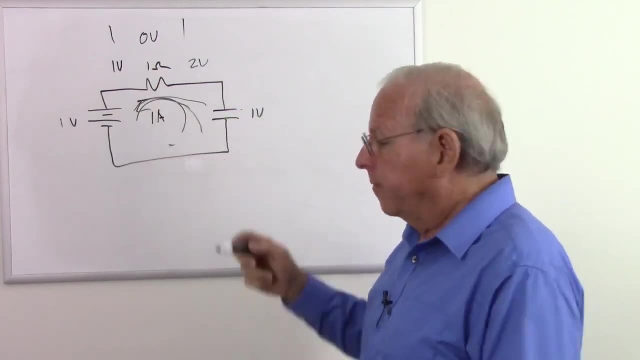 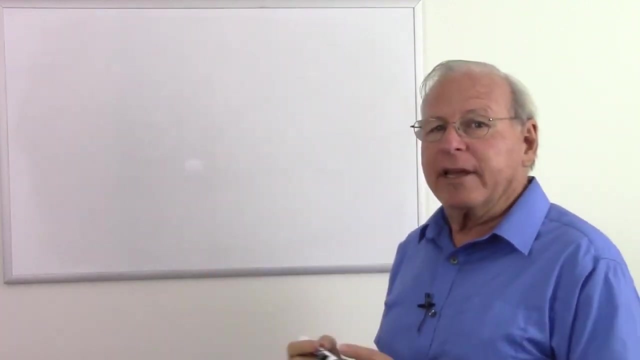 So that's basically what the AC circuit does. It's like a DC voltage, but the voltage is constantly changing, And if it changes in a periodic way, we call it alternating current. So let's take a look at how that circuit works at different moments in time and analyze why we get a phase angle. 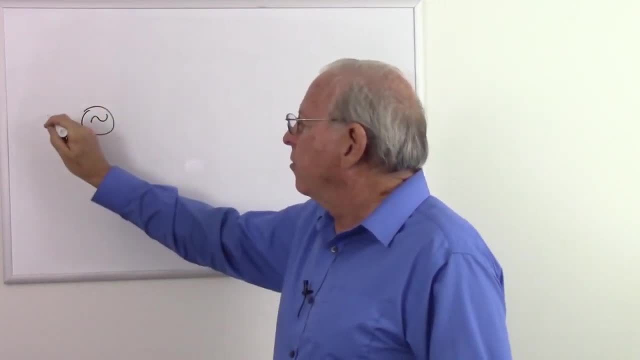 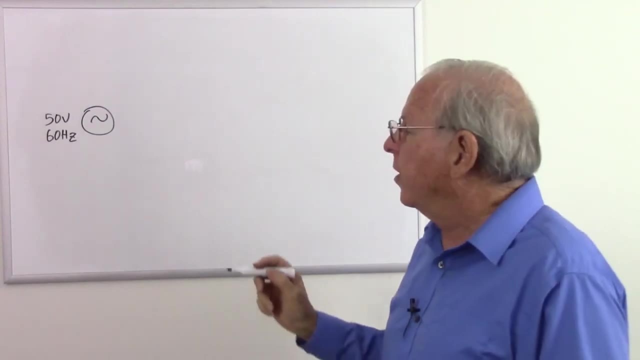 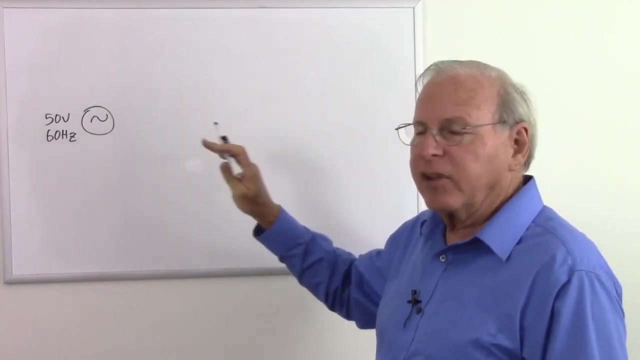 So this is the circuit I'm going to use. There's our alternating current source. I'll use 50 volts at 60 hertz, although the frequency doesn't really matter too much at this point. It matters for calculating different parameters of the circuit. but for the phase angle, what we need to know for the phase. 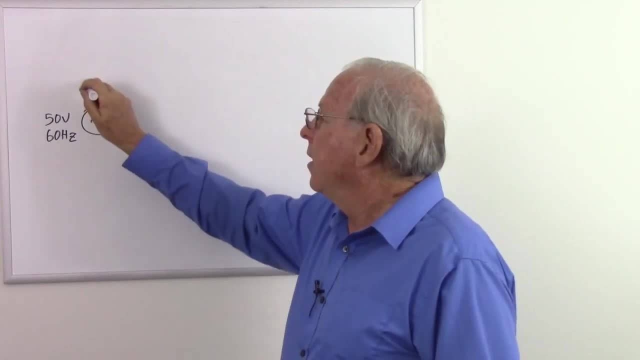 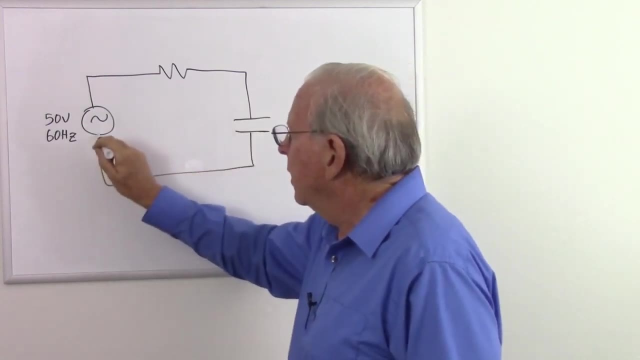 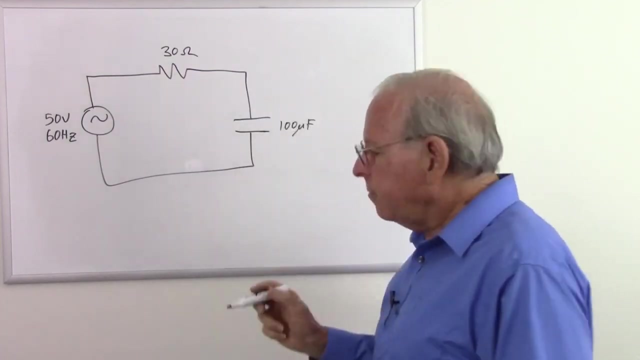 angle, it's somewhat inconsequential. So now I'm going to put a resistor here and a capacitor. I'm going to make this 30 ohms and 100 microfarads. So what's going to happen with this circuit? Well, of course, this voltage. 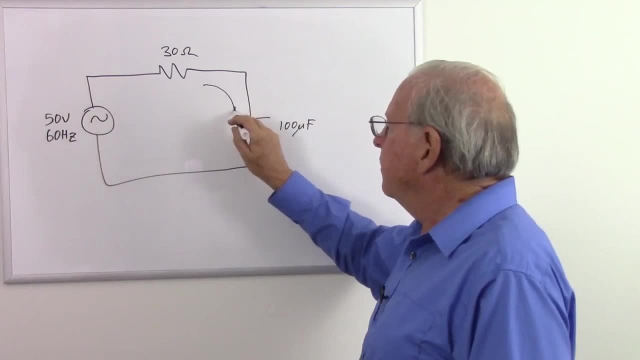 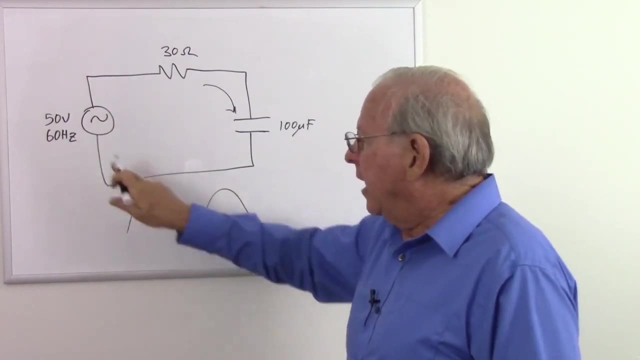 is going to go up and this capacitor is going to start charging and it's going to try to charge toward whatever voltage. this is, Remember what's happening. That voltage is going up and down and up and down and it says 50 volts, but that's the RMS voltage. It actually peaks at about 70 volts. 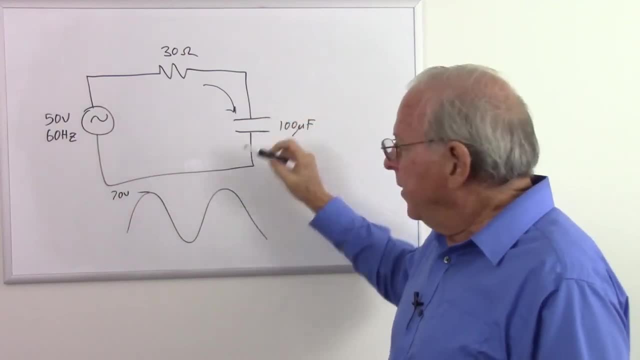 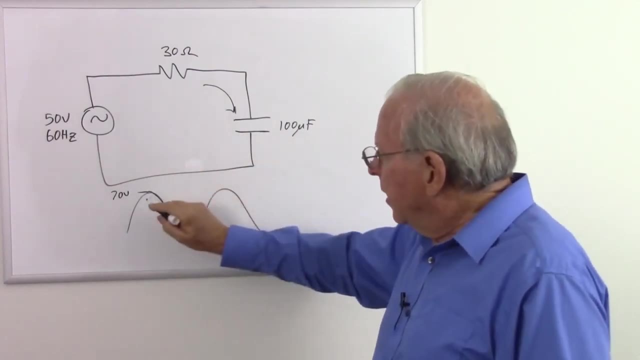 So that keeps going up and up, and as that's going up and up, this is charging And then eventually that's going to drop. As long as this has not caught up, it will continue to charge, And if this starts to fall, as long as this is still higher, it'll still continue to charge. 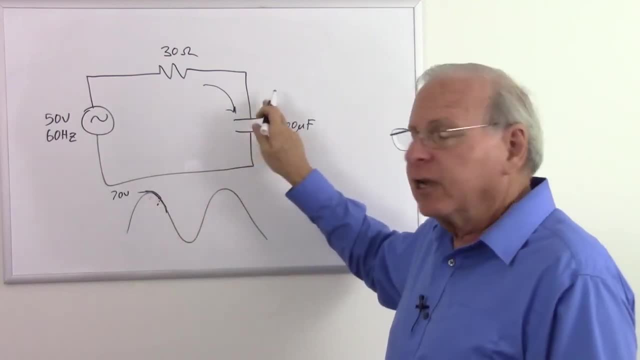 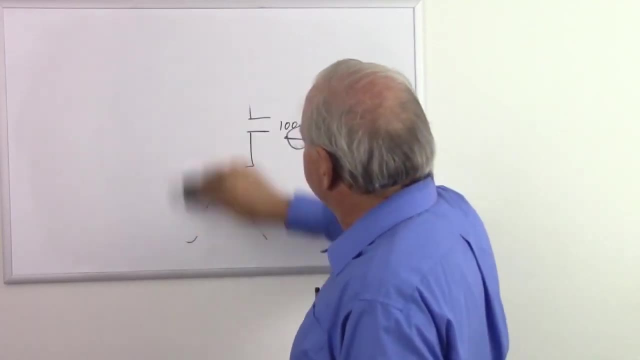 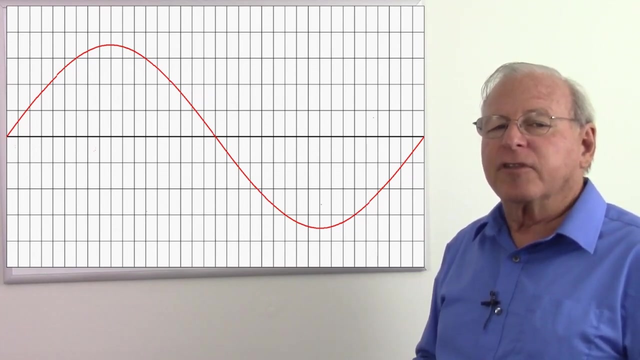 But as soon as this voltage falls below the voltage here, it'll start to discharge. Now let's take a look at a graph of that and see what the consequences are. So here I have a graph of a sine wave and it shows 360 degrees, or one cycle of the sine wave. 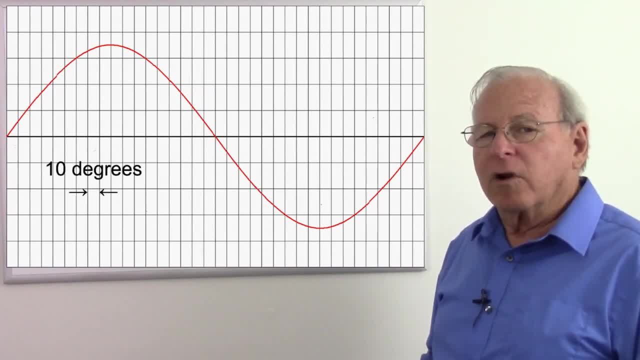 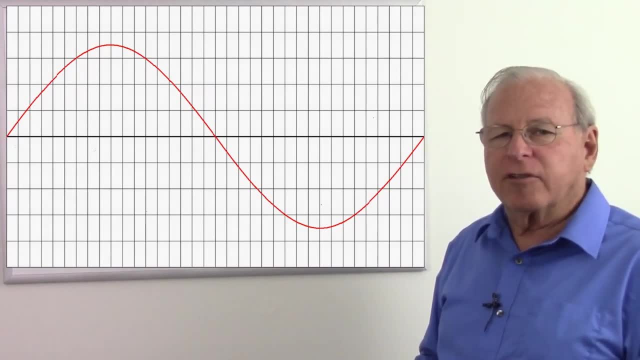 of the vertical lines is 10 degrees. The horizontal lines represent voltage. Each horizontal line is 20 volts. So we have this 50 volt sine wave which actually peaks at about 70 volts and then goes to zero, then peaks at again at a minus 70 volts, making our complete cycle And once again it's 360. 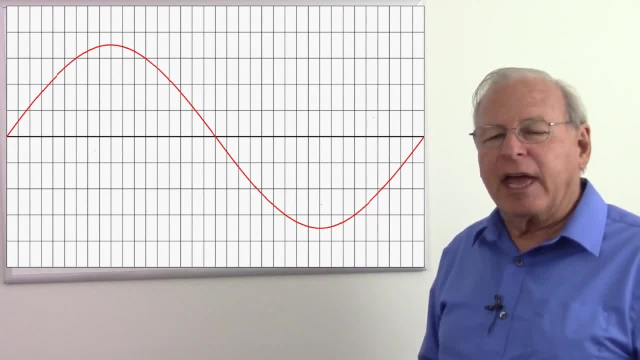 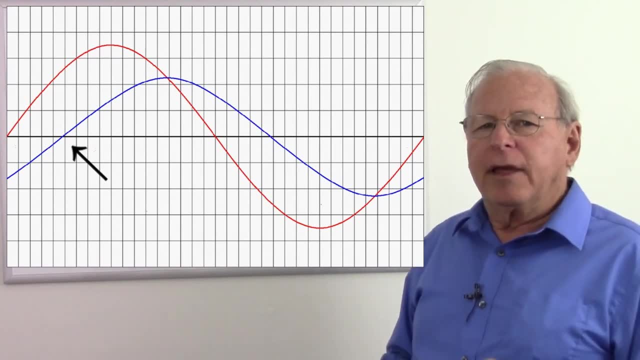 degrees across. Now let's look at what happens as that capacitor charges. Let's pick it up right here, where the voltage crosses zero on its way up. Now the source voltage is higher than the capacitor voltage, so the capacitor is going to charge and it's going to keep charging, but the capacitor 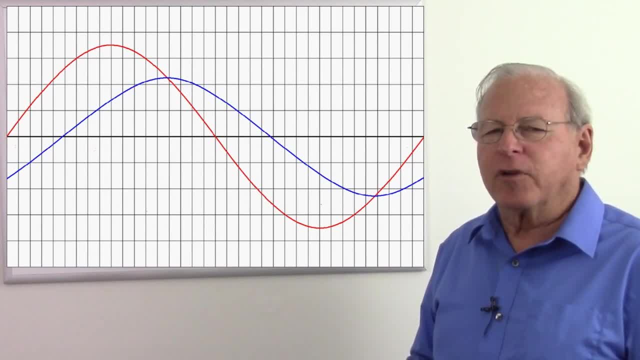 voltage can't catch up to the source voltage because the source voltage keeps going up And, look it even kind of charges in a straight line here instead of heeling over. But right here the source voltage peaks and starts to drop, But as long as it is higher than the capacitor voltage. 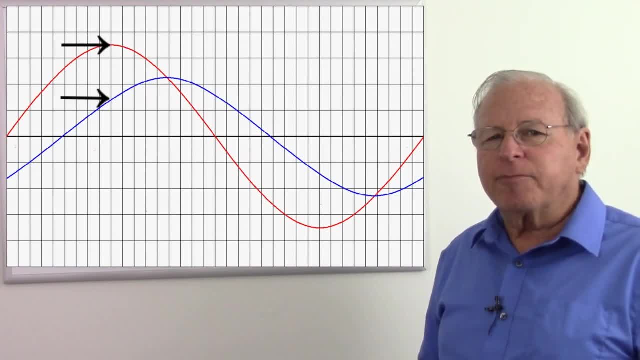 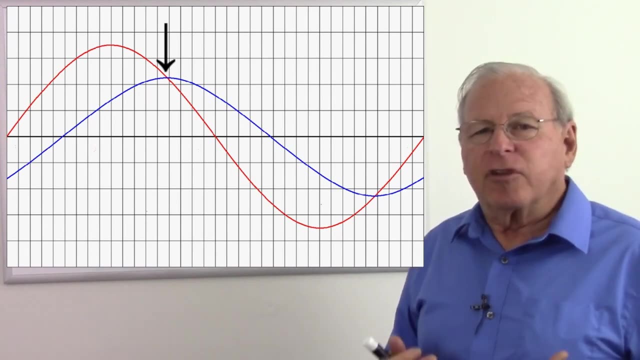 the capacitor continues to charge, but it's not charging as fast because the voltage is coming down. so the capacitor voltage starts to heel over. And then, right here, the source voltage has come down and now meets the capacitor voltage. Now, what must happen at this point? Well, once the source voltage goes below the capacitor voltage, the capacitor must start. 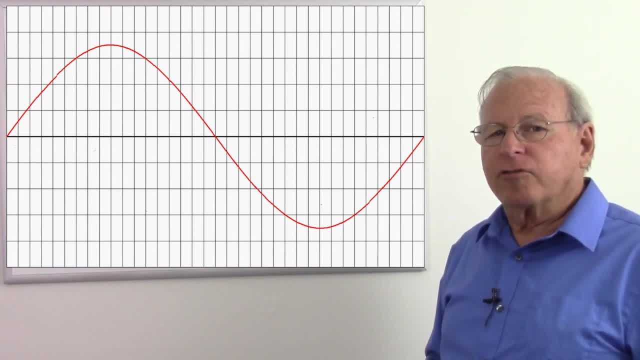 So here I have a graph of a sine wave and it shows 360 degrees, or one cycle of the sine wave, and each one of the vertical lines is 10 degrees. The horizontal lines represent voltage. Each horizontal line is 20 volts. So we have this 50 volt sine wave, which actually peaks at about 70. 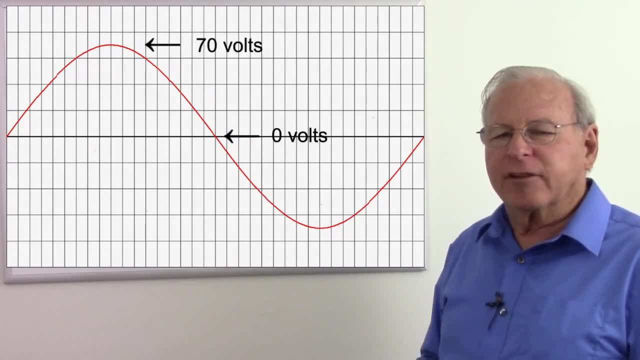 volts and then goes to zero, then peaks at again at a minus 70 volts, making our complete cycle, And once again it's 360 degrees across. Now let's look at what happens as that capacitor charges. Let's pick it up right here, where the voltage crosses zero on its way up. 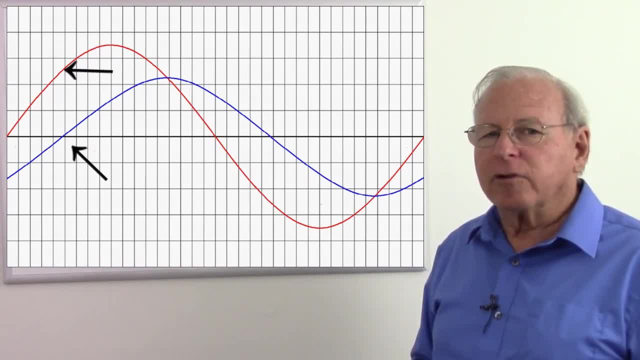 Now the source voltage is higher than the capacitor voltage, so the capacitor is going to charge and it's going to keep charging, But the capacitor voltage can't catch up to the source voltage. because the source voltage keeps going up And, look it, even kind of charges in a straight. 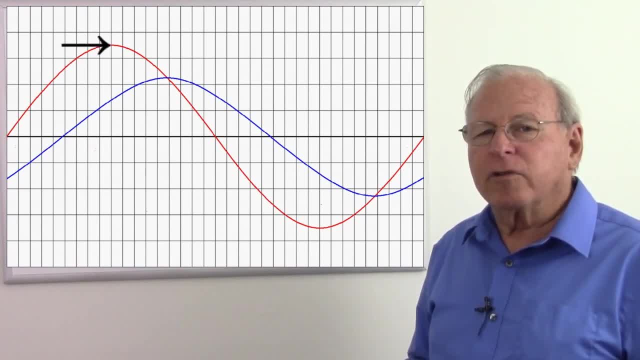 line here instead of heeling over. But right here the source voltage peaks and starts to drop. But as long as it is higher than the capacitor voltage, the capacitor continues to charge, but it's not charging as fast because the voltage is coming down, so the capacitor voltage starts. 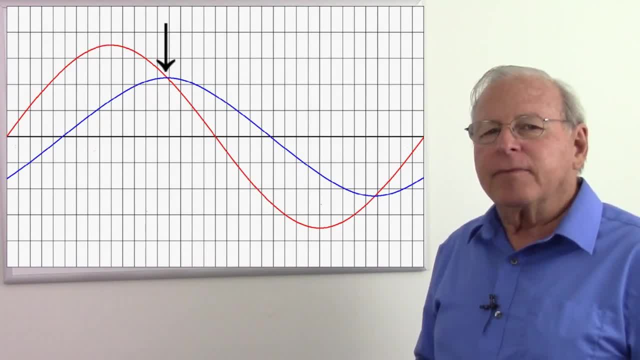 to heel over. And then, right here, the source voltage has come down and now meets the capacitor voltage. Now, what must happen at this point? Well, once the source voltage goes below the capacitor voltage, the capacitor must start discharging. So here we see, the capacitor voltage peaking. 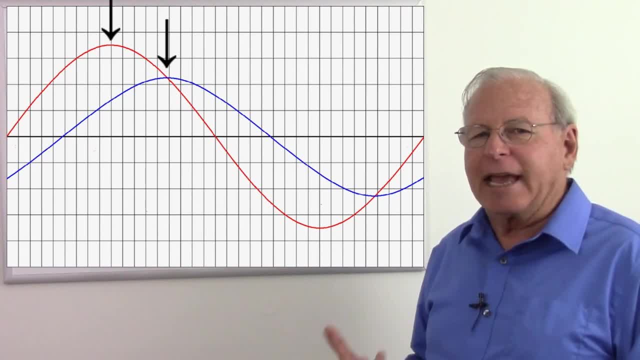 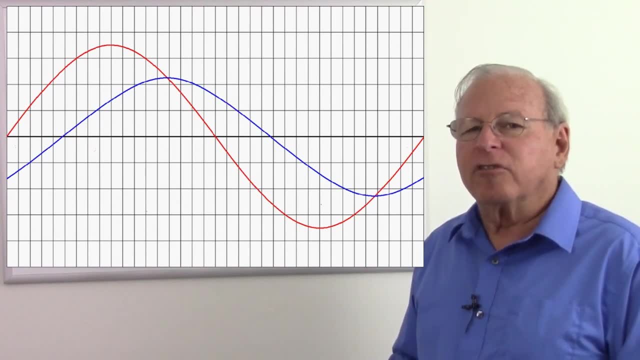 sometime after the source voltage peak because it's lagging behind and it's charging. But as soon as the source voltage crosses the capacitor voltage, the capacitor starts to discharge. So the capacitor voltage must peak where it crosses the source voltage, because that's where they become equal. And if we look at the graph, we see this is happening when the battery. 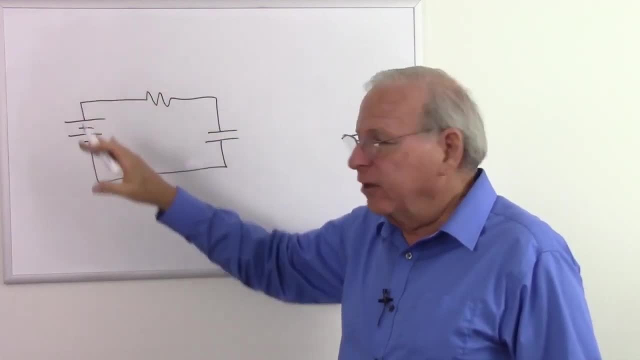 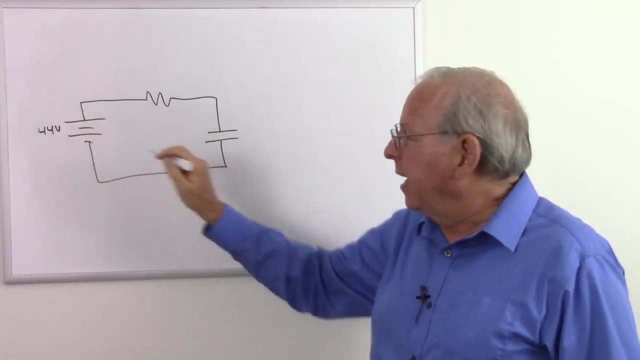 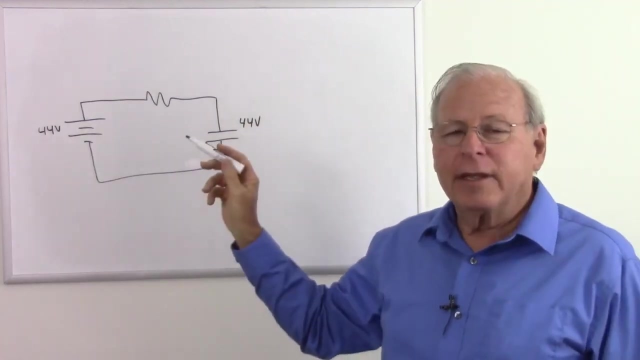 voltage. remember: the battery voltage is going up and down. it's really an AC source here, And so when this reaches at about 44 volts, it's dropping down. This is going up, but they meet when this reaches 44 volts, So at the point that the capacitor 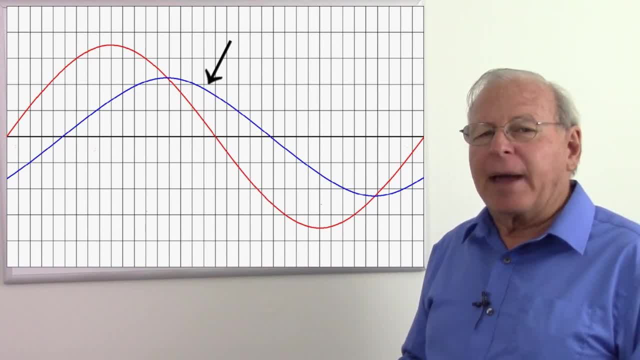 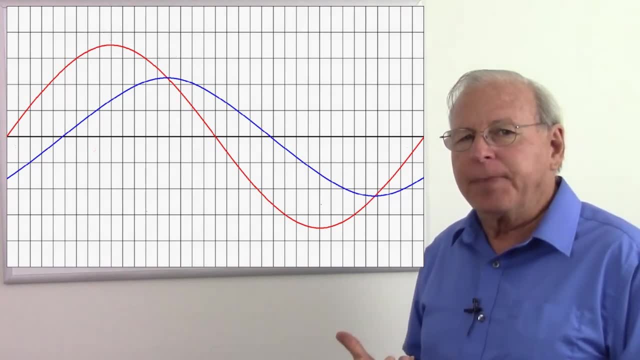 discharging. So here we see the capacitor voltage peaking sometime after the source voltage peak because it's lagging behind and it's charging. But as soon as the source voltage crosses the capacitor voltage, the capacitor starts to discharge. So the capacitor voltage must peak where it crosses the source voltage, because that's. 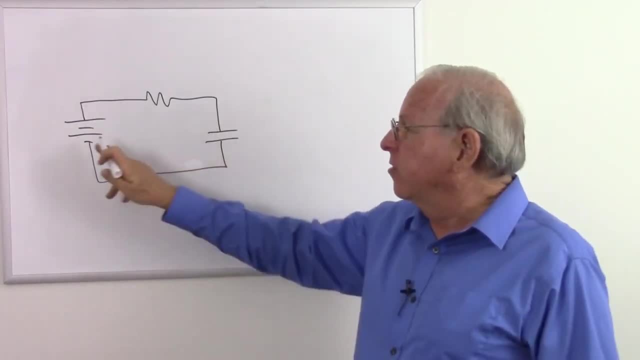 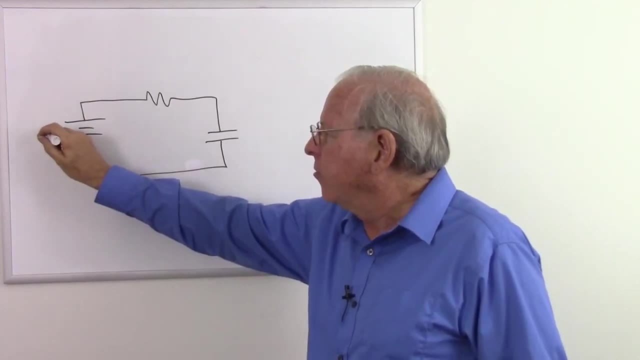 where they become equal. And if we look at the graph, we see this is happening when the battery voltage- remember the battery voltage- is going up and down. it's really an AC source here, And so when this reaches at about 44 volts it's dropping down. this is going up, but they meet. 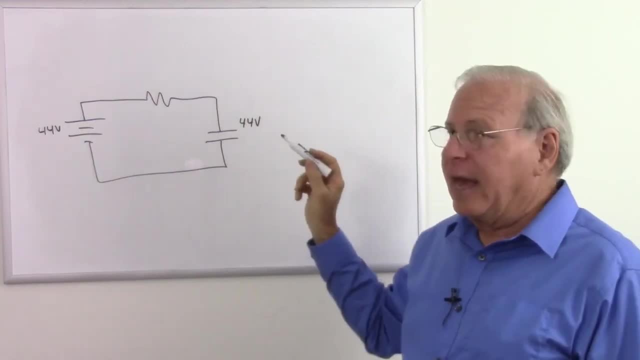 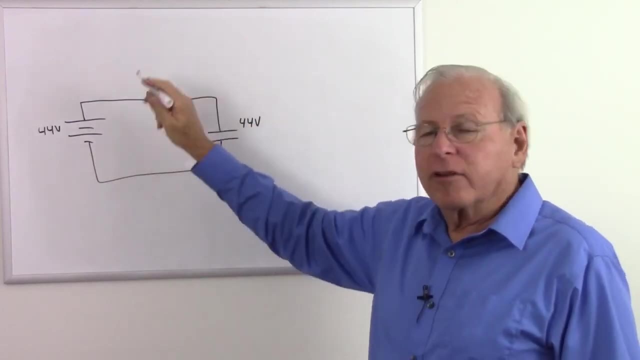 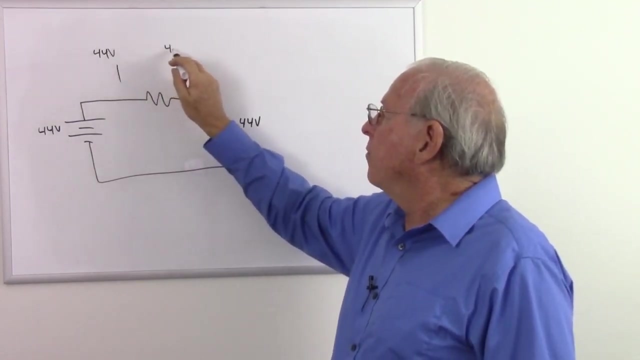 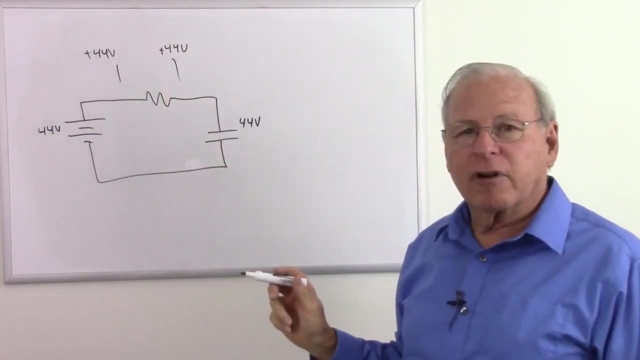 at 44 volts. So at the point that the capacitor voltage and the source voltage meet, how much voltage is across the resistor? We have 44 volts on this side, 44 volts on that side. In this case they're positive, but if it was negative it would be the same thing. How much voltage is across the? 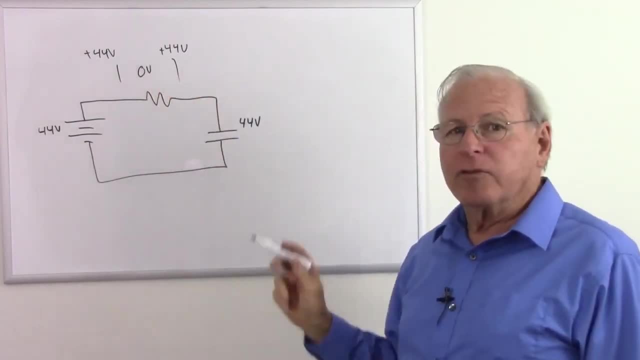 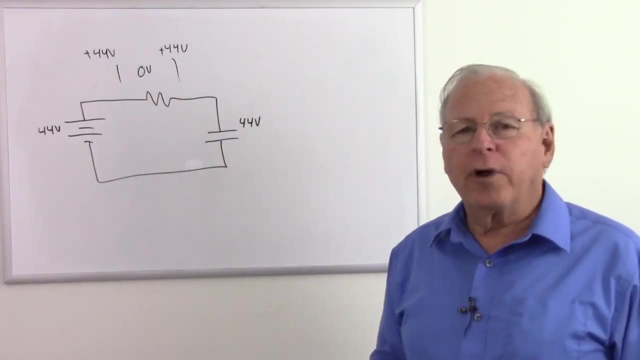 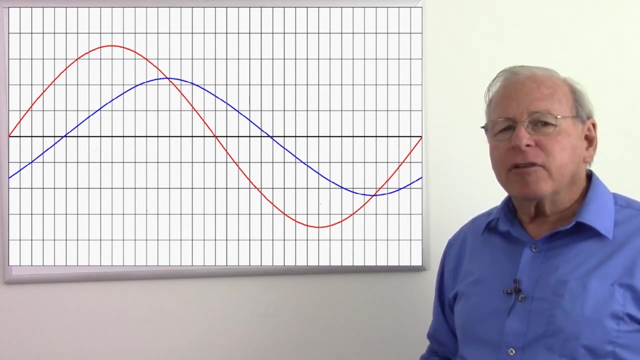 resistor Zero volts. So with zero volts across the resistor, how much voltage is across the resistor? Current is flowing, Zero amps. So two things are happening. at this point in the graph We see that the capacitor voltage must peak where it crosses the source voltage. Now this is going. 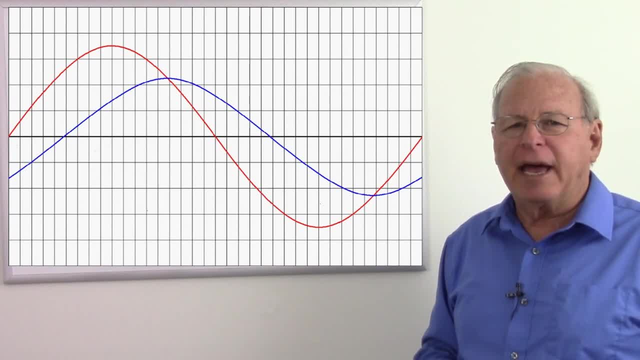 to happen at a different time depending on your combination of resistor and capacitor. If you have more resistance or more capacitance, it's going to take longer for the capacitor to charge, so this is going to happen later. If you have less resistance or less capacitance. 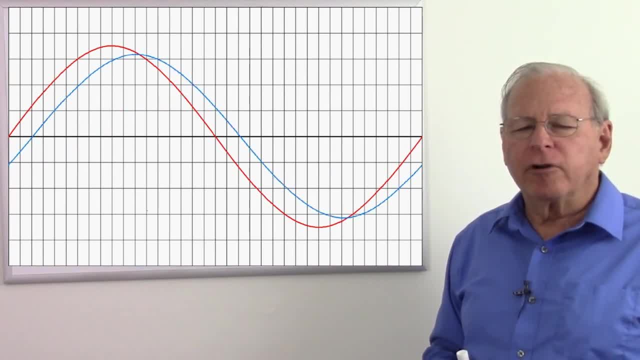 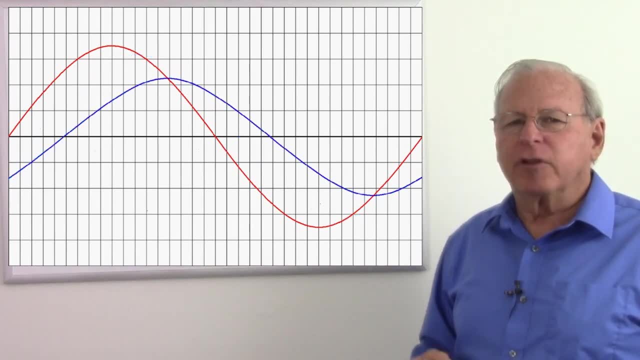 the capacitor is going to charge faster and so it's going to happen sooner. But the voltage will peak where it crosses the source voltage. It has to, because when the source voltage is higher it's charging, when the source voltage is lower, it's discharging. 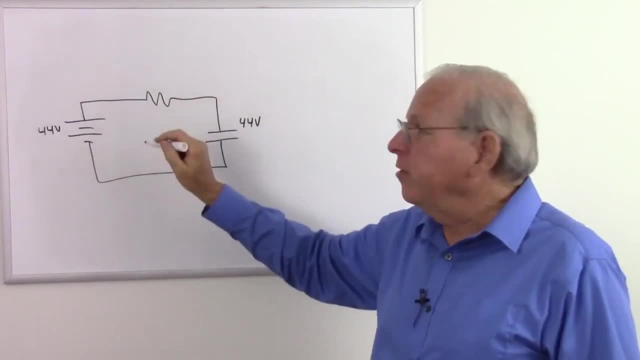 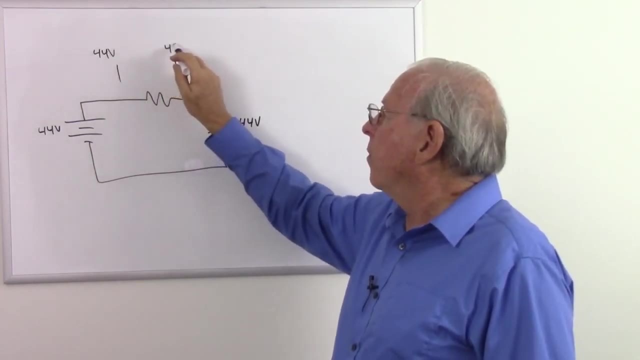 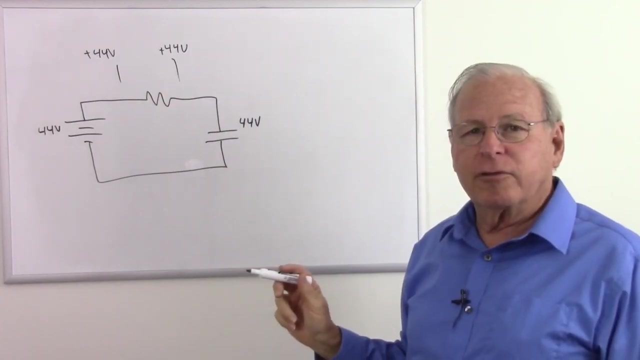 voltage and the source voltage meet. how much voltage is across the resistor? We have 44 volts on this side, 44 volts on that side. In this case they're positive, but if it was negative it would be the same thing. How much voltage is across the resistor? Zero volts. 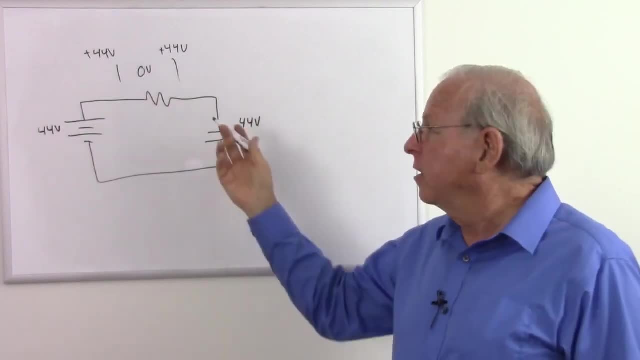 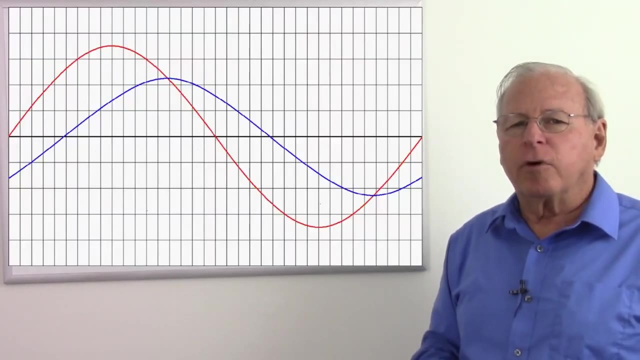 So with zero volts across the resistor, how much current is flowing? Zero amps. So two things are happening. at this point in the graph We see that the capacitor voltage must peak where it crosses the source voltage. Now this is going to happen at a. 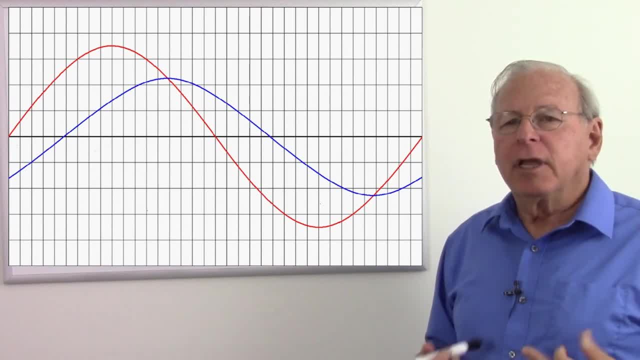 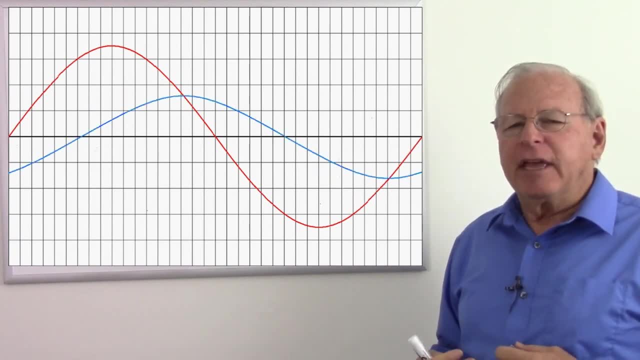 different time depending on your combination of resistor and capacitor. If you have more resistance or more capacitance, it's going to take longer for the capacitor to charge, so this is going to happen later. If you have less resistance or less capacitance, the capacitor is. 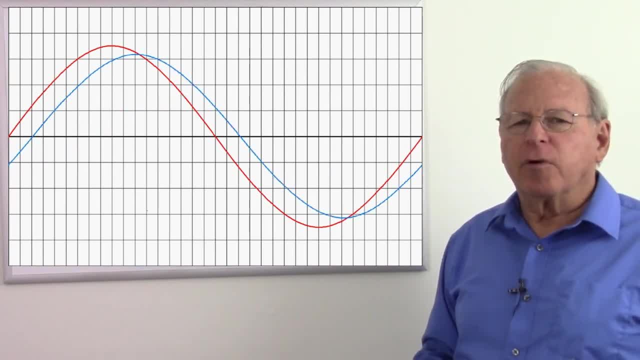 going to charge faster, and so it's going to happen sooner. But the voltage will peak where it crosses the source voltage. It has to, because when the source voltage is higher, it's charging, When the source voltage is lower, it's discharging, and so that's the point where that changes. So 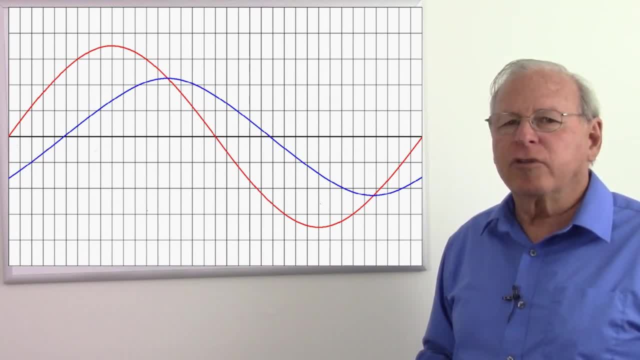 your capacitor voltage will always peak when it crosses the source voltage. This is the primary factor that determines the phase angle, but it's not the phase angle. This is the phase lag of the capacitor voltage, And again we see that at that point there's going to be zero volts. 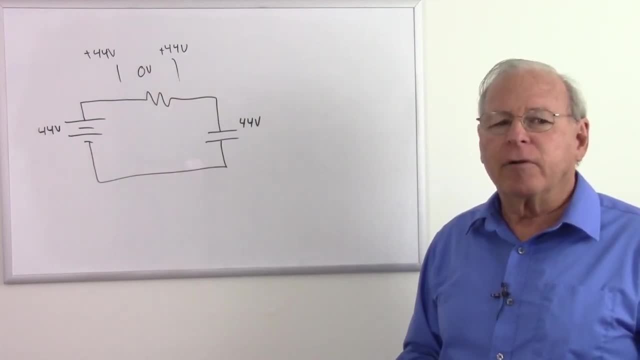 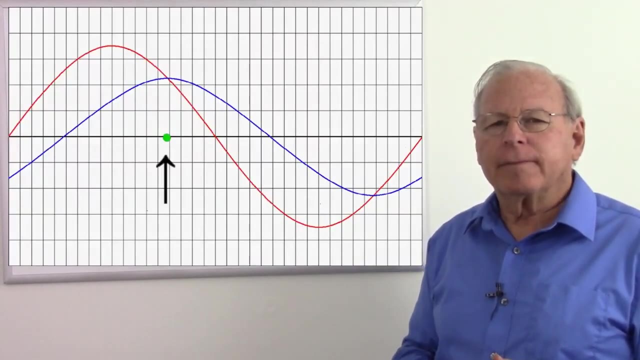 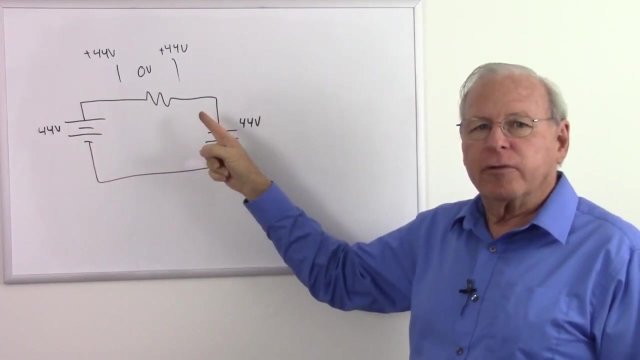 across the resistor. So how much current do we have in the circuit? Zero. So at the point that these two voltages are equal, we have zero amps of current. And that was just like the DC circuit. When the capacitor reached the source voltage, there was zero current flowing through. 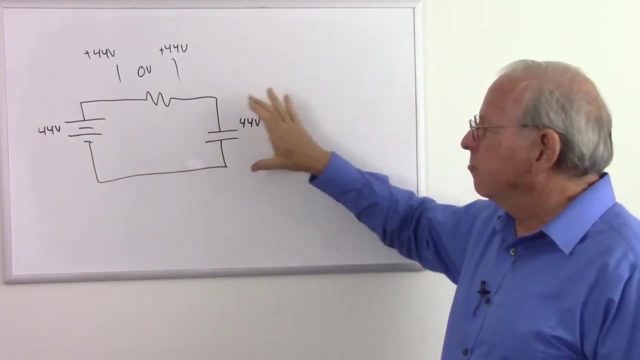 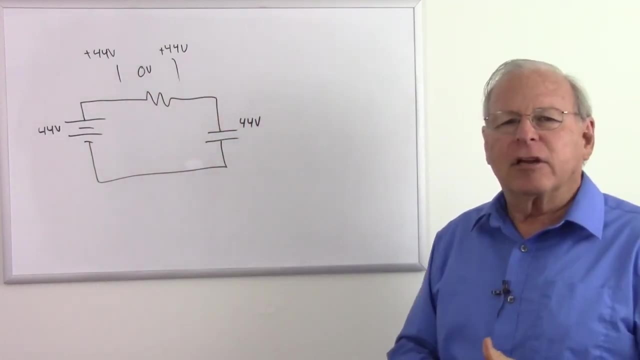 the resistor, and so we had zero current through the circuit and we had our maximum voltage across the capacitor. So, just like the DC circuit- in fact, we're looking at this as a DC circuit. Now we need to look at the next factor that leads to the 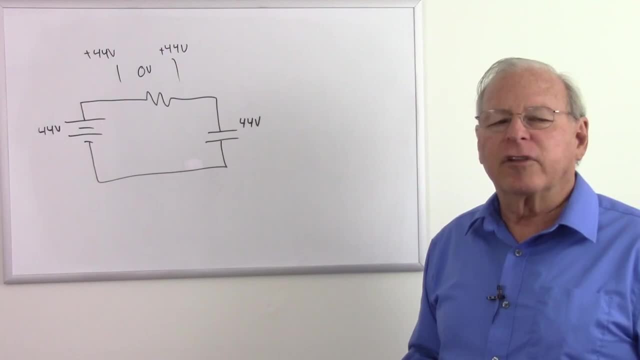 phase angle between the current and the voltage source in the circuit. So we've already seen that the current must be zero when the capacitor voltage crosses the source voltage. Now we know that the voltage across the capacitor is going to be 90 degrees out of phase with the current. 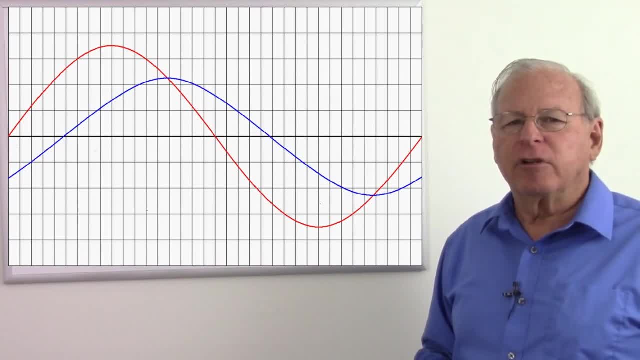 and so that's the point where that changes. So your capacitor voltage will always peak when it crosses the source voltage. This is the primary factor that determines the phase angle, but it's not the phase angle. This is the phase lag of the capacitor voltage, And again we see that at that. 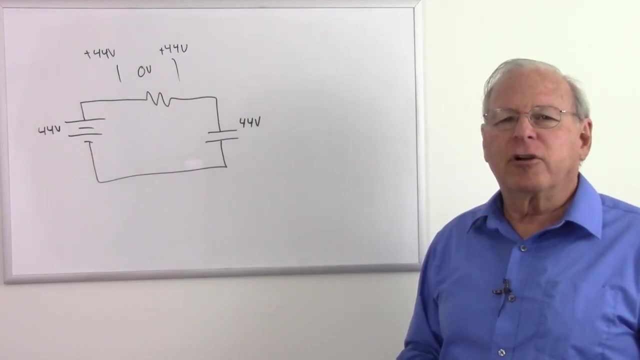 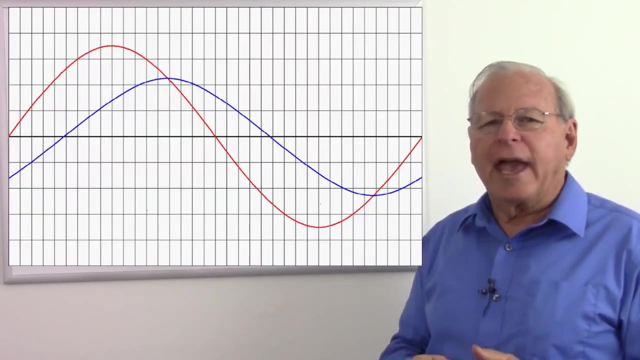 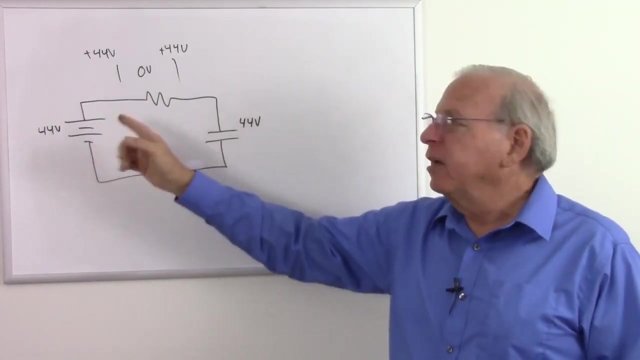 point there's going to be zero volts across the resistor. So how much current do we have in the circuit? Zero. So at the point that these two voltages are equal, we have zero amps of current. And that was just like the DC circuit. When the capacitor reached the source voltage there was 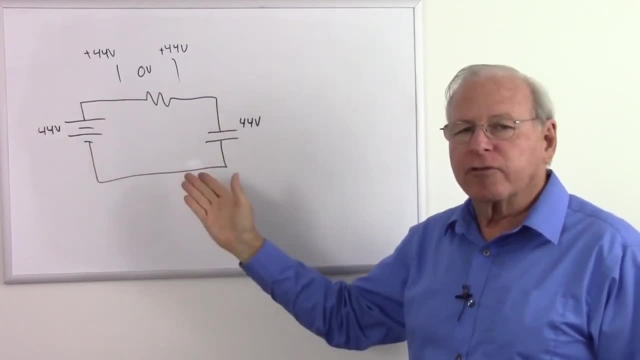 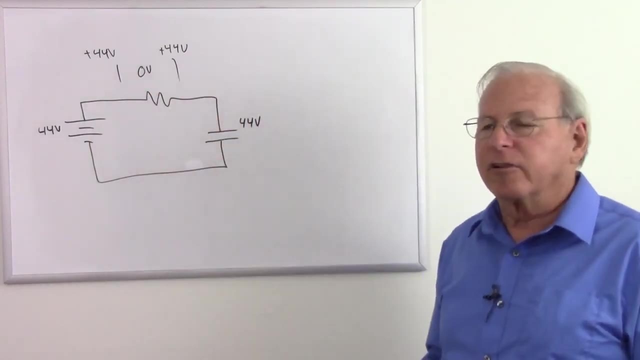 zero current flowing through the resistor, and so we had zero current through the circuit and we had our maximum voltage across the capacitor. So, just like the DC circuit- in fact, we're looking at this as a DC circuit. Now we need to look at the next factor that leads to the phase angle between the 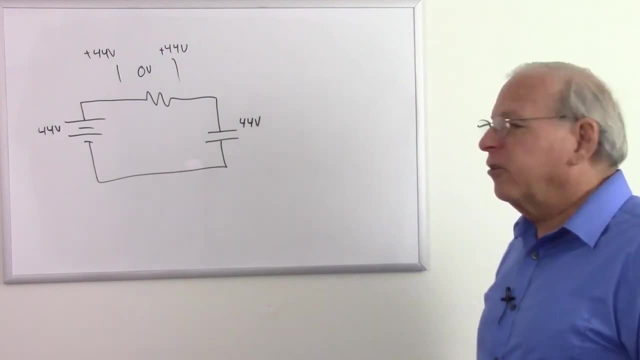 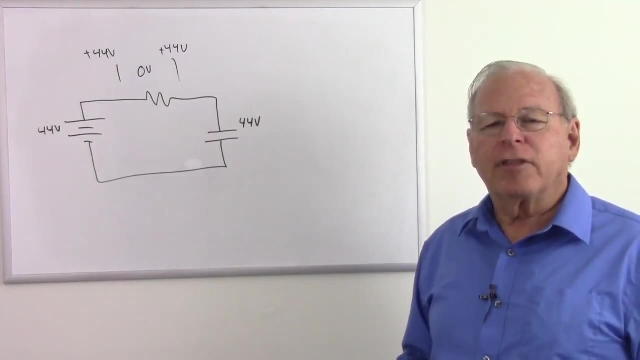 current and the capacitor voltage. This is going to be the phase angle between the current and the voltage source in the circuit. So we've already seen that the current must be zero when the capacitor voltage crosses the source voltage. Now we know that the voltage across the capacitor is 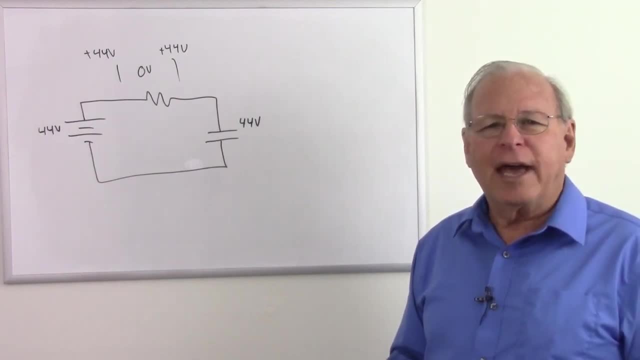 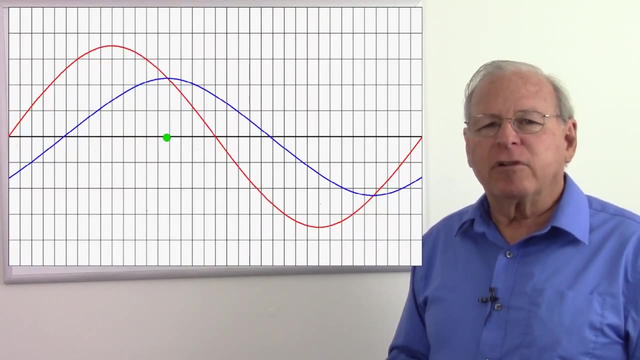 going to be 90 degrees, out of phase with the current. So why is that? Well, it has to be. First of all, we look here and we see that, just like in the DC circuit, when the capacitor voltage is at its maximum, the current must be zero. Now let's look at when the capacitor voltage is zero. So if 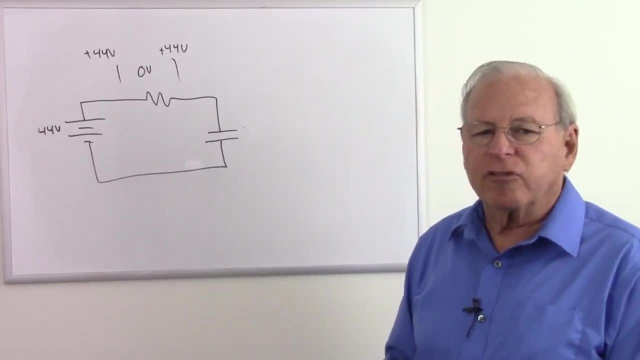 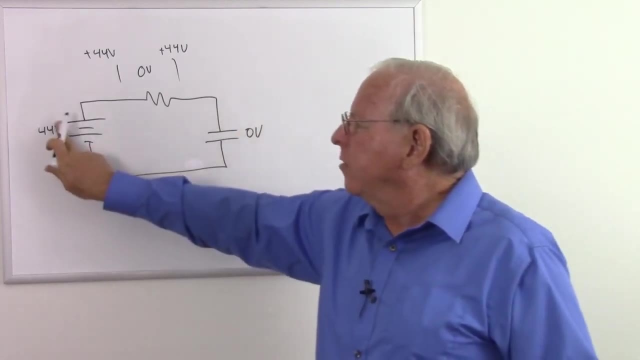 we take a look at the circuit here. this voltage is going to be 90 degrees out of phase with the current. This voltage is going to reach zero at some point And the source voltage at that point is going to be about minus 50 volts. So what do we have here? 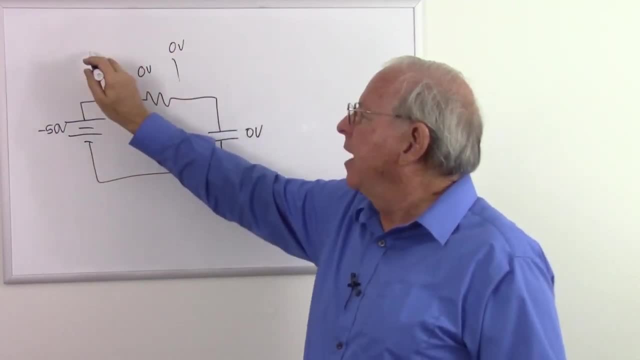 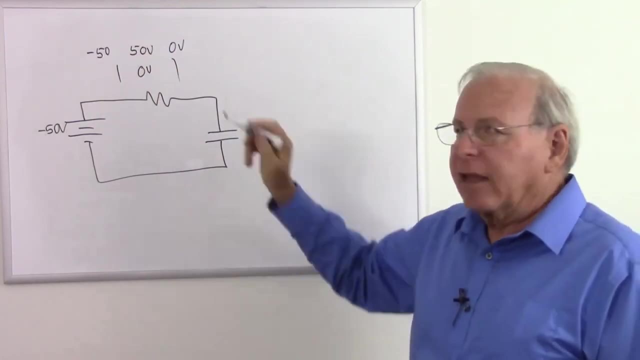 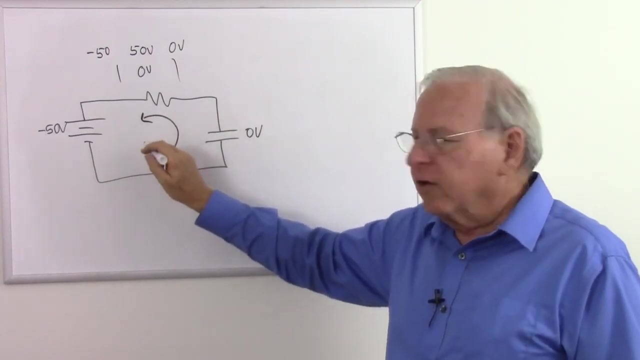 We have zero volts on that side of the resistor and approximately minus 50 volts there, So we have a 50 volt difference. That's going to give us a current going in the opposite direction now, because the capacitor is now discharging of 1.66 amps flowing in the opposite direction And that's 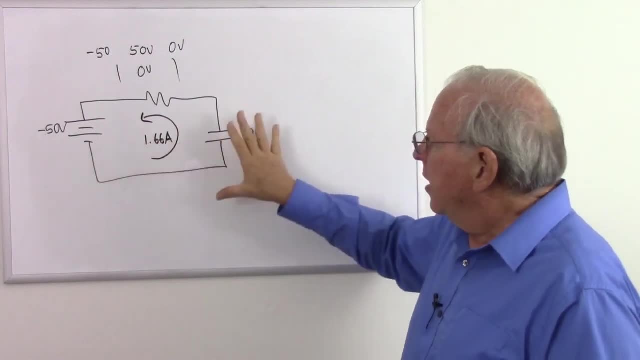 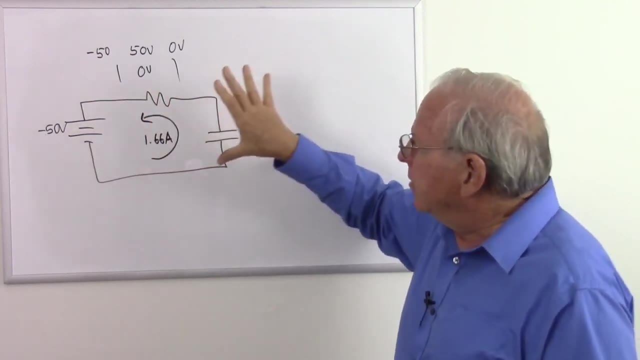 going to be our peak current, That's going to be the highest current we get, because after we pass that point, well, this is no longer zero, That's going to be going lower, And it's just the point where we get the greatest difference in voltage across that capacitor. So what have we seen so far? 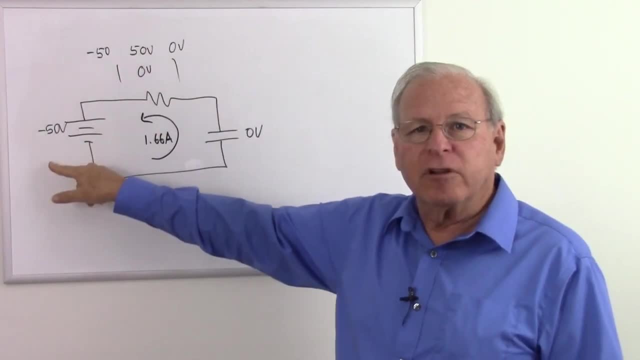 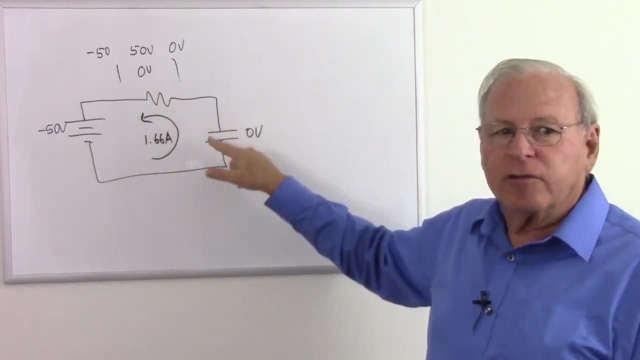 When the capacitor voltage peaks, it's going to be at the point. it's at the same voltage as the source voltage, equal on both sides of the resistor: zero current. When the capacitor voltage reaches zero, it's going to be at the point we have the greatest difference in. 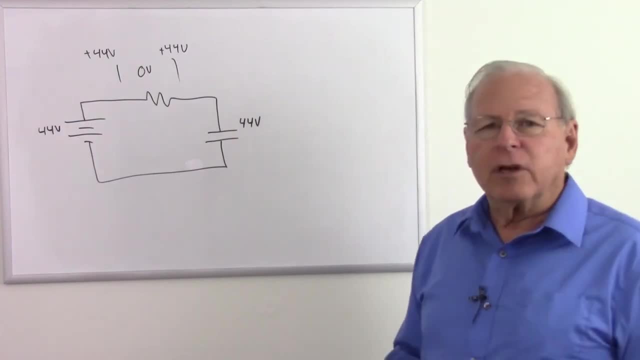 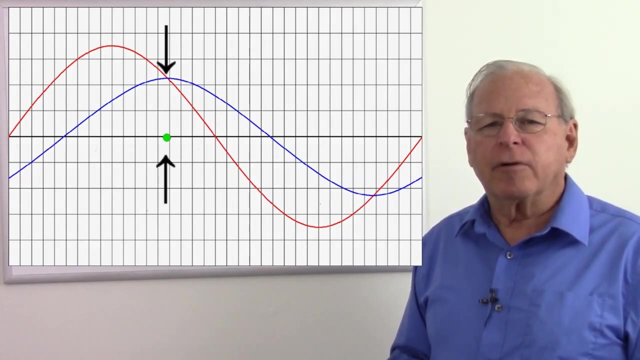 So why is that? Well, it has to be. First of all, we look here and we see that, just like in the DC circuit, when the capacitor voltage is at its maximum, the current must be zero. Now let's look at when the capacitor voltage is zero. So if we 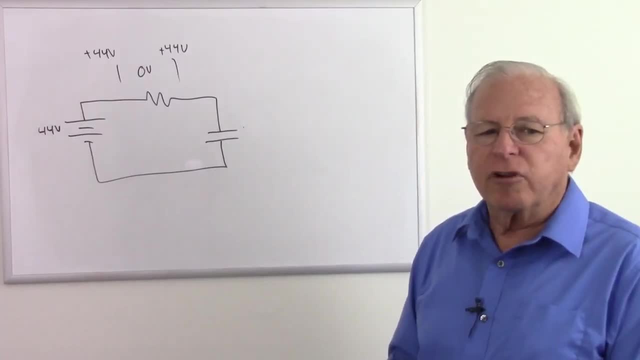 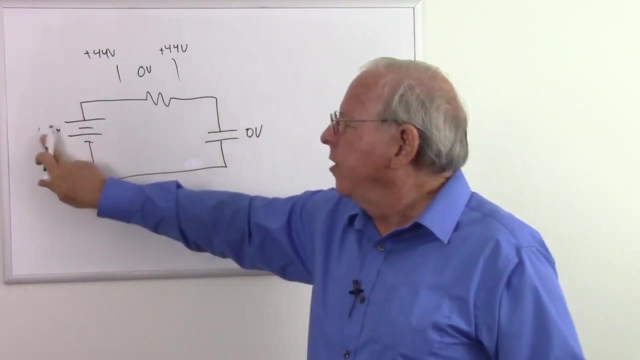 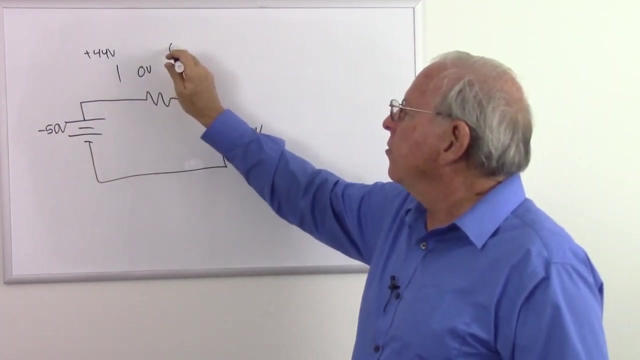 take a look at the circuit here. this voltage is going to reach zero at some point And the source voltage at that point is going to be about minus 50 volts. So what do we have here? We have zero volts on that side of the resistor and approximately. 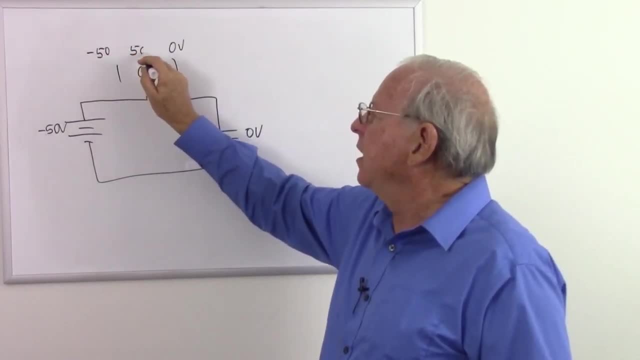 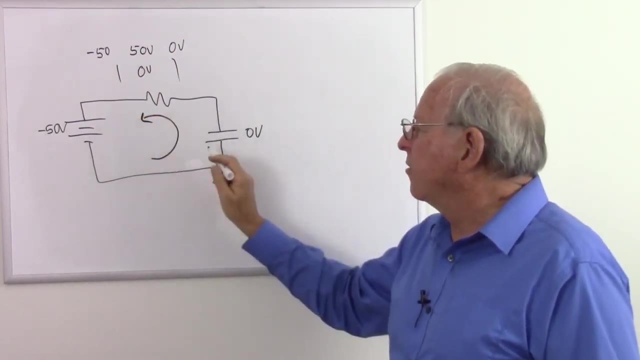 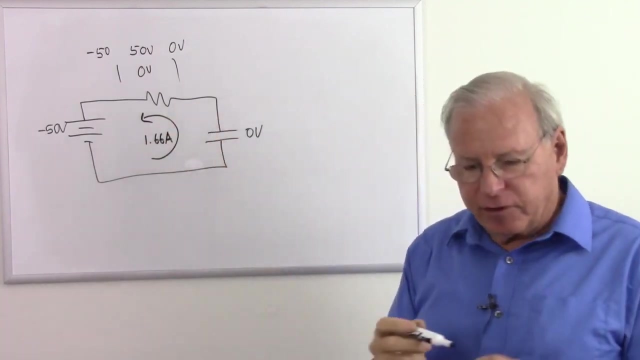 minus 50 volts there, So we have a 50 volt difference. That's going to give us a current of 1.66 amps. So we have a current of 1.66 volts flowing in the opposite direction now because the capacitor is now discharging of 1.66 amps flowing in the opposite direction And that's. 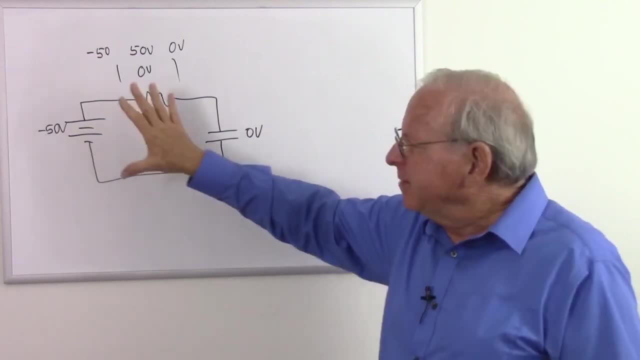 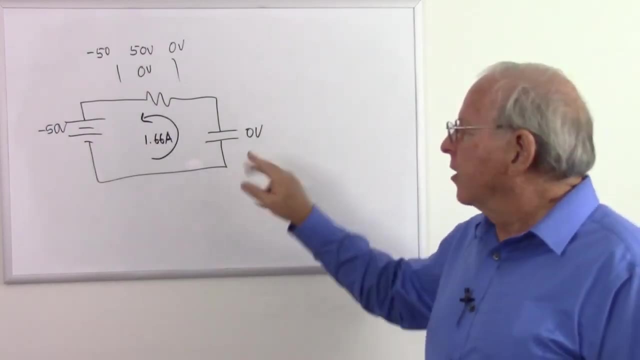 going to be our peak current, That's going to be the highest current we get, because after we pass that point, well, this is no longer zero, That's going to be going lower, And it's just the point where we get the greatest difference in voltage across that capacitor. So what have we seen so far? 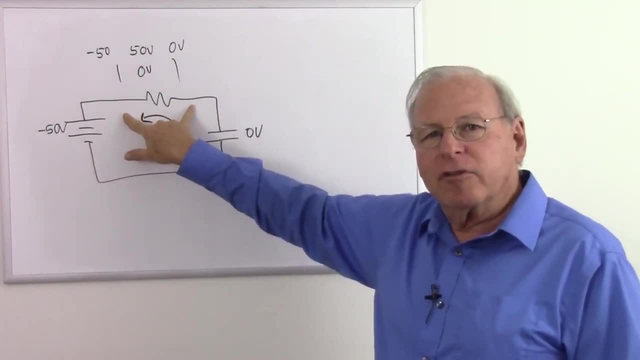 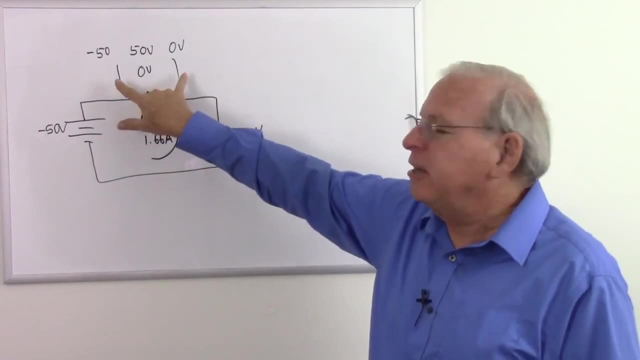 The source voltage. So the voltage is equal on both sides of the resistor: Zero current. When the capacitor voltage reaches zero, it's going to be at the point. we have the greatest difference in voltage across the resistor And there's where we get our peak current. So let me give that a 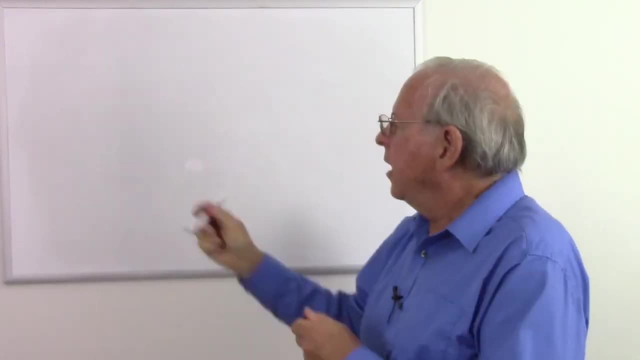 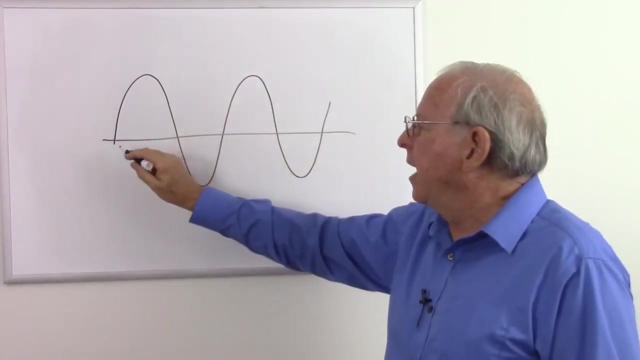 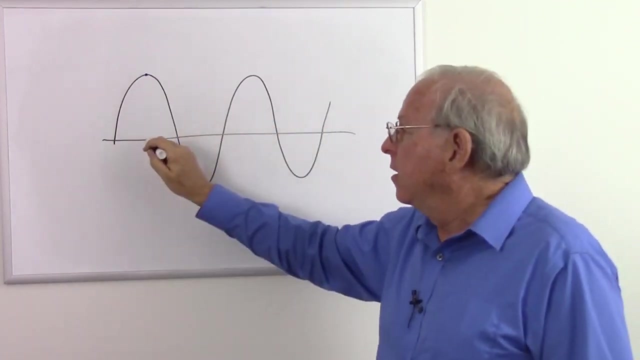 quick drawing. Here is our capacitor voltage. Let me draw a zero line here, And our current is going to be happening sometime before that. But we do know that when the capacitor voltage reaches its peak, that the current through the circuit will be zero, because at that point is. 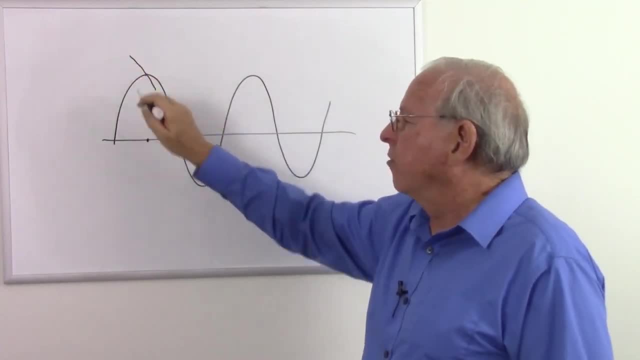 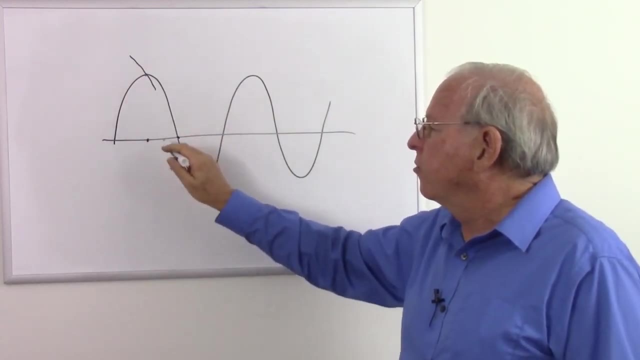 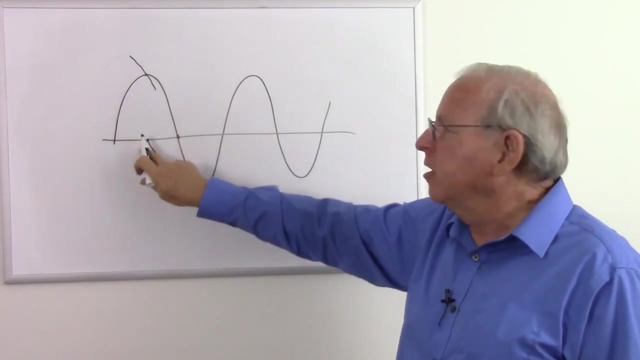 when it's crossing the source voltage. So they're equal. So we get zero amps of current. But then, when this reaches zero, we just determine that's when we're going to get our greatest current. So when the capacitor voltage peaks, we get zero amps of current. When the capacitor voltage reaches, 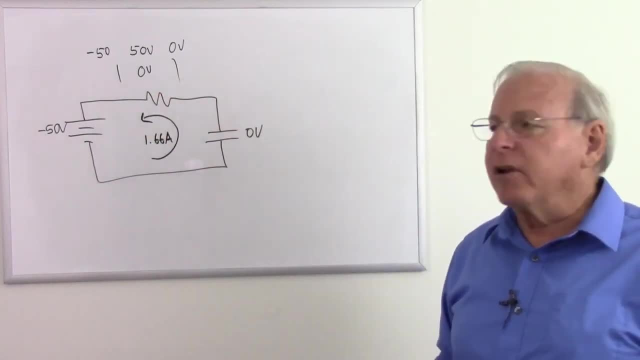 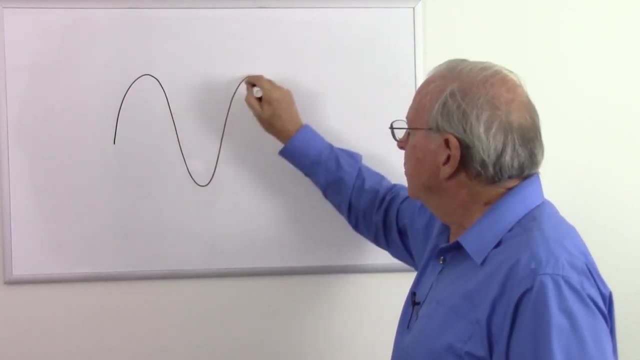 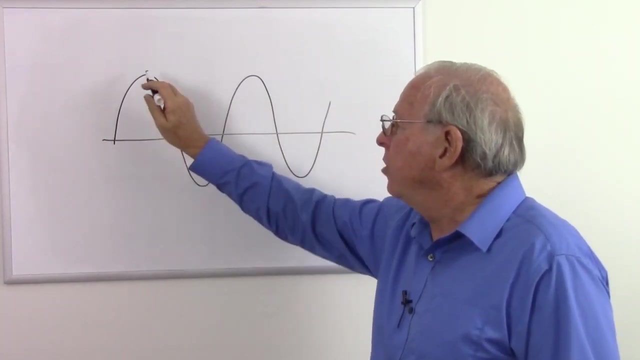 voltage across the resistor and there's where we get our peak current. So let me give that a quick drawing. Here is our capacitor voltage. Let me draw a zero line here, and our current is going to be happening sometime before that, but we do. 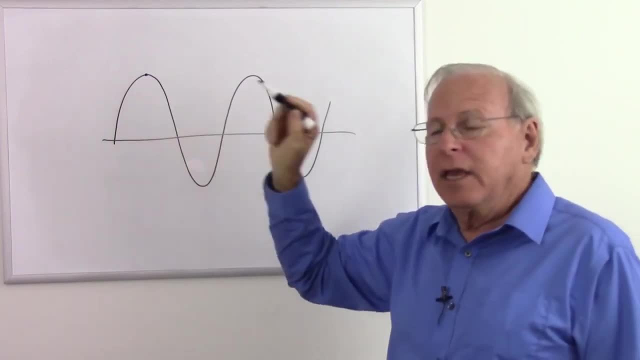 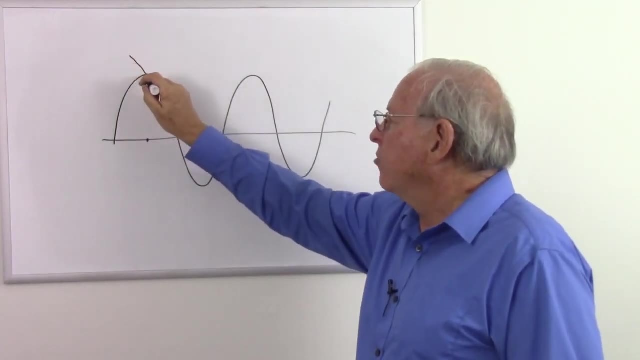 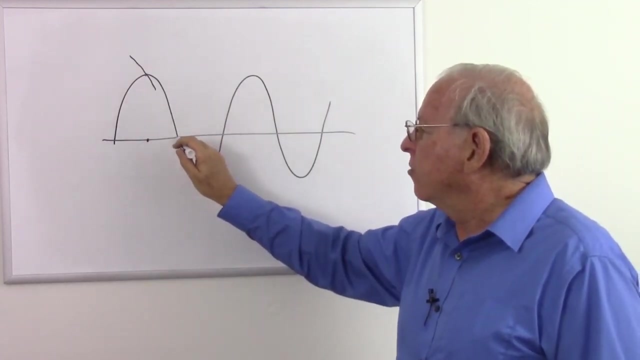 know that when the capacitor voltage reaches its peak, that the current through the circuit will be zero, because at that point is when it's crossing the source voltage. So they're equal, so we get zero amps of current. but then when this reaches zero, we just determined that's when we're going to get our 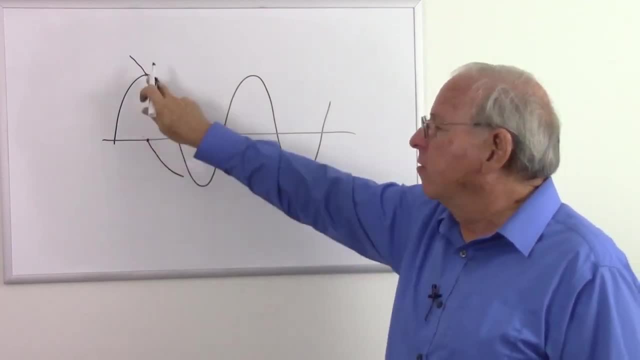 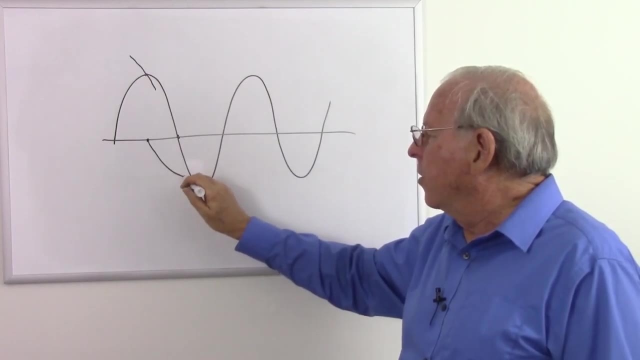 greatest current. So when the capacitor voltage peaks, we get 0 amps of current, When the capacitor voltage reaches zero, we get our maximum current, and when the capacitor voltage decreases, we get our maximum current, And then when that current comes over here and reaches zero, we already determined that. 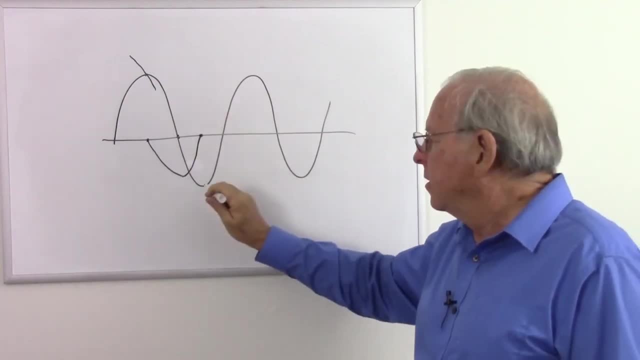 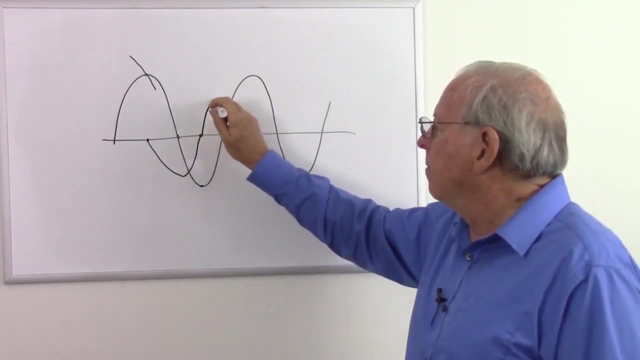 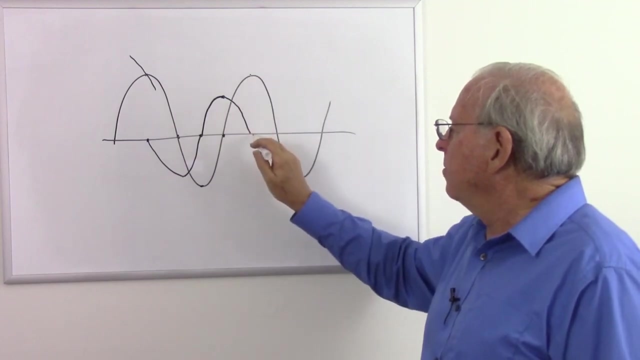 when the current is zero, we have our maximum voltage across the capacitor, And then, when that voltage reaches zero, what are we going to get? We're going to get our maximum current, And this just keeps happening over and over again: Zero, maximum, maximum, zero. 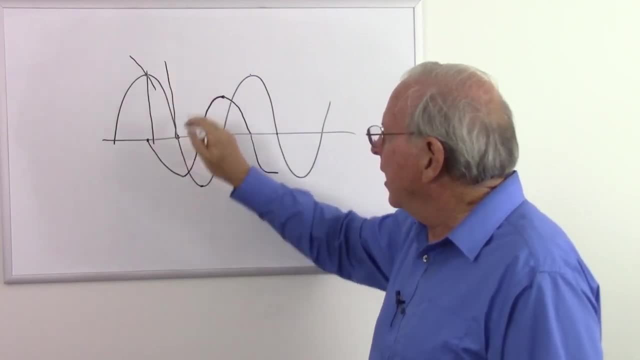 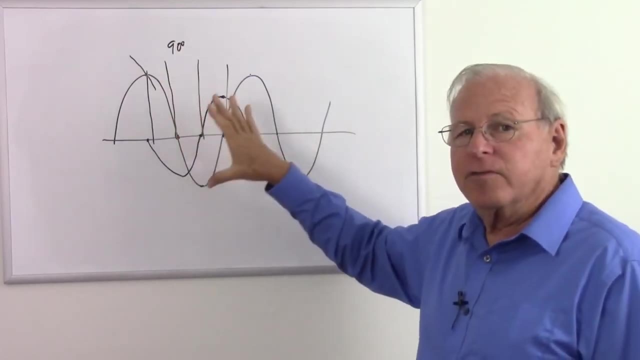 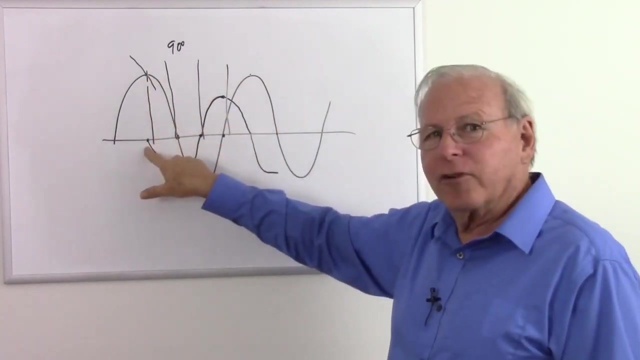 And so look where they are. Each time that happens is 90 degrees. So that's why we have that 90 degree phase difference in the voltage and current at the capacitor. because of this Capacitor voltage is maximum current through the circuit must be zero. 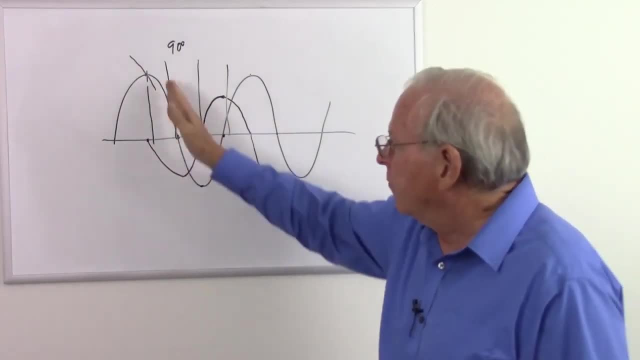 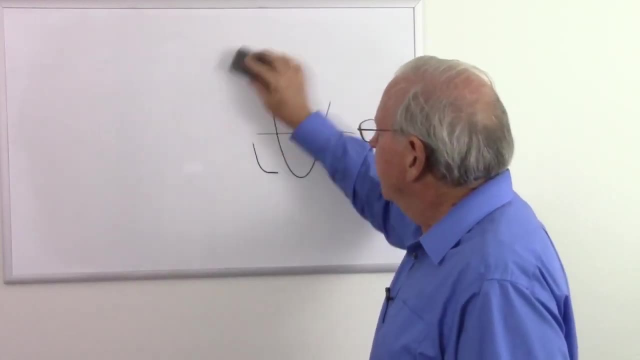 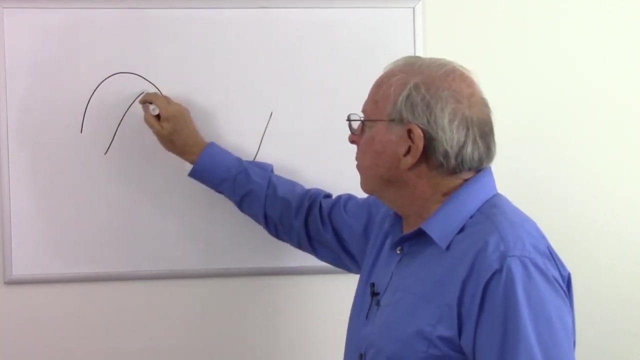 Capacitor voltage is zero, the current through the circuit must be maximum and therefore that's happening 90 degrees apart. So we're almost there. We almost know why. we have the phase angle. So we have the source voltage and then the capacitor voltage. 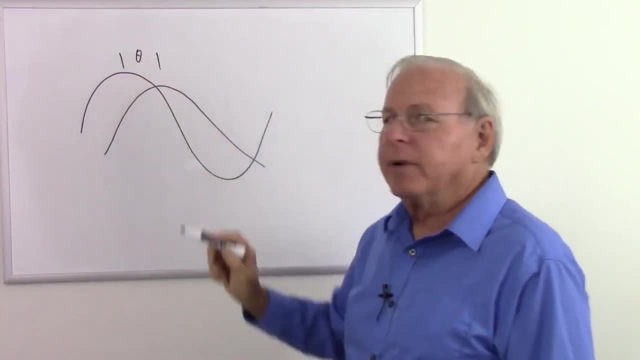 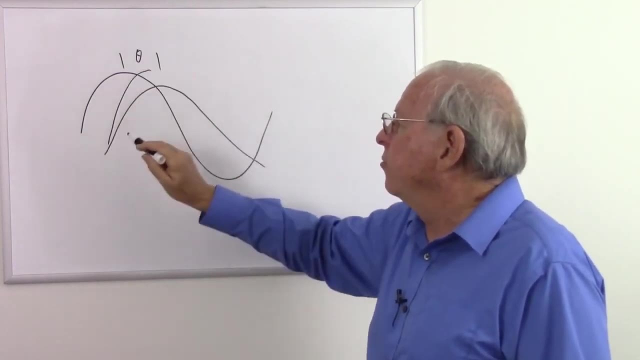 And these happen some angle which we haven't determined yet And that changes depending on the resistor and capacitor combination. So less resistance or less capacitance happens sooner. More resistance or more capacitance it happens later. So that's what determines this. 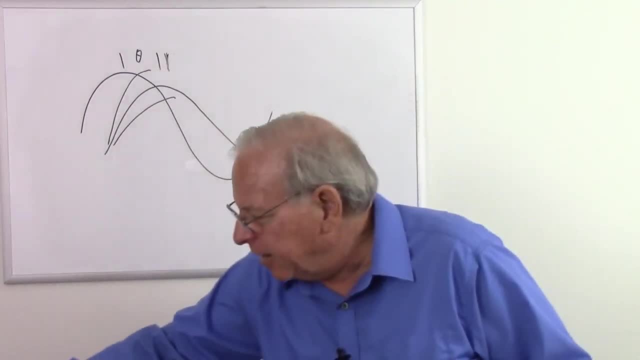 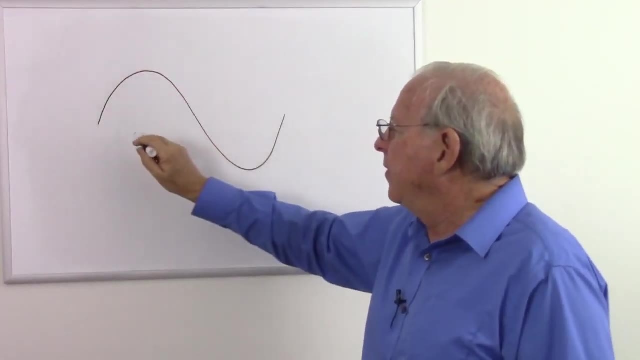 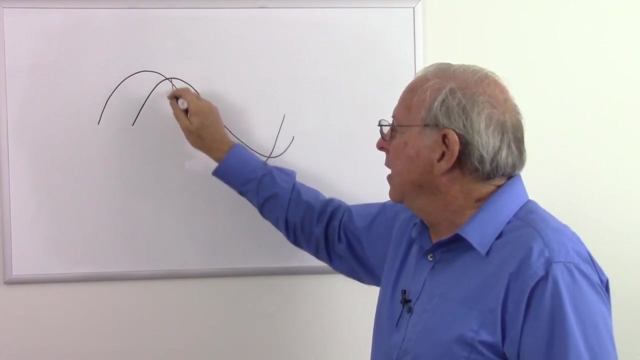 And this ultimately determines the phase angle. But if I redraw this, Okay, Okay, Okay, We once again have our source voltage and then our capacitor voltage, But now we know that the current through the circuit is going to be 90 degrees before that. 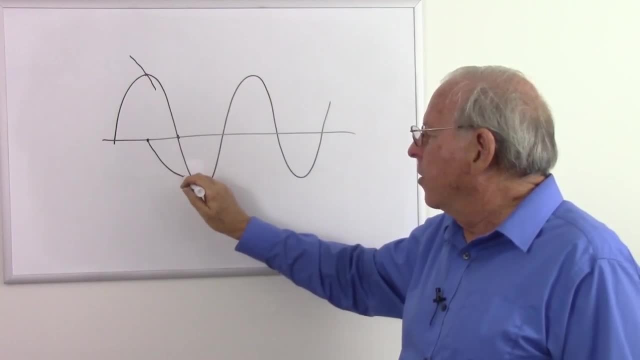 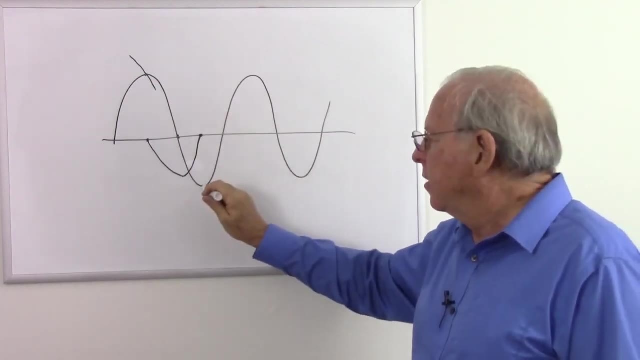 zero, we get our maximum current And then, when that current reaches zero, we get our maximum current When it comes over here and reaches zero. we already determined that when the current is zero, we have our maximum voltage across the capacitor And then, when that voltage reaches zero, 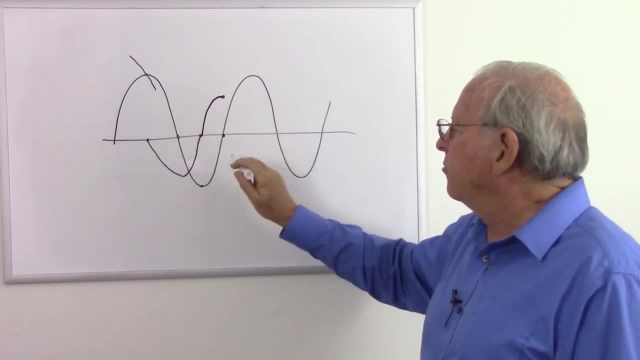 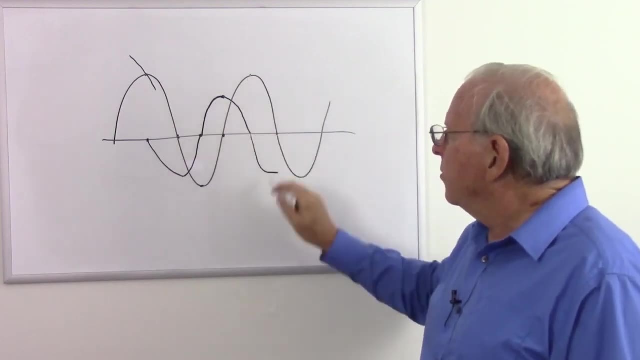 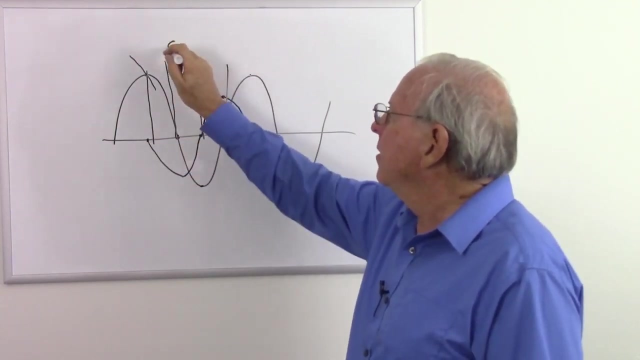 what are we going to get? We're going to get our maximum current- And this just keeps happening over and over again: Zero, maximum maximum zero. And so look where they are. Each time that happens is 90 degrees. So that's why we have that 90 degree phase difference in the voltage and current at the 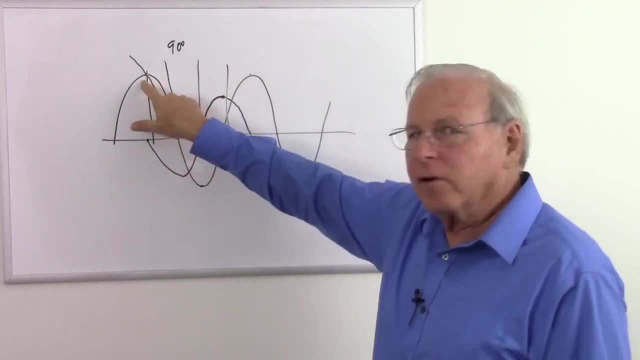 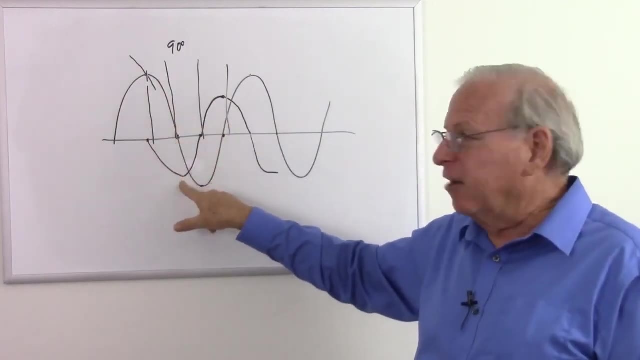 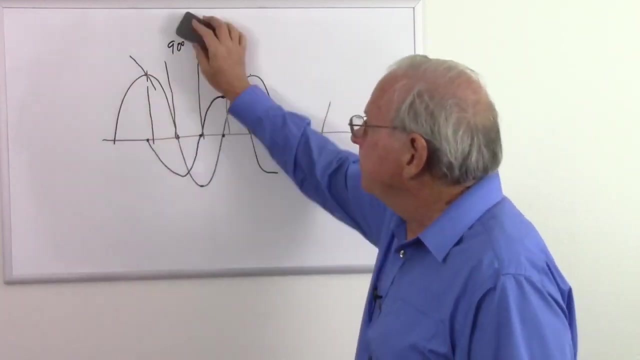 capacitor. because of this, Capacitor voltage is maximum, Current through the circuit must be zero. Capacitor voltage is zero, The current through the circuit must be maximum And therefore that's happening 90 degrees apart. So we're almost there. We almost know why we have the phase angle. 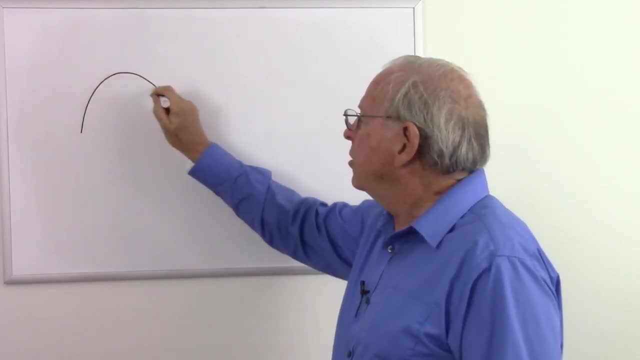 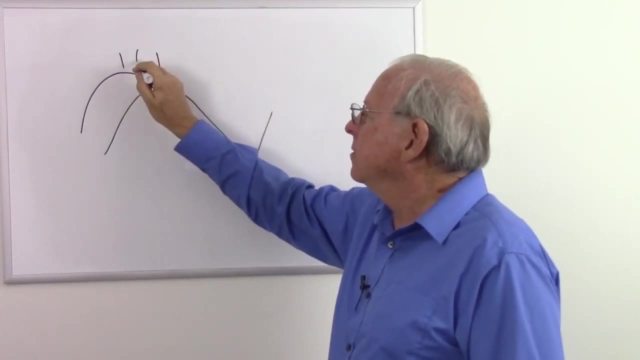 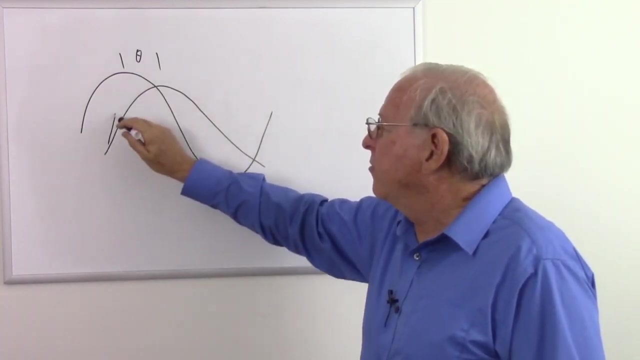 So we have the source voltage And then the capacitor voltage, And these happen some angle which we haven't determined yet, And that changes depending on the resistor and capacitor combination. So less resistance or less capacitance happens sooner. More resistance or more capacitance it happens later. So that's. 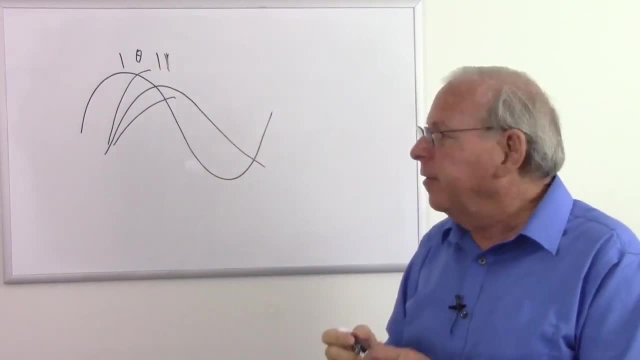 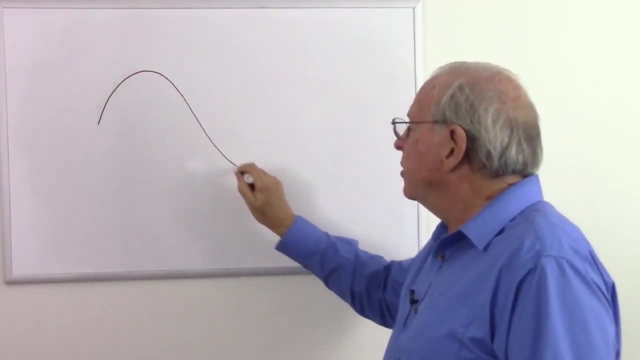 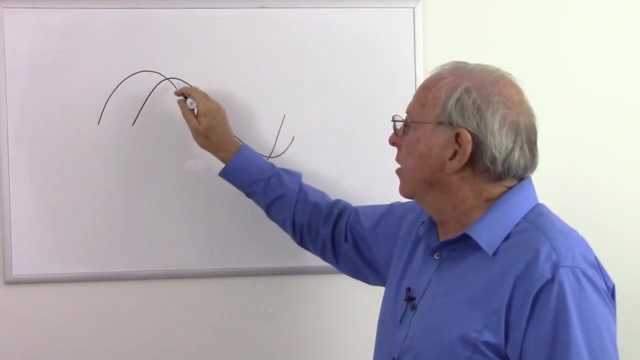 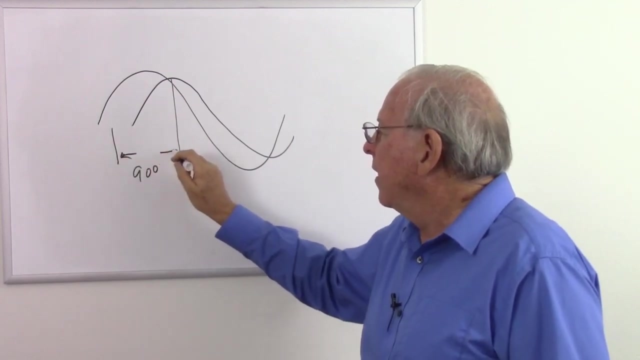 what determines this? And this ultimately determines the phase angle. But if I redraw this, we once again have our source voltage and then our capacitor voltage, But now we know that the current through the circuit is going to be 90 degrees before that capacitor voltage, And that is the final step that determines. 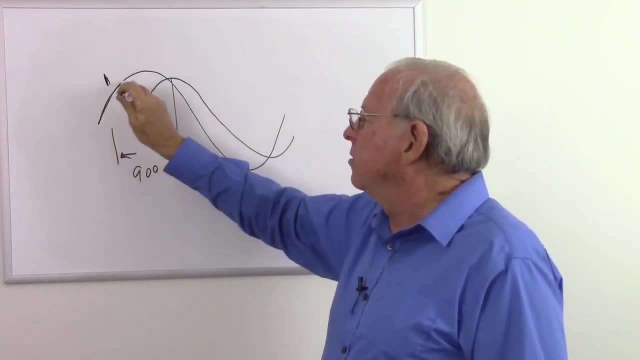 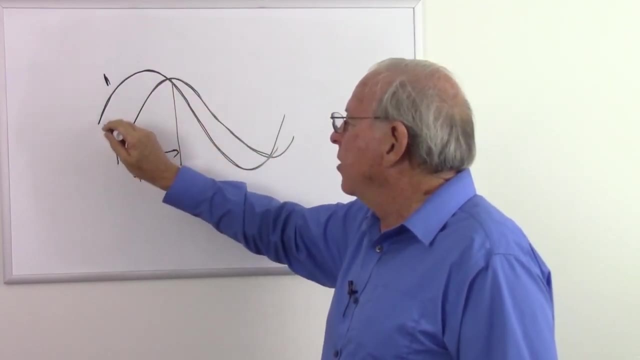 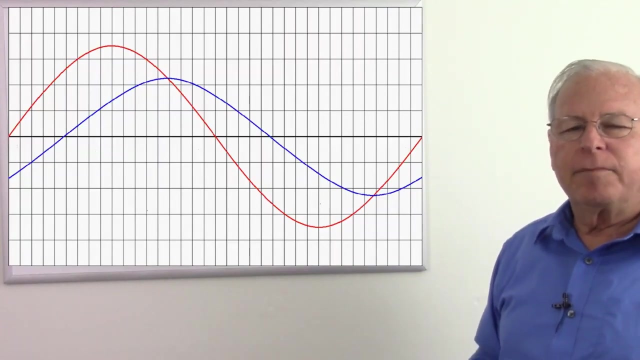 what the actual phase angle is. So here's our source voltage, Here's our capacitor voltage, And our current is going to be somewhere ahead of that. So if we look at our graph here, here we have the source voltage peaking. here the capacitor voltage peaks some. 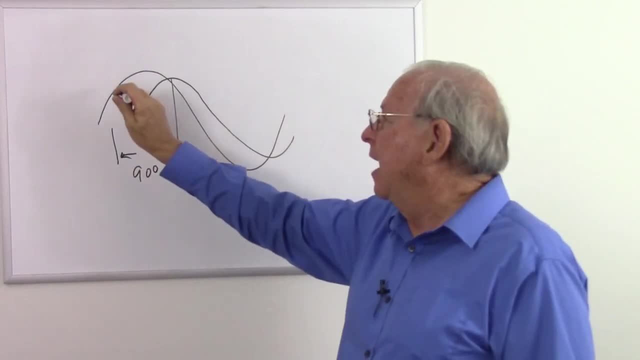 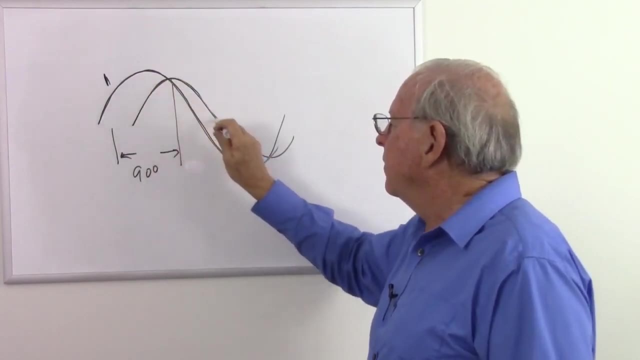 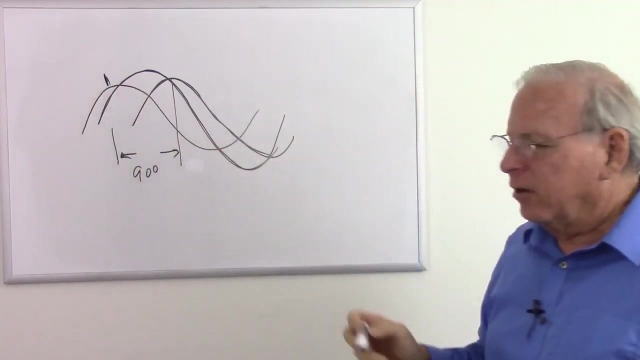 capacitor voltage, And that is the final step that determines what the actual phase angle is. So here's our source voltage, Here's our capacitor voltage And our current. Okay, And our current is going to be somewhere ahead of that. So if we look at our graph here, we have the source voltage peaking here. 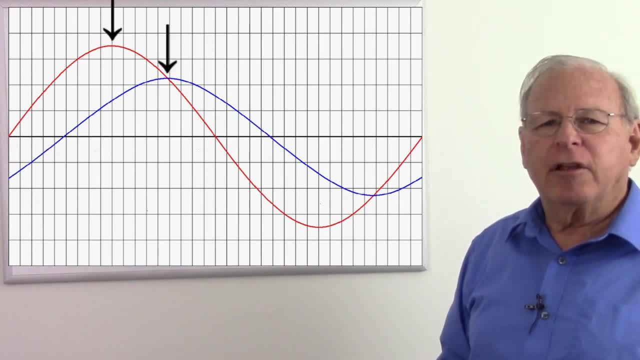 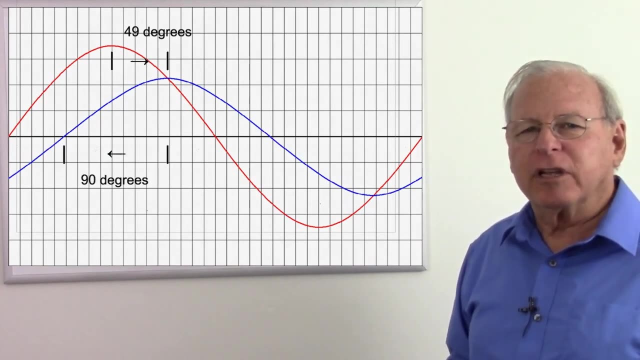 The capacitor voltage peaks sometime later, And that happens to be in this particular case. We have the capacitor voltage peaking 49 degrees after the source voltage, But then the circuit current is going to be 90 degrees before that, So we take the lag of our capacitor voltage behind the source voltage. 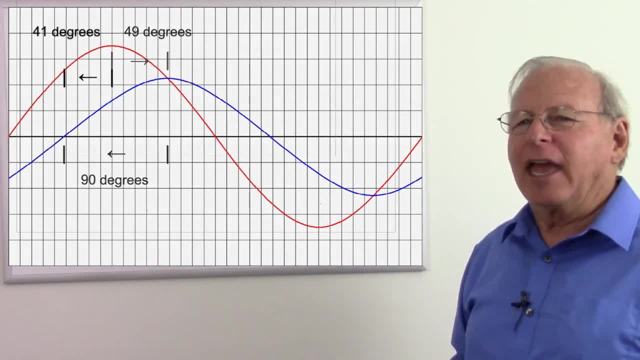 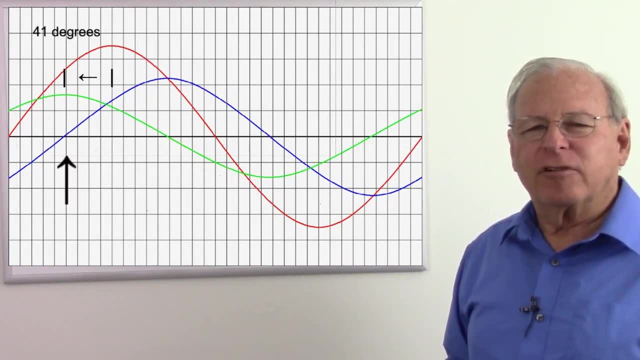 Subtract 90 degrees from that And we get the phase angle of our current. Notice that the current peaks when the capacitor voltage is zero And the current is zero when the capacitor voltage peaks. They're 90 degrees out of phase, just as they should be. 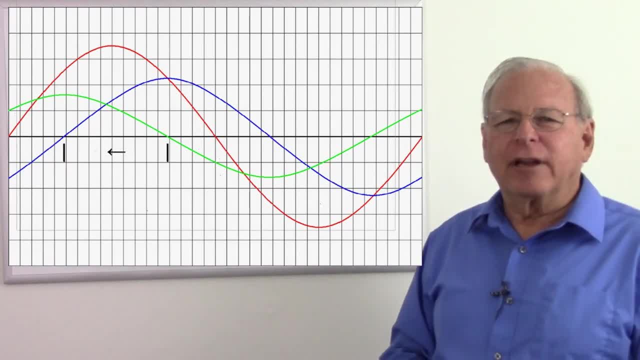 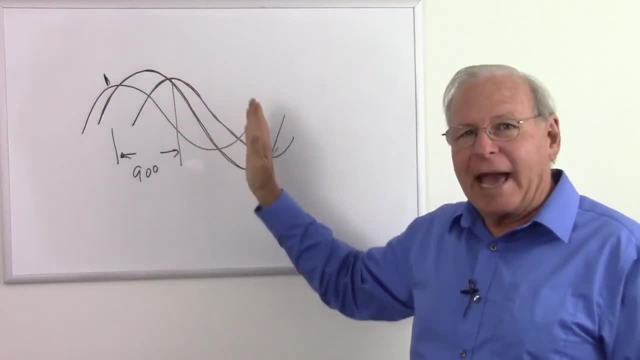 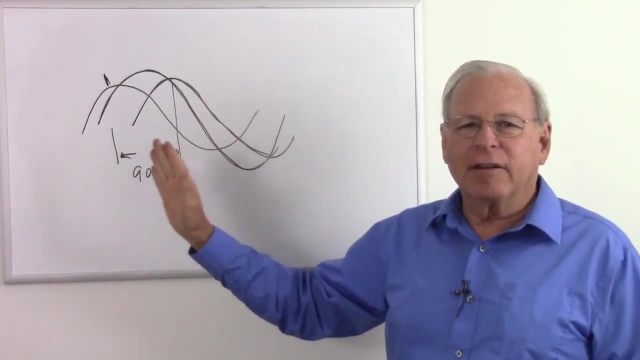 And that is why we get a phase angle in our circuit. Ultimately it's caused by the capacitor lagging behind the source voltage, But the actual angle of the current through the circuit has to do with the fact that it's 90 degrees ahead of the capacitor voltage. 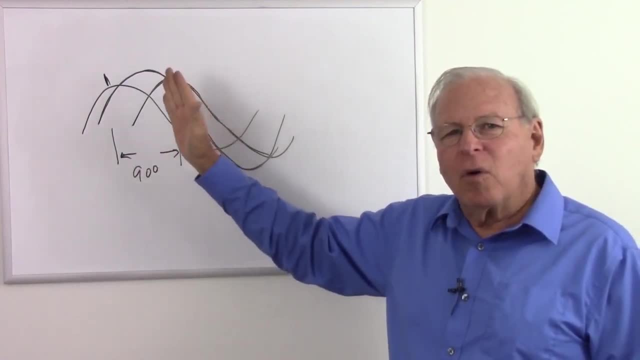 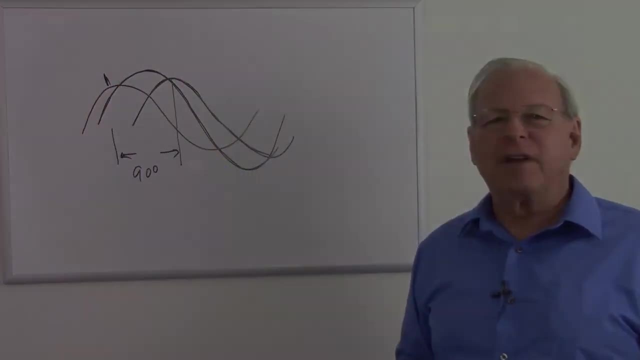 So the capacitor voltage ultimately determines what the phase angle is, But it's going to be the capacitor voltage minus 90 degrees And that's our final phase angle. If you found this video useful and informative, please give me a thumbs up down below. 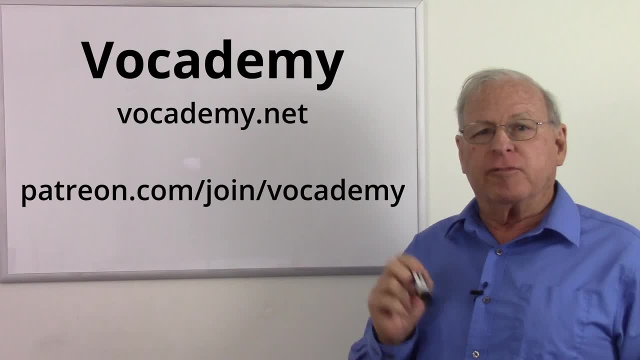 It really helps the channel And subscribe, because that not only informs you when I put new videos up, but it really helps the channel also. And a big thank you to my patrons at Patreon. I could not have done this without you. I could not make these videos without your support. 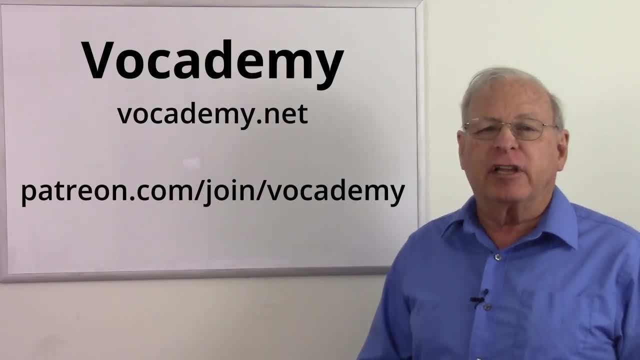 If you want to help me put these videos online and keep real vocational education free at vocademynet, you can go to patreoncom slash, join, slash vocademy and pledge your support. And again, a big thank you to my patrons who make this possible. And a big thank you to everyone for watching.